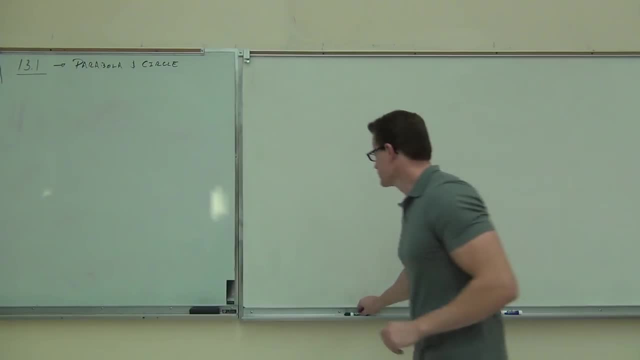 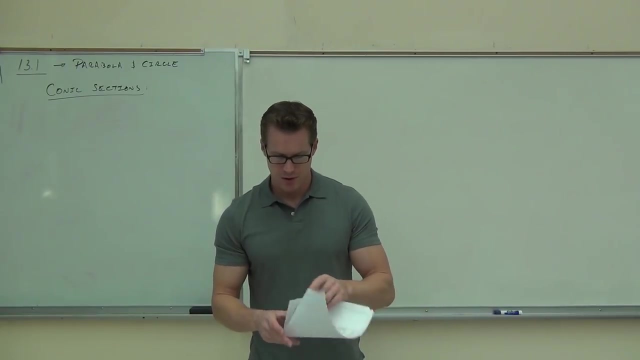 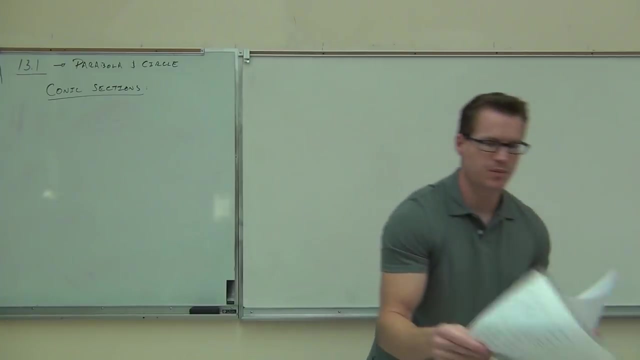 Conic sections. Here's what a conic section means. It means if I take a cone and start cutting it with a plane, these are the shapes I'm going to get. I want you to imagine this. Let's pretend for a second that I can make a perfect cone. I'm going to cut a cone out of this piece of paper. Cones look like that, basically. Now imagine that with this cone, I start cutting it. So here's my plane. 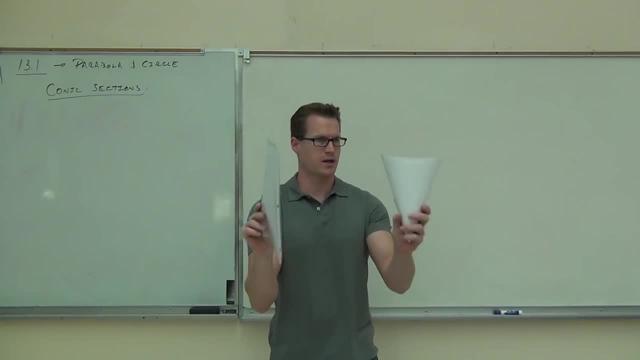 Imagine this is a perfectly flat plane and it's super sharp so I can cut through this. What would happen if I took this cone and I cut it straight across here and left it and looked at the shape that it made on my plane? 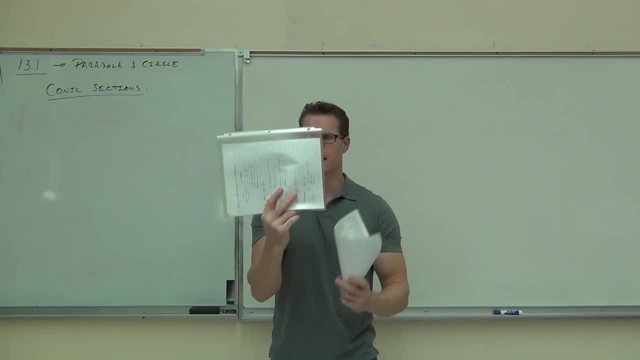 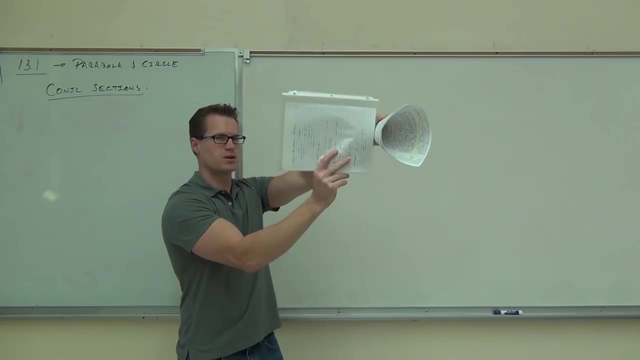 What would the shape be if I cut it straight across my cone and then looked at it? A circle. That would be a circle. If I cut my cone, look at that. Doesn't that look like a circle to you? If I cut that straight across and look at that shape, that's going to make a circle. Do you follow? 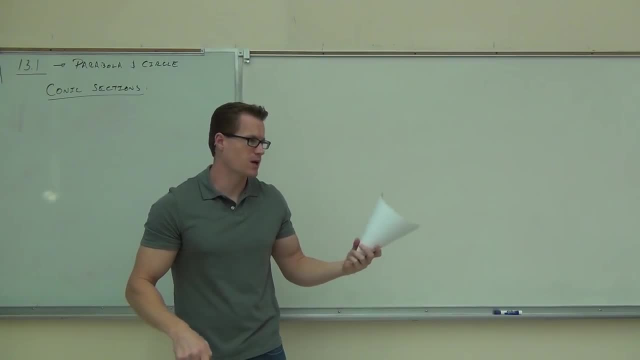 That's why it's a conic section. It means what we're going to have if we cut it. 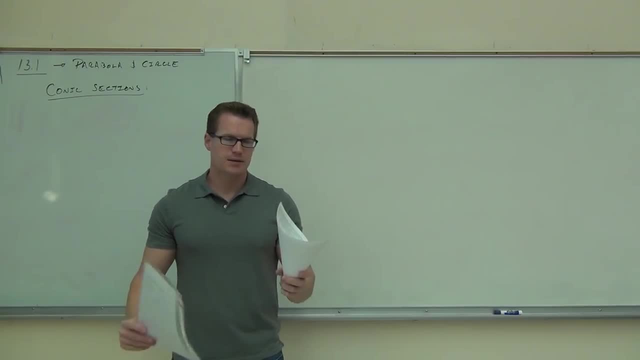 Now if I take and I cut it this way, straight up. If I cut it straight up, right through part of that cone, I'm going to get a couple of the shapes. I'm going to get a parabola. I'm also going to get a hyperbola if I cut it. I'm also going to get an ellipse if I cut it diagonally. If I cut it this way, I'm not going to quite get a circle. I'm going to get like an oblong circle and that's going to be called an ellipse. We're going to find those out later. 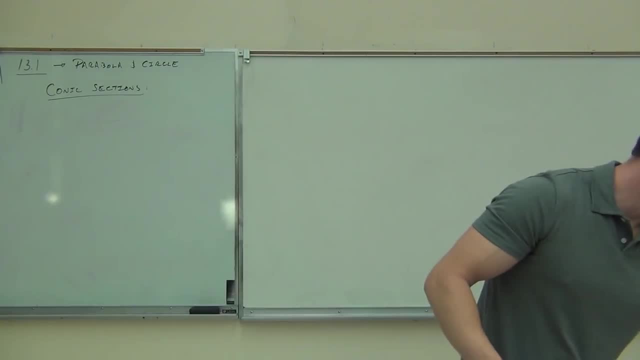 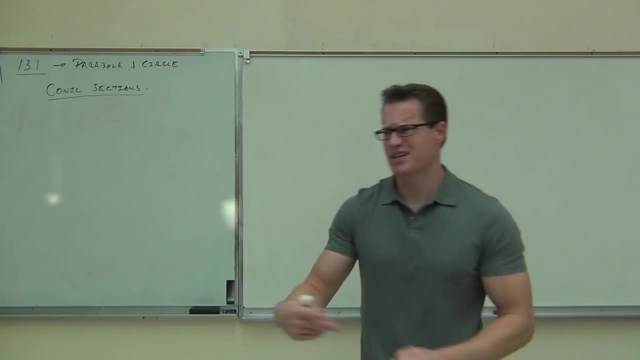 But for right now, we're going to talk about the first couple conic sections, circles and parabolas. Now we've already really talked about parabolas which is going to be kind of nice for us because it's just kind of a review. 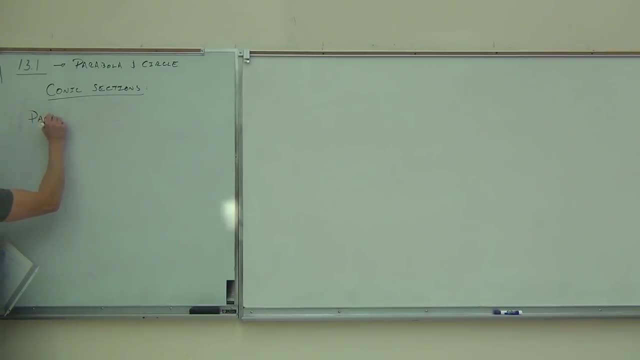 So with our parabolas, we have two types. 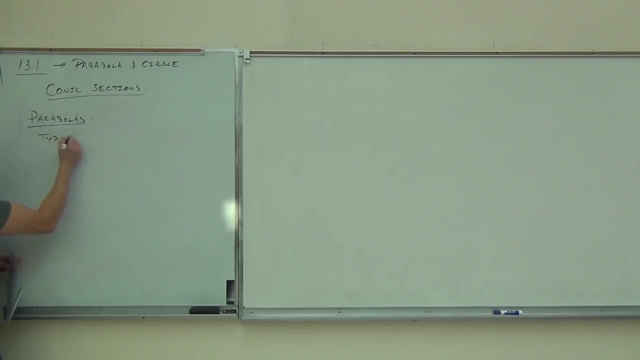 Type one is the one that we've been talking about this whole time. Do you guys remember that? I hope so. It was literally just on your test, right? I hope so. You should get your test back. 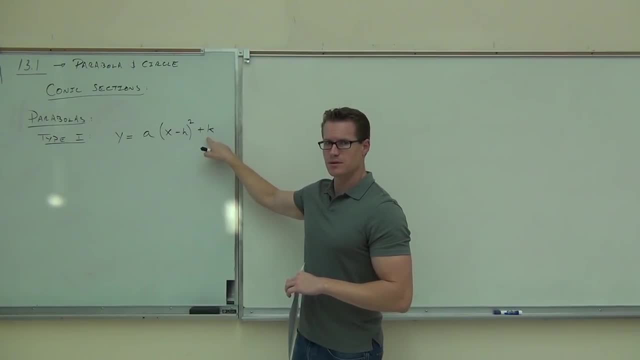 What's this do? Vertical shift. Vertical shift. Very good. 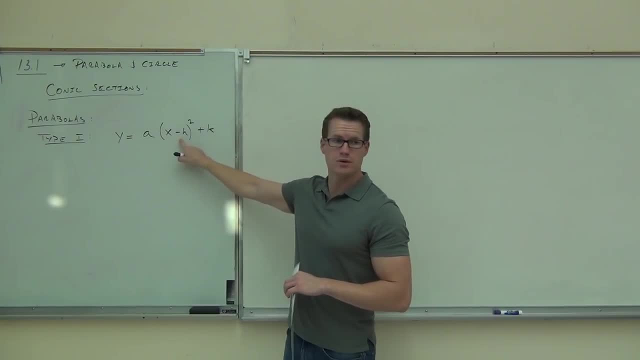 So this means up k or down k depending on whether it's plus or minus. What's this do? Right. This would be left or right. Minus means right. Plus means left. That says parabola. 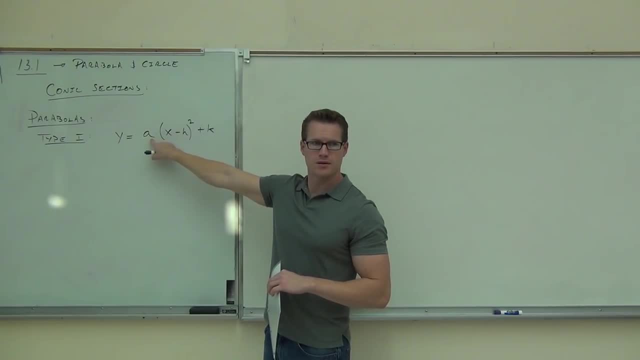 This says what? Whether it's reflected or not and whether it's wide or narrow. Good. Plus means upward. Minus means downward. Big numbers mean narrower. Small numbers, i.e. fractions means wider. Are you with me on that? 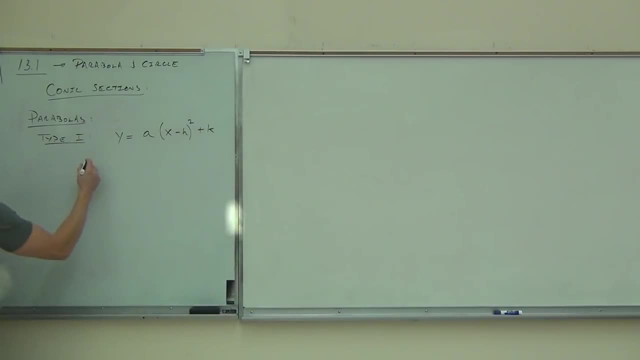 This is the parabolas we know and love. And as a matter of fact, if we try to graph it, we can actually find the vertex just by the shifting. If this gives us up and this gives us up and down, this gives us right and left, then if we put those two things together, then our vertex is actually at h k. 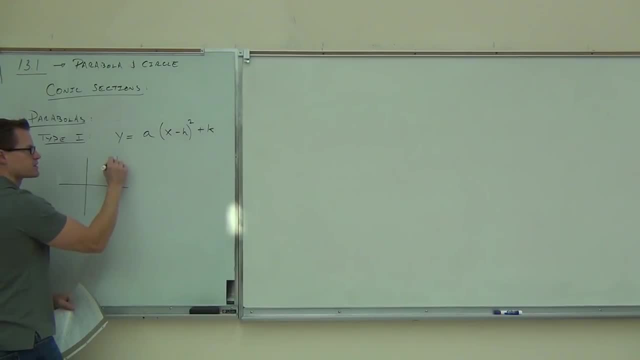 So whatever our numbers here give us gives us our vertex. Now, of course, if there was a negative up here, we would be reflected downwards. 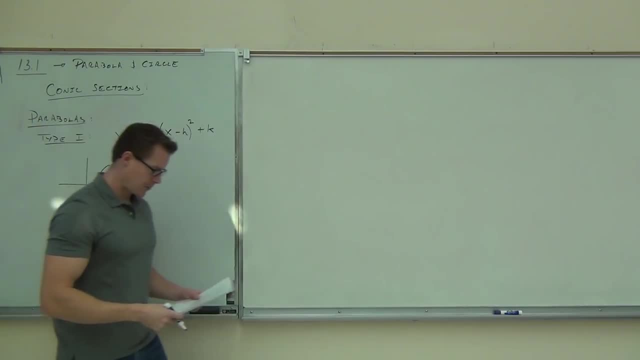 If there's not, well, then we're upwards. So we can have this one. We could also have an upward facing. I'll give you one of those, too. Now, of course, I can't be precise because I don't know what h and k are. I'm just giving you the in general. 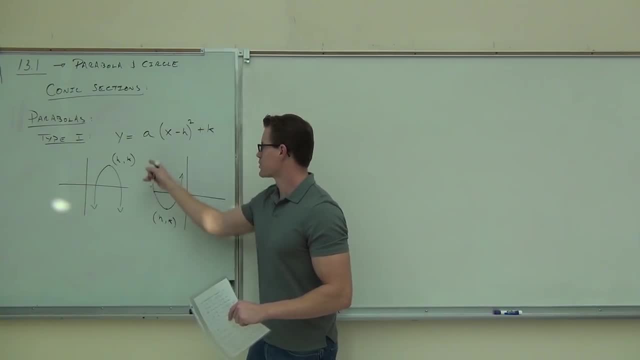 We had these two ideas. We had normally our parabola would go upwards if a was positive, if a narrow, if a was large, or wide if a was small, fractions. We also can locate shifting, and that means we move our vertex to where those shiftings occur, up or down according to k, left or right according to h. 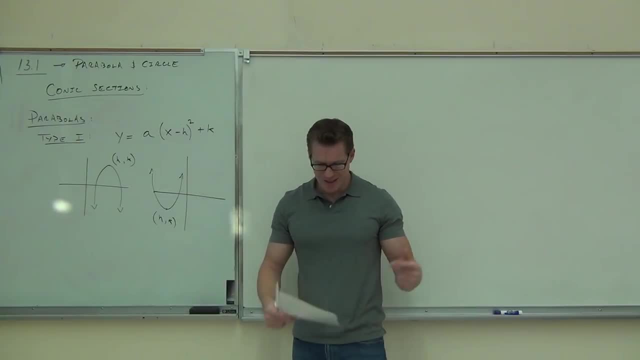 Are you guys okay with these pictures? Now, I'm not going to give you any examples because we've done so many of those. This is old stuff. 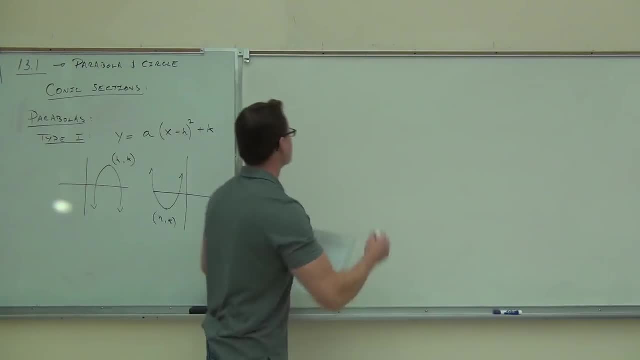 What we haven't talked about is type II parabolas. Type II parabolas say this. 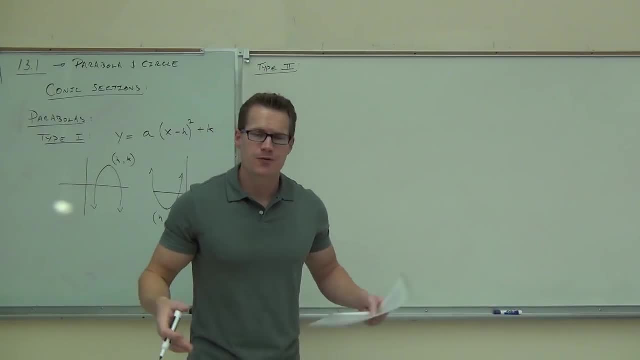 Let's ignore for a second the whole function idea. Functions mean they pass the vertical line test. 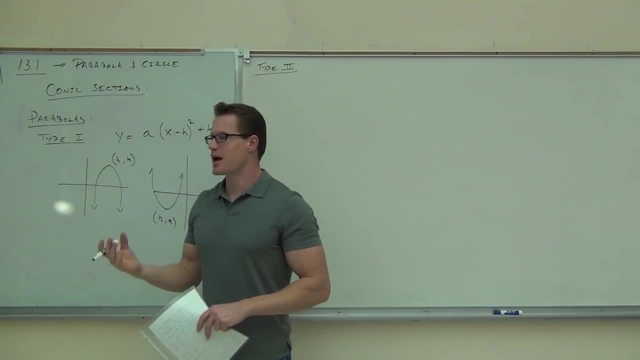 So let's ignore that for a second. Can we define a parabola not with an independent variable of x 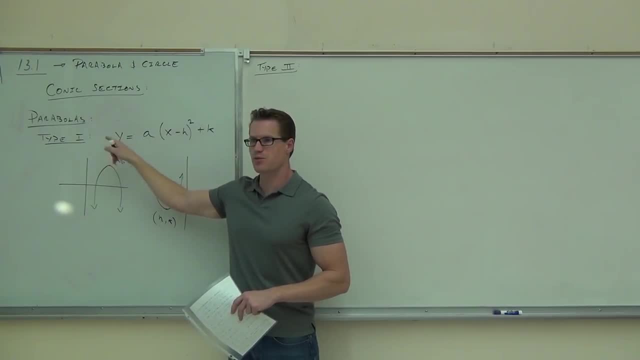 but with an independent variable of y? That means instead of y equals something in terms of x, we're going to have x equals something in terms of y. What this will do, this will flip our parabola not straight up and down but left and right this way. Does that make sense to you? 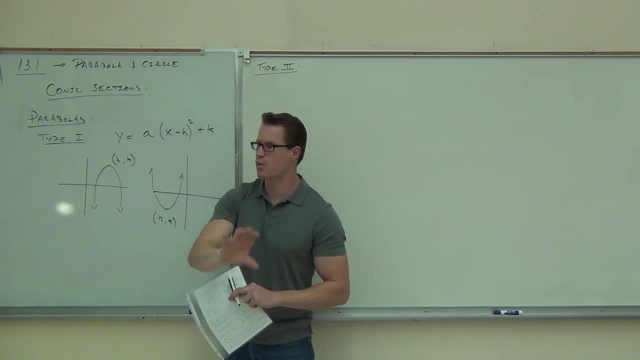 So we're going to have now a parabola based on y, not x. That's a type II parabola. Is it going to be very similar? Yeah, absolutely. 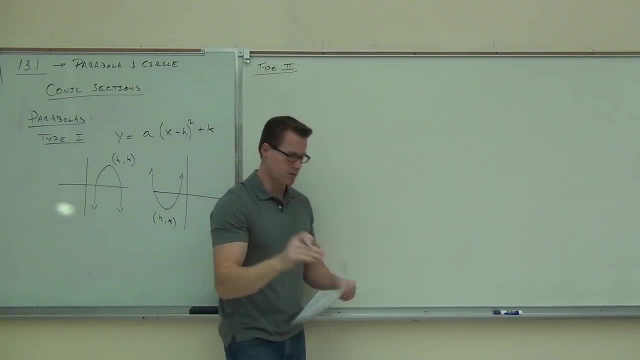 It's only going to be facing this way or this way instead of up or down. 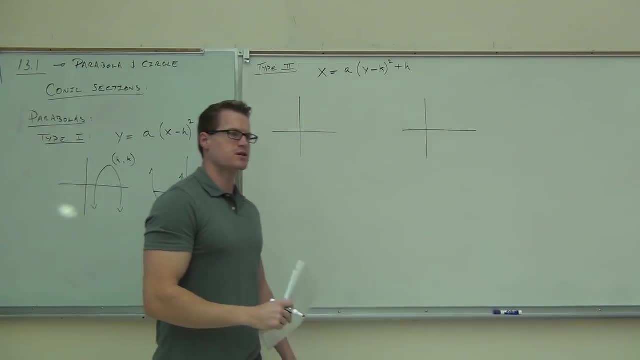 Now you're going to notice a couple things about this. First thing we notice about this is that, well, our y's and our x's are changed. That means that our independent variable is no longer x. It's no longer going to be based on the x axis. It's based on the numbers you plug in for y. What that's going to do for us also is change around our vertex. 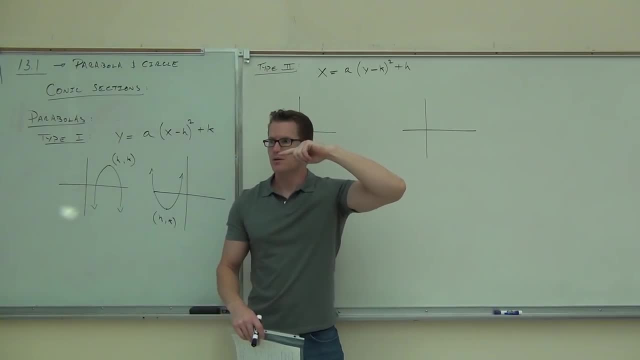 So whereas this number here used to be a shift up or down, now it's a shift left or right and that makes sense to you. If this is a shift right or left, this one's going to be a shift up or down because we switched our variables. So this one now is a right and left and this one now is an up or down. So we're switching our variables. 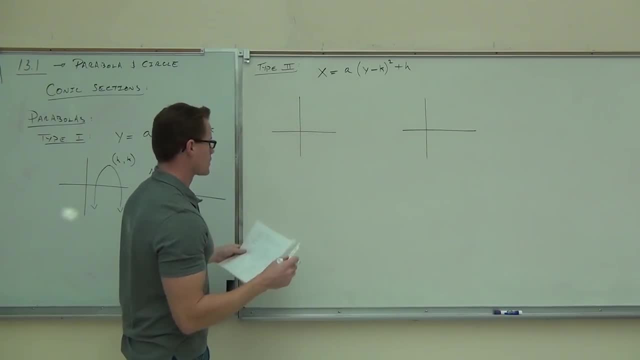 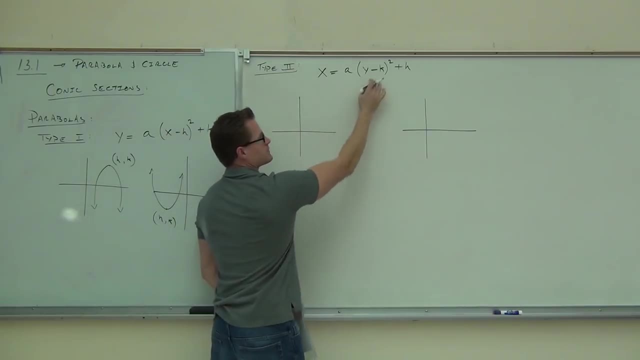 That means we're switching our axes basically. So in our case here, our vertex is still going to be h, k, but look where h and k is coming from. h gives us our right, left. k gives us our up, down. 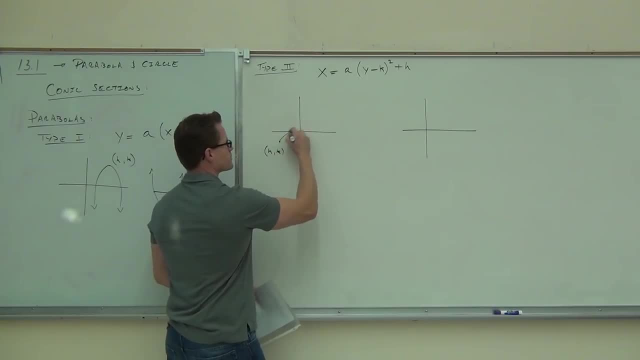 Now a positive means that we're going to be facing this way. So if a is positive, we're opening this way. If a is negative, we'd be opening the other way. The whole skinny white idea still works. 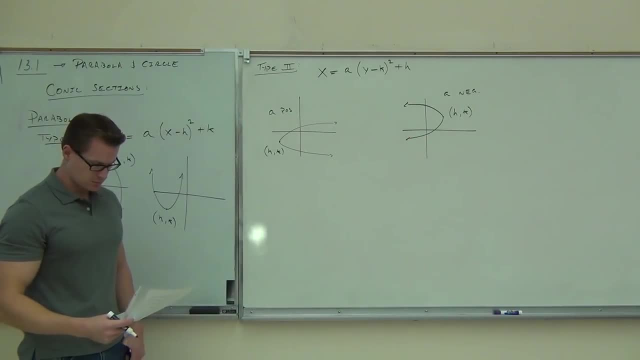 That still works. Same thing. Same thing. Would you like to try an example? Sure. OK. I figured you kind of might. 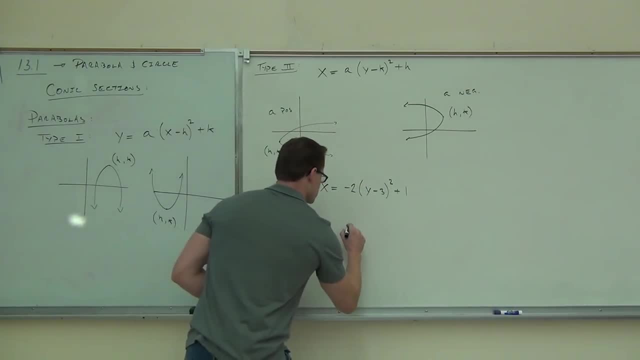 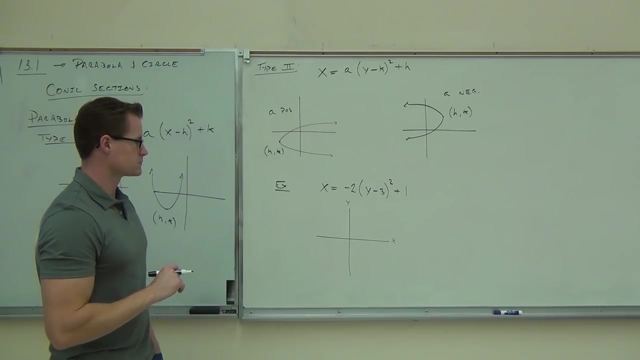 OK, are you ready for it? You've got to switch some ideas in your head right now. 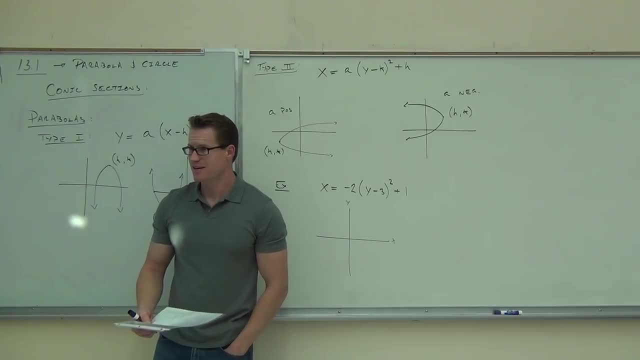 OK. some ideas in your head now, okay? Get a switch some ideas in your head. 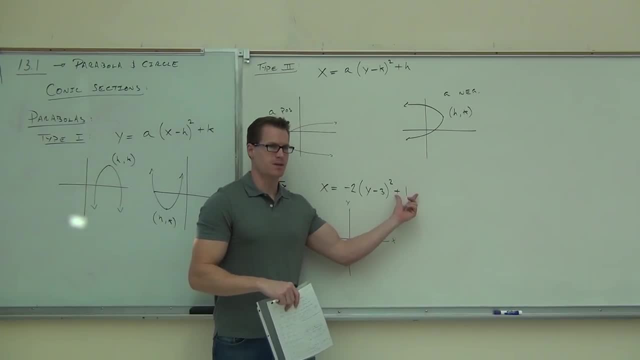 Do you remember how this number would typically be up one? You with me? 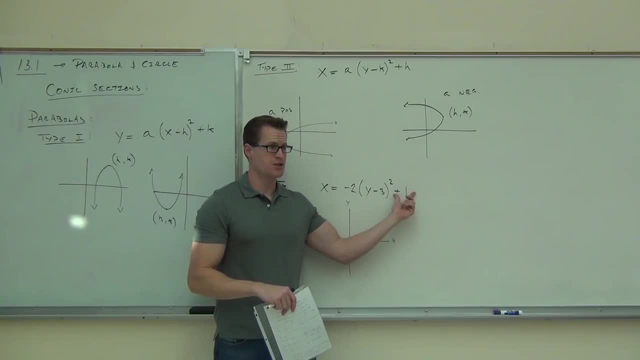 Now this is not up one, we've switched our axes, this is now right one. Does that make sense to you? This is right one. 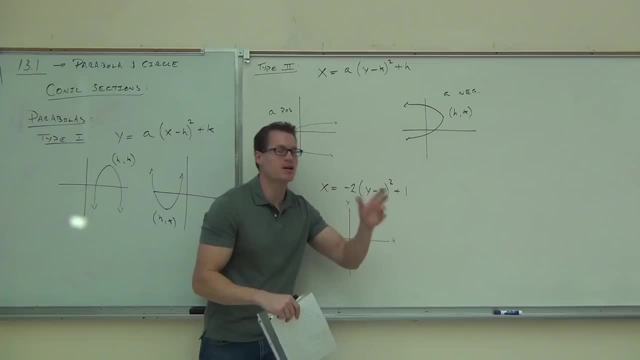 The whole plus is right thing makes sense now because again, we're switching our axes. So whereas this would normally be an up, this is now a right. You follow me on this one? So this is gonna be right one. Now, what would this normally be? What would this normally be? Right three. 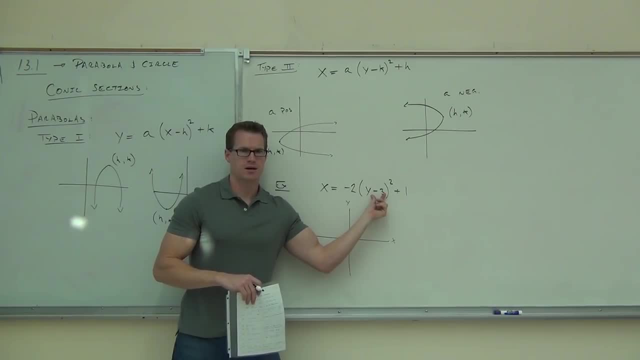 This would be a right three. This is gonna be a up, an up three. Does that make sense? Are you sure? 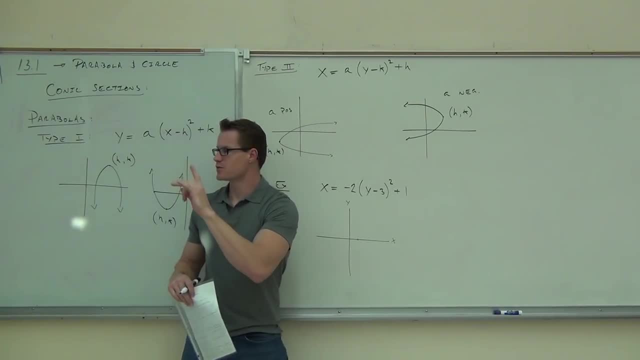 So why up? Because you're switching left and right up. 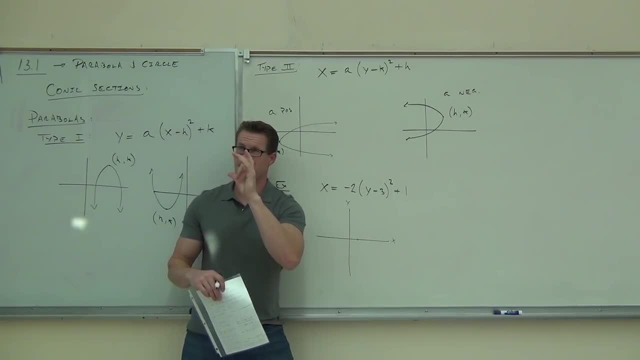 You're switching right, you're switching left and down and you're switching up and right. 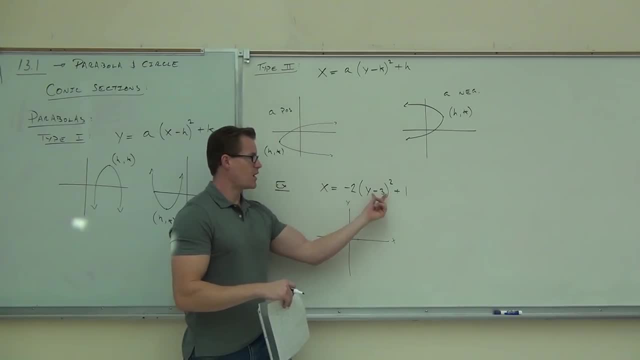 Oh, that's hard to remember. But you're switching those ideas. So now this is your right and left and it's like your brain wants to say it. Plus means right, minus means left. This is your up and down now, but minus means up and plus means down. So you've switched those concepts. How many of you feel okay with this? It's a little weird, right? It's a little strange. 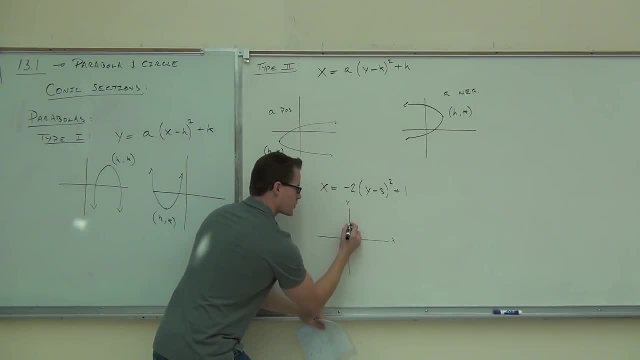 So our vertex here is gonna be at one comma three. 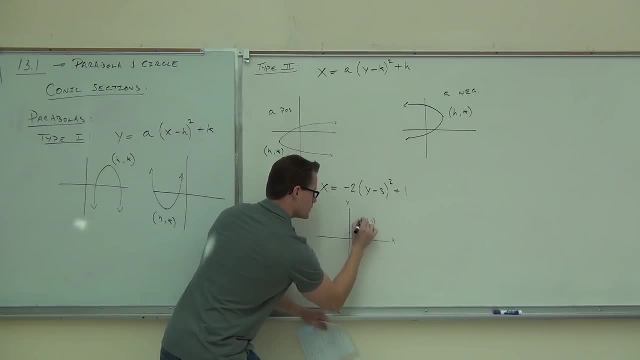 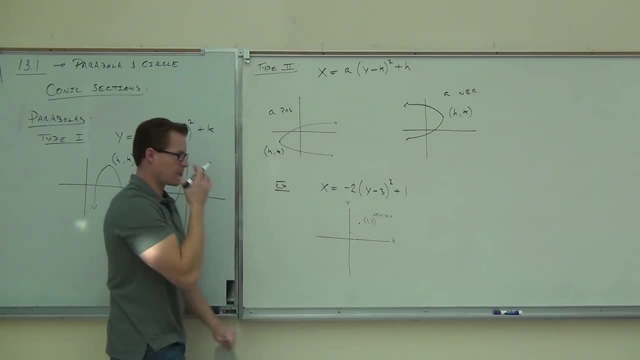 Hey, question. Can you determine which way my parabola should be opening? Is it gonna be open up or down, do you think? That would be... 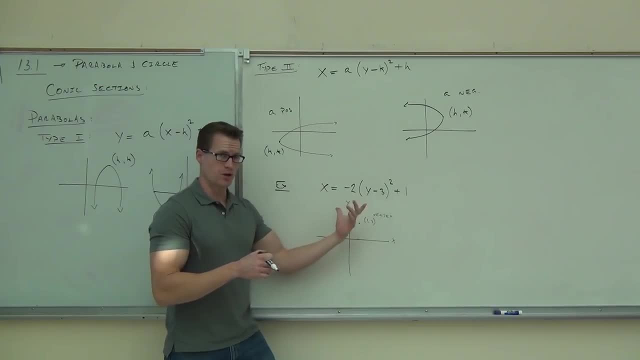 If that was gonna be open... if that was a y, if y equaled something to x, sure, it'd be up or down. 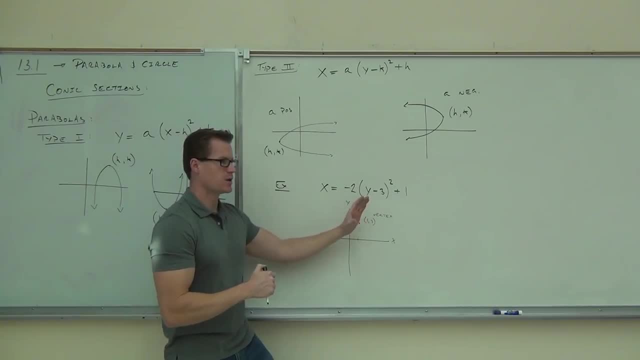 We would have exactly this. But now we're either going to be opening to the right or opening to the left. Now, if typically up 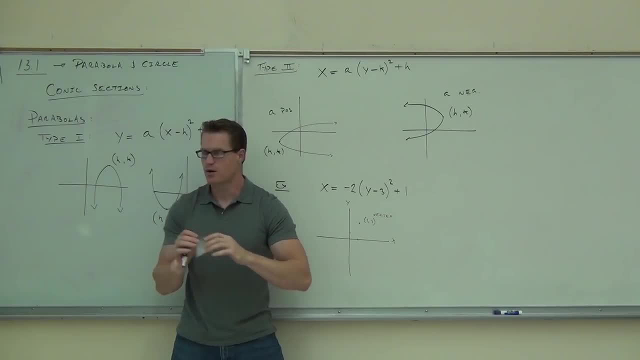 means right and down means left now, which are we? Are we to the right or are we to the left? Which do you think? 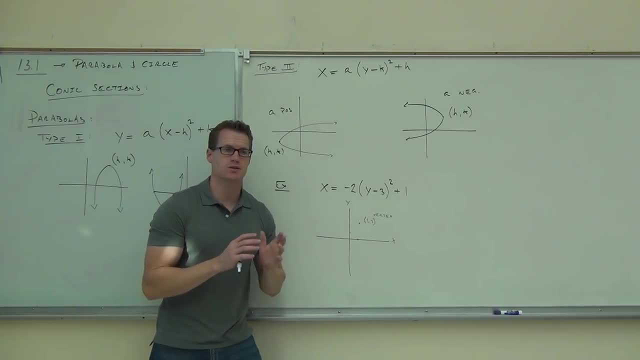 We're to the left. Exactly right. Now there's one thing that we can still do. This is kind of nice with this type of parabola. Watch carefully over here. 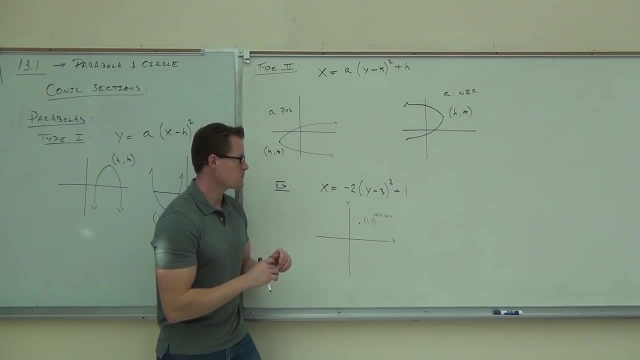 What we can do we can look at this thing and also determine our well, you know what, I don't want to do that too. Just sketch your parabolas for now. 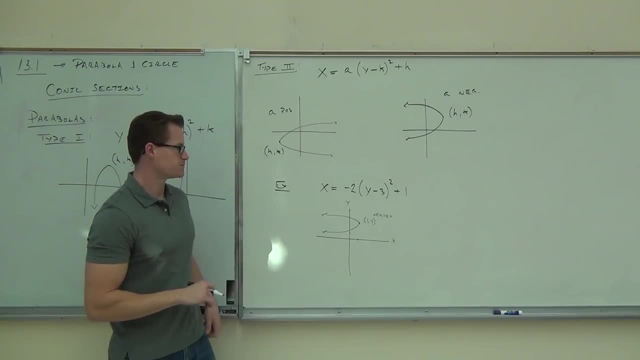 It's going to be a little bit more narrow because we have that whole number again. Now is it a function? No. But is it a different type of parabola? Yeah, it's a type 2 parabola. We can make it on its side now. 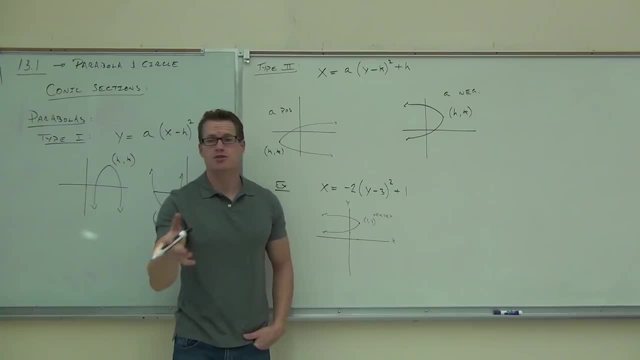 How many of you will feel okay with this? This idea. Let me have you try one of your own real quick. There you go. 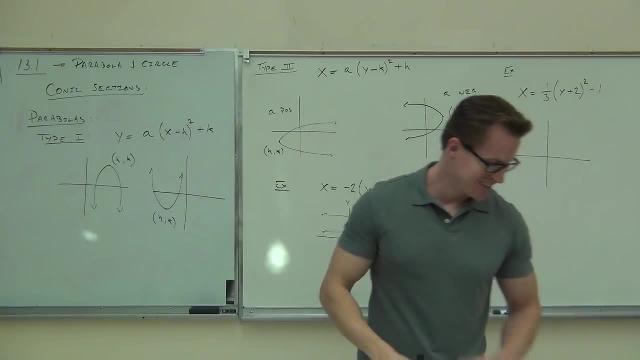 It's hard to even write those for me. We've been doing another one so long. Is that my third time? Yeah. 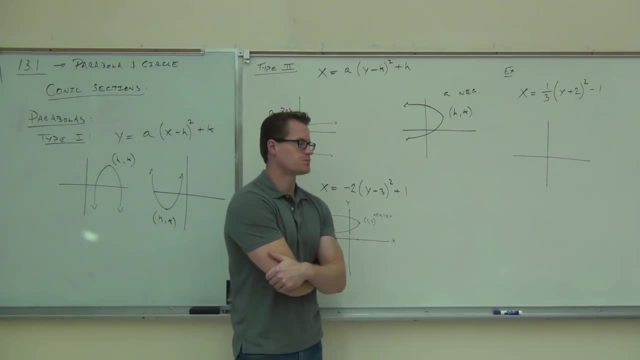 Is it possible to have two axes? No. Oh. I don't know what that is. 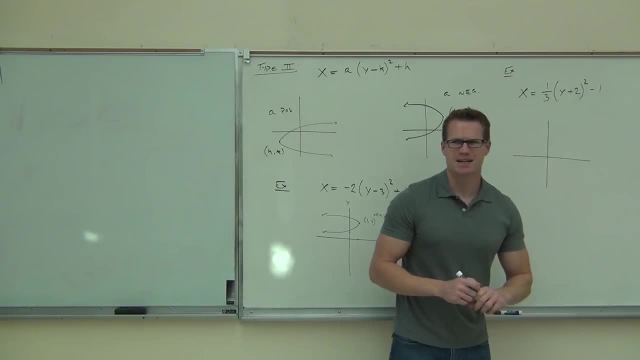 Let's see if we got it. Firstly, are we a type 1 or a type 2 parabola here? Type 2. Type 2 because we have x equals something in terms of y that makes it a type 2. That means it's going to be on our side somehow. 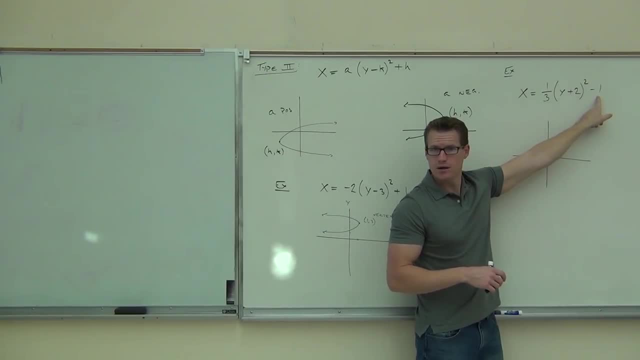 Firstly, what does this do? Is this a down 1? Left 1. A left 1. This is a left 1. Did you find left 1? 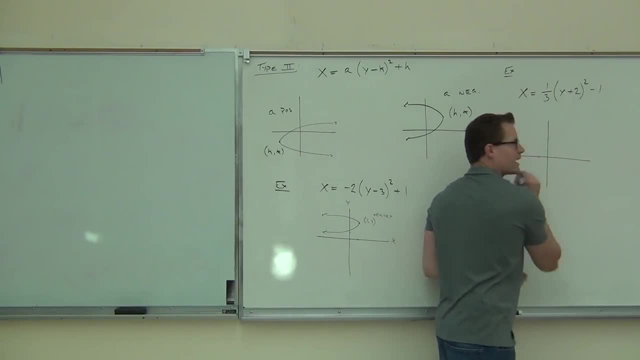 Yeah. Good. Okay. You'll get the hang of it. 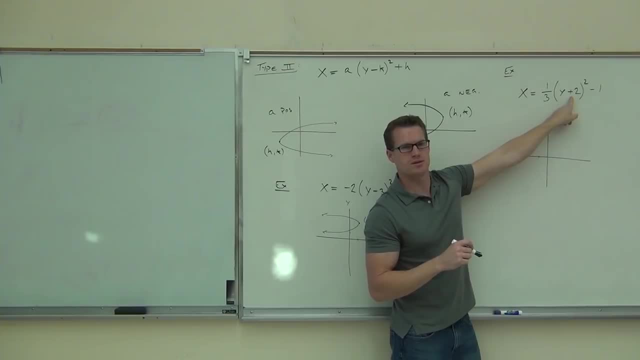 Now what does this 1 do? This plus 2? Down 2. Ah, yeah. It's in parentheses. It's opposite what you think. Now it's down 2 spots. 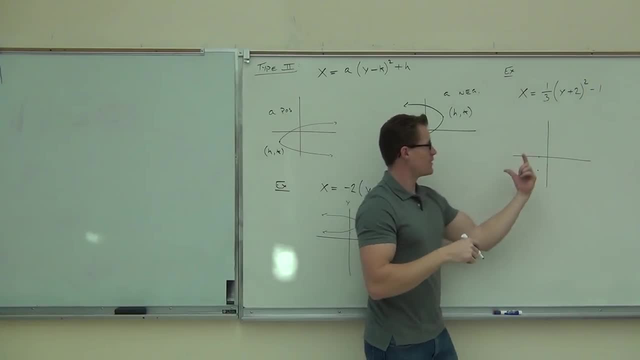 So that's where we put our vertex. Are we going to be leftward opening or rightward opening? Rightward opening. Rightward opening. And is it going to be wide or narrow? Wide. 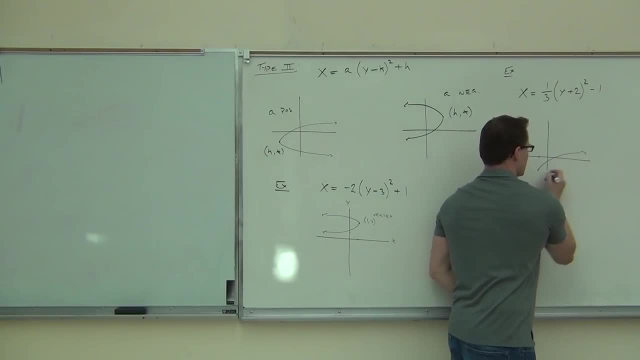 A little wider. So we're going to make a nice sketch of a parabola. There you go. 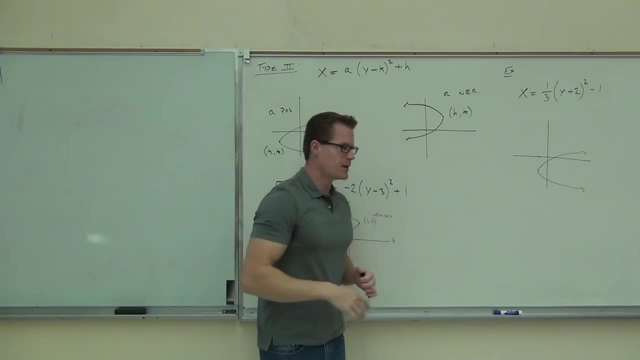 How many people feel okay with our idea here? Good. Alright. Now I need you to know that we can do the very same thing. 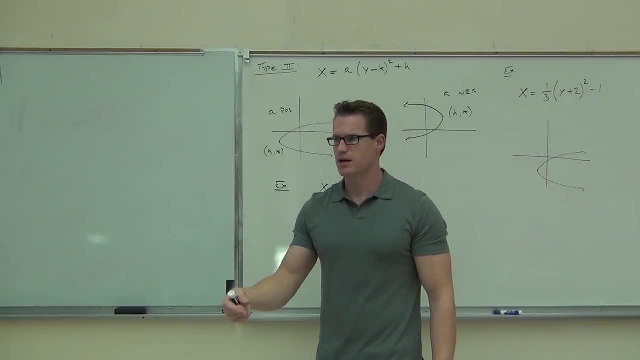 If I had you find, remember finding the vertex? Finding the vertex and the y-intercept and that on your test. 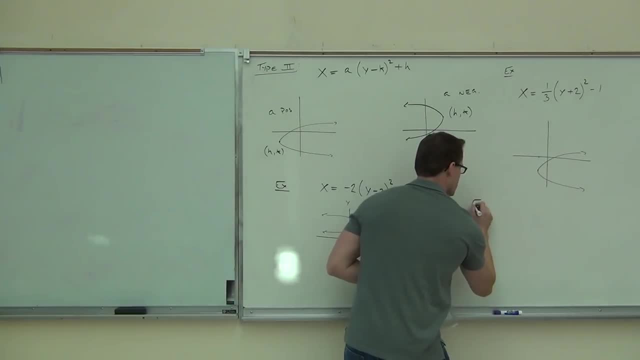 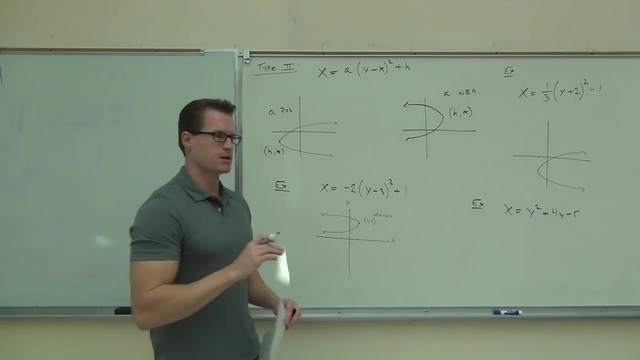 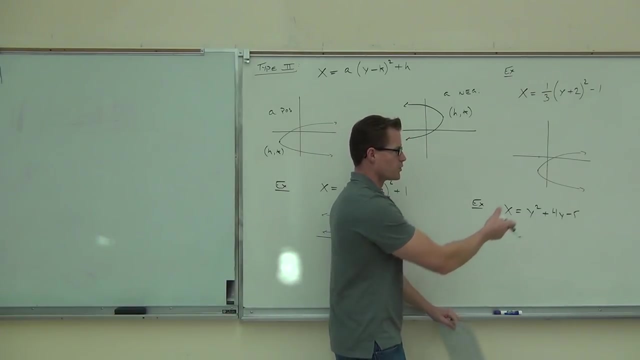 You can also do that with a type 2 parabola. So for instance, if I give you this one, x equals y squared plus 4y minus 5. You can still find the vertex. Now it would be x-intercept. And the y-intercept. And the y-intercepts. So x-intercept here would be our negative 5. 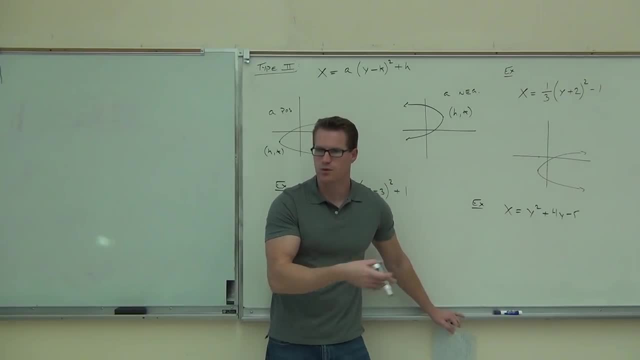 Remember we're now on the different idea where we're going sideways now. So the x-intercept would be negative 5. 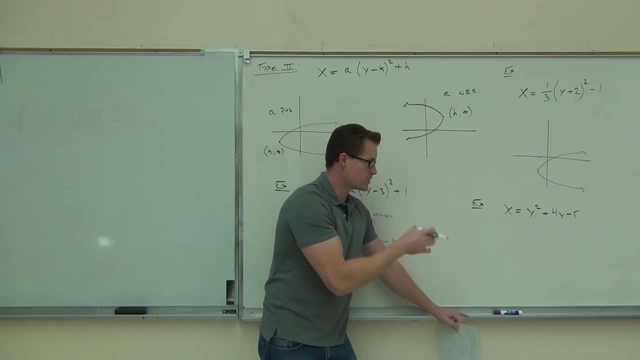 The y-intercepts would be when you said that equals 0 and you factor and solve. You with me on that? 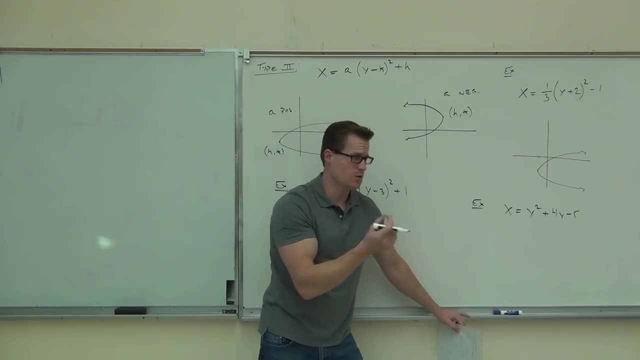 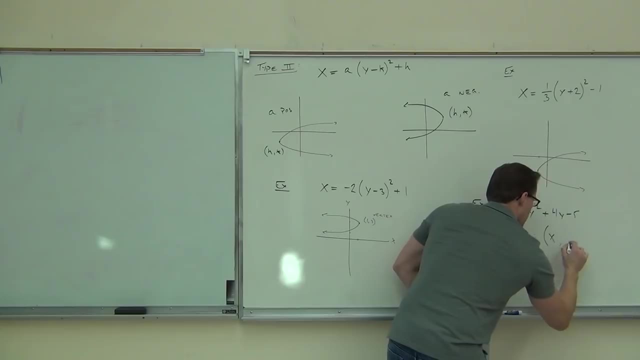 The vertex is the only one that's a little bit different. Remember we're searching variables here. So our vertex would be given by x. Common negative b over 2a. You find this one and plug it into here. So I'll make that like I did earlier. 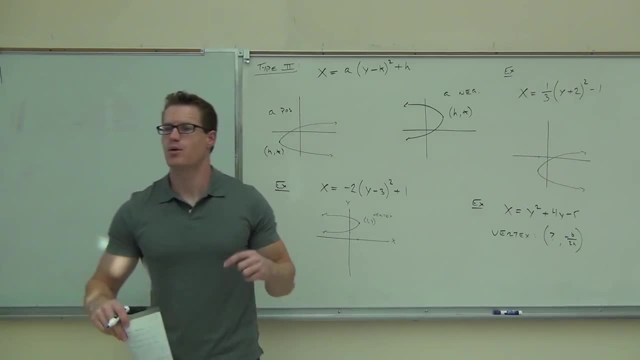 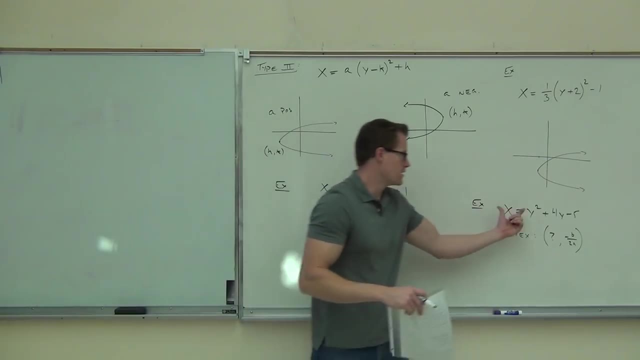 Question mark. You have to find it in terms of y first because now y is your independent variable. Does that make sense why we switched those things? Because now you don't have any x coefficients to work with. You only have y coefficients. So that's the only one that's different. Your x-intercept would still be that number. Your y-intercepts would be set to equal to 0 and factor and solve it. 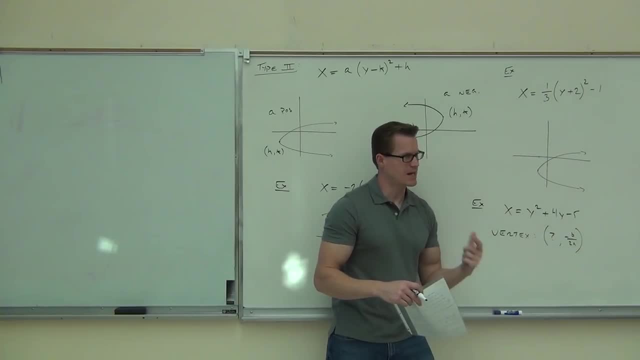 Your vertex is just reversed. Same exact idea. 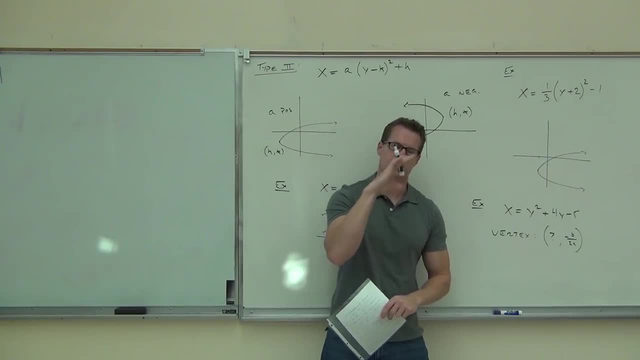 Try one of those out when you get home. Just think about it as if it's on its side. Does that make sense to you? 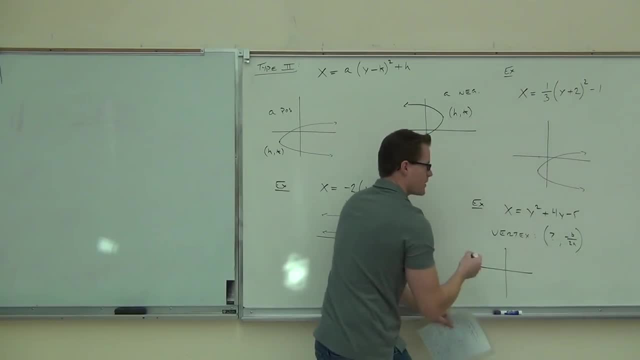 So in our case we could... What I mean by this is x-intercept is negative 5. 1, 2, 3, 4, 5. That's right there. 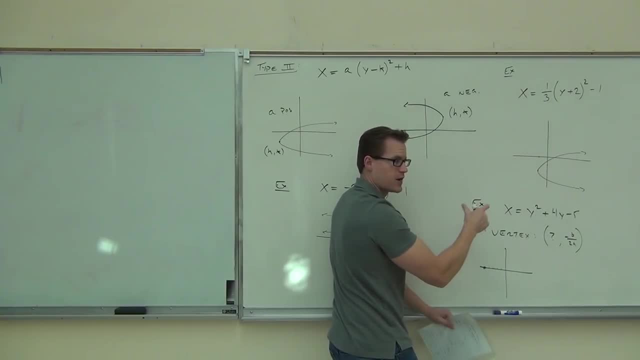 Your y-intercepts, if you factor that, you're going to get x plus 5 and x minus 1. 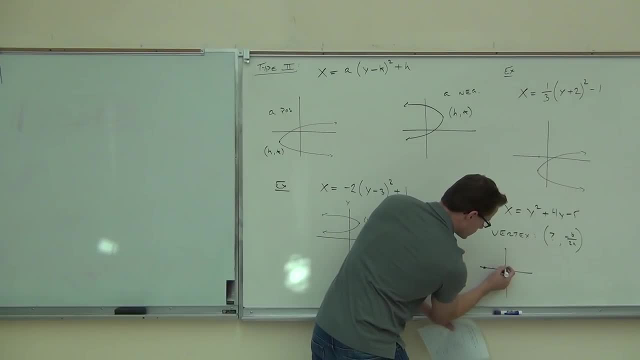 That means we get 1. Did I do that right? 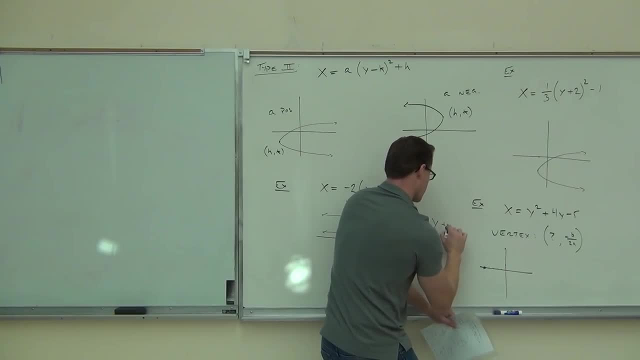 Let's see. There we go. y equals negative 5 and y equals 1. So we have y equals 1 right here. 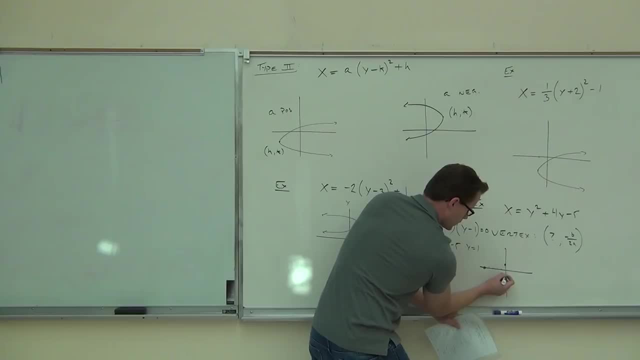 It's weird, right, because y is positive up this way. 1, 2, 3, 4, 5. And then you'd find your vertex. Your vertex should be somewhere around there. 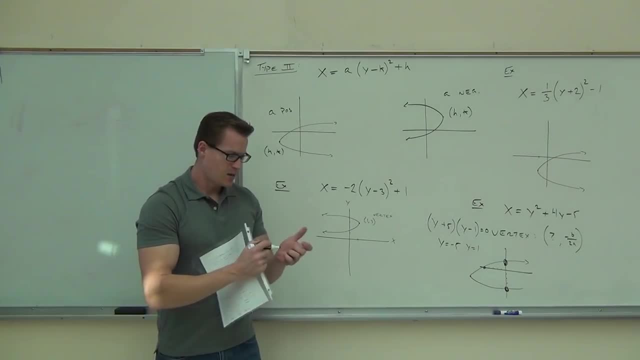 Let's make those bigger. There we go. But that's the basic idea. So try that out on your own. 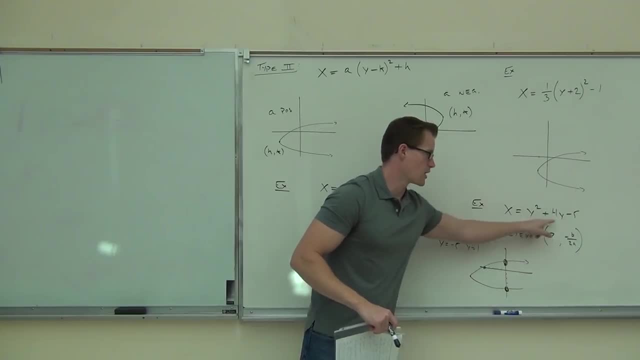 The only one I didn't do is the vertex, but I think you guys can handle that. Can you find out your a here? 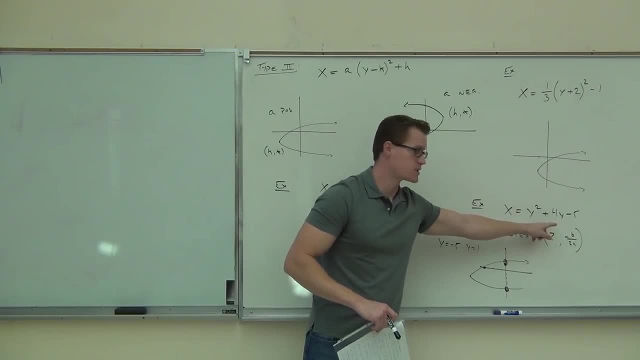 What's your a? What's your b? What's your c? So plug in negative b over 2a. 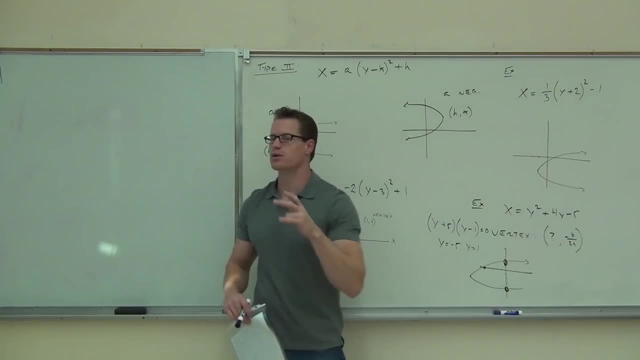 Then we plug that into the function to find x instead of finding y. That will give you your vertex in this case. 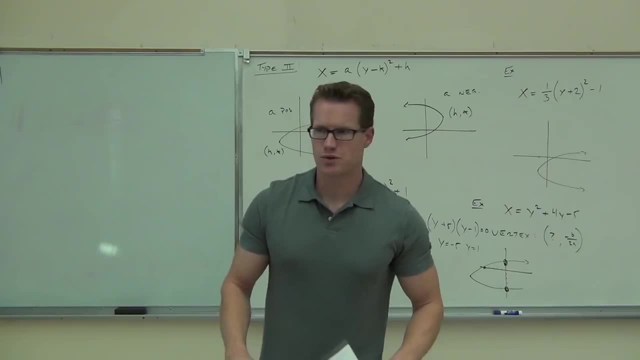 Now the other concept we have to look at is circles. We're going to do an introduction to circles right now. 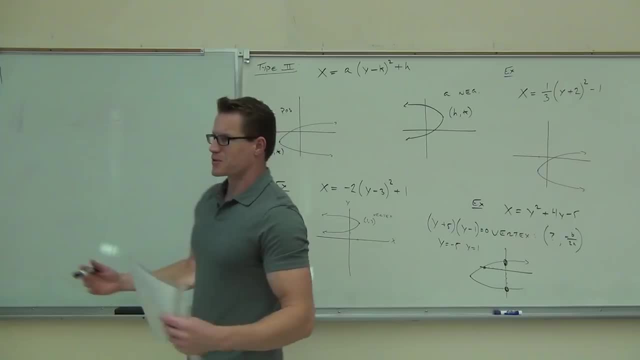 I'll give you more specifics next time. What is a circle? It's round. Round. What's round mean? Circle. Oh, good. That's not circular reasoning at all. 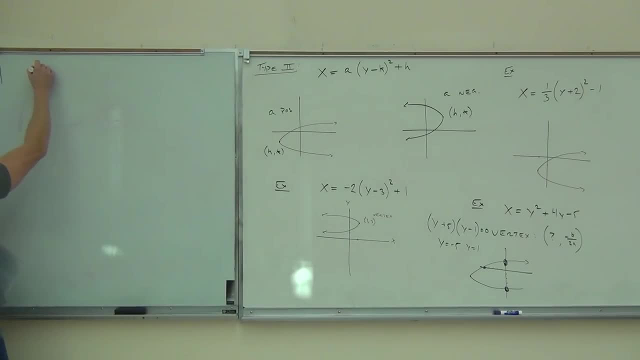 It touches. It touches all the time. It touches all the time. Very good. Very good. This touches all the time. Is that a circle? No. If you're really blind, it is. Very good. What's a circle? What's a circle? 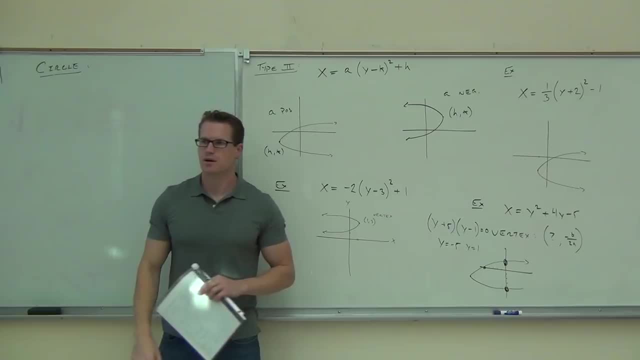 How would you, if you had to make a circle, if you had to make a perfect circle, because when I draw a circle, I know we all know what a circle is. A circle is this. That's actually not even a circle. If you had to draw a circle like that, it's probably not going to work out that well, right? Unless you're really talented. It's still not going to be a perfect circle. 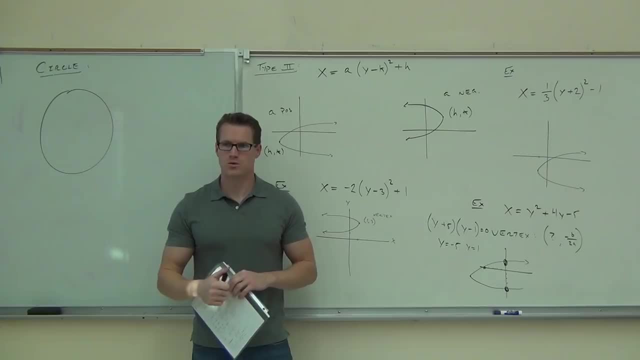 How would you draw a perfect circle? As a radius? Well, of course circles have radius, but how would you do it? If I said draw a circle, what would you need to draw a circle? Oh, that thing. Compass? Well, you could use a compass, but if those weren't invented. Trace something that's around it. A compass. A stick. Maybe that's it. Tell us the answer. 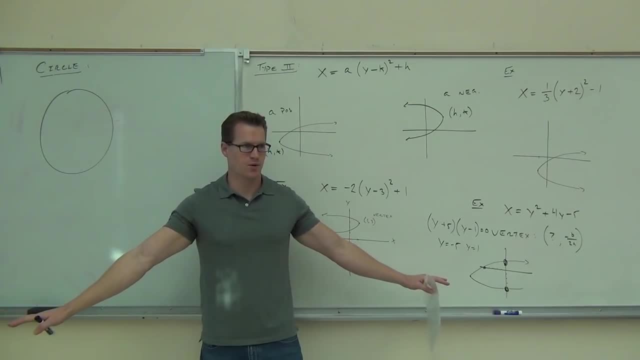 Sure. Let's say here's sand. You have a sand floor. Okay? You have a sand floor. You have a stick. What else do you need? Nothing. Say what? 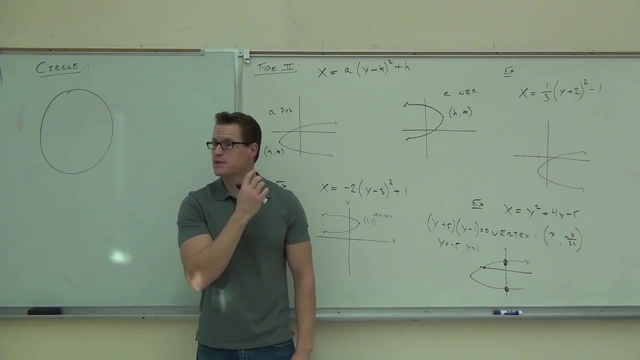 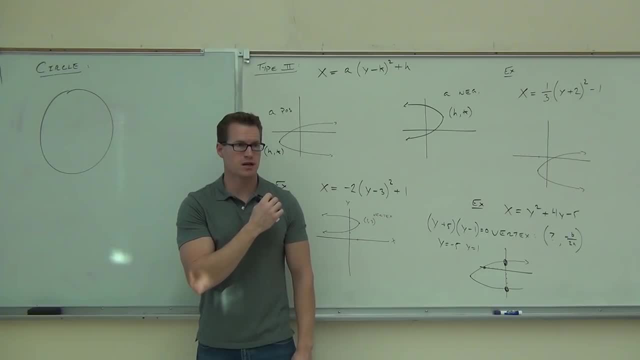 So I have some rope. Can you draw a circle with two sticks and a rope? Yes. How would you do it? Say what? 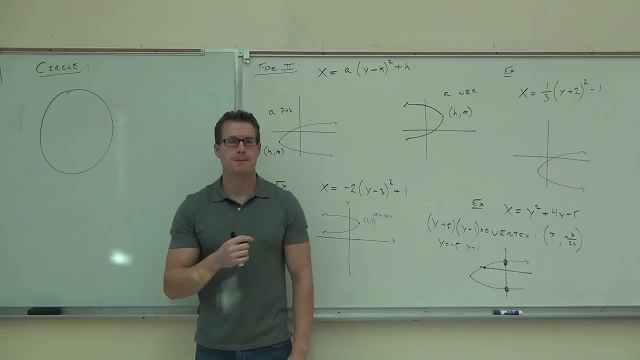 I would put the two sticks, like one more down, one vertical, and then trace a string and connect it all the way around. Okay. 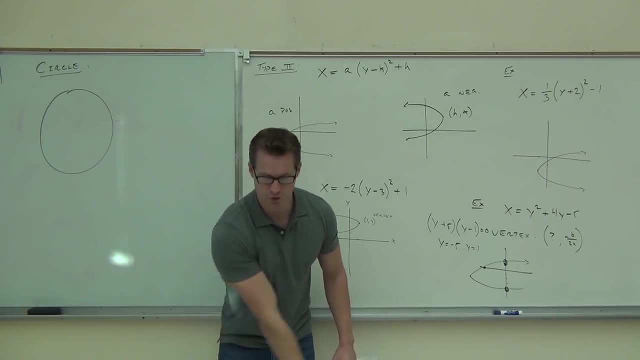 What if I meant that I want you to draw a circle in the sand, like you just go and make a circle. How would you do it? Think about it. 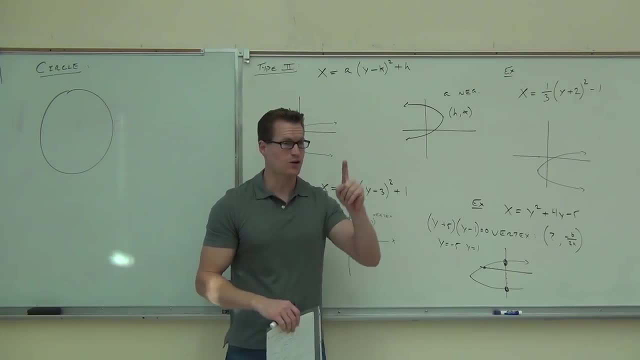 You have two sticks or one stick and your finger. You have a finger if you want. You still have fingers. And you have a rope. How would you do it? Tie the rope to the two sticks and then go around. Tie the rope to the two sticks. One in the middle. Okay. 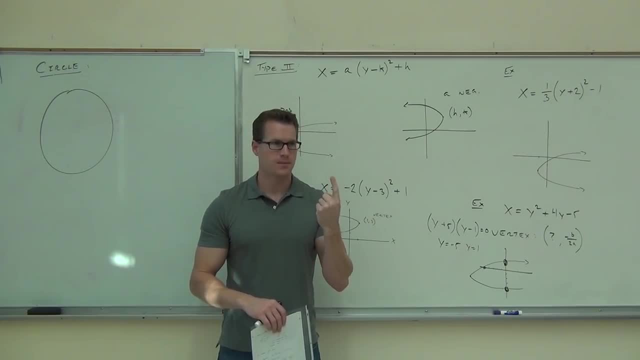 And all the way to the end of the rope. And then go around. Is that going to make a circle? Yeah. Absolutely. That's a perfect circle. In fact, that's a definition of a circle. 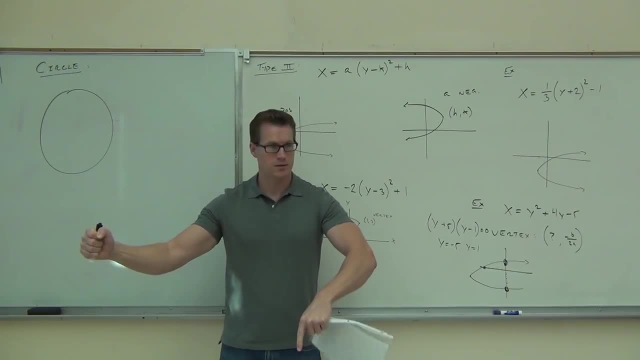 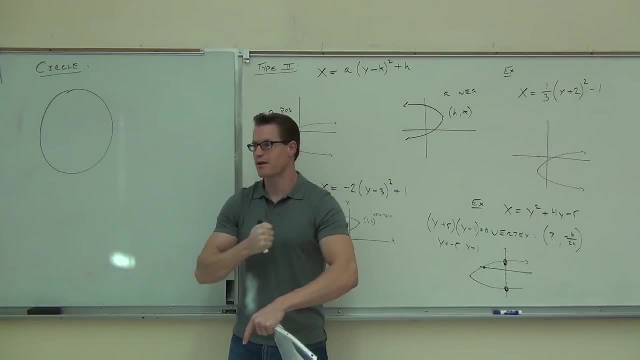 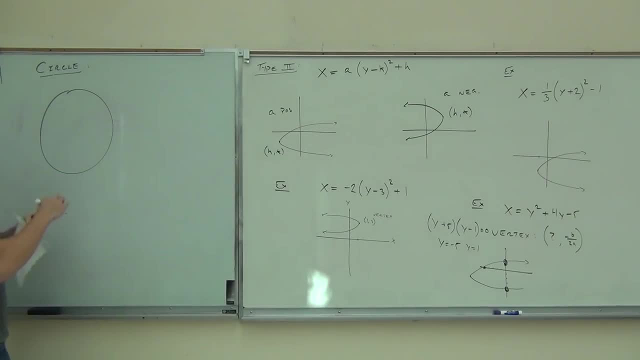 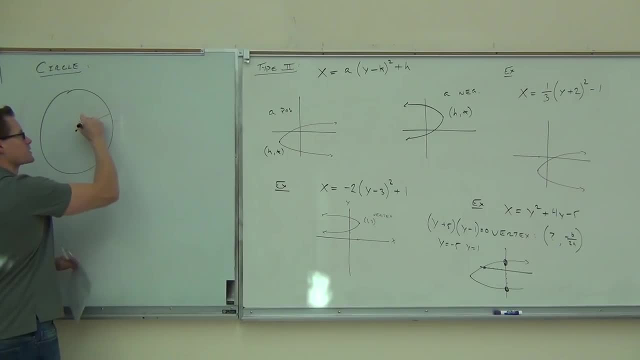 Circle. Circle. Circle. Circle. Central. Because one circle is a multiple circle. So a circle is just a set of points a fixed distance away from some center so that you have just created a circle. So when you talk about circle you mean we have this center point. We've got this thing, a rope going from the center to the edge of our circle. We typically call that a radius. It's weird to think about how you actually do something, how you draw a figure. But that's how you do something. You are drawing in a circle by sticking your finger in the sand and having a rope away from it and using the stick to draw. 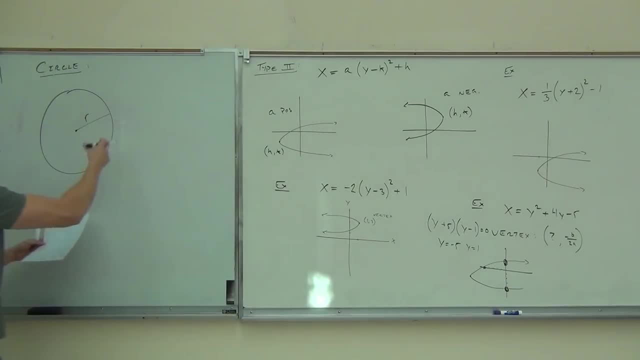 That's how people created circles initially. So that's our idea of a circle. 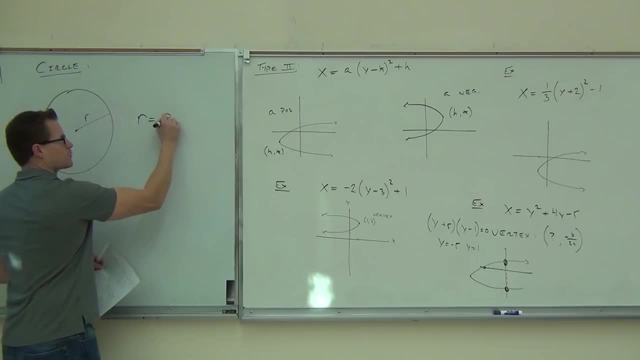 It's some radius, some distance away from some center, which we're going to call HK. 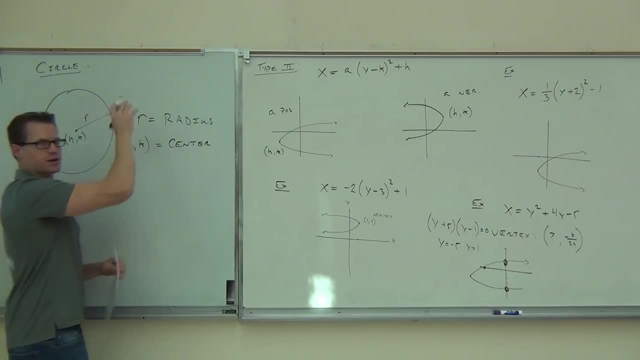 And the set of points that we get, all these infinite number of points connected to make our circle have the coordinates x comma y, just like normal points do. 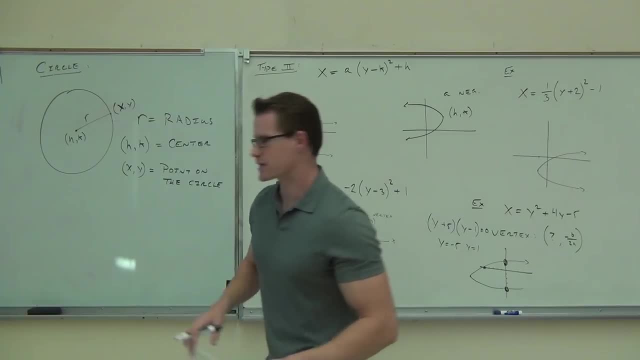 With this in mind, I'll give you the equation for a circle, and we'll come back to this next time. 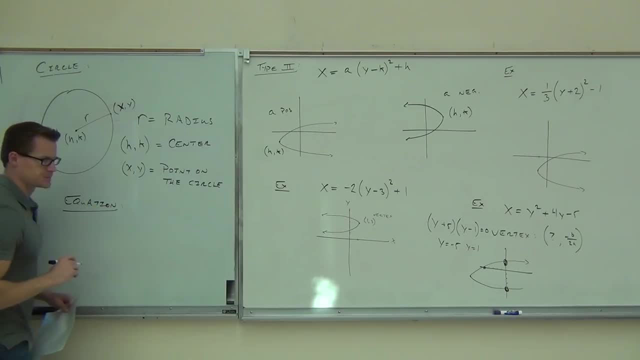 Here's the equation for a circle. If our center is h comma k, and every point on our circle is x comma y, and we have this radius r, the equation for a circle is x minus h squared. y minus h squared. y minus h squared. 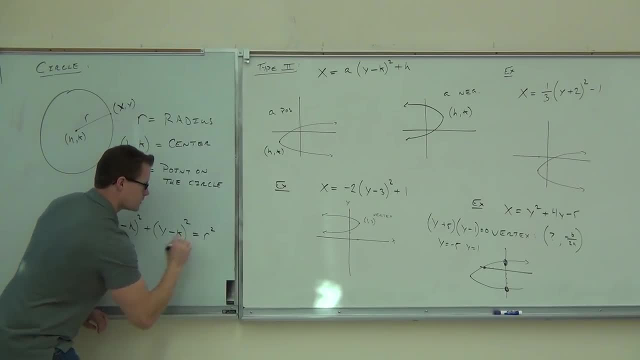 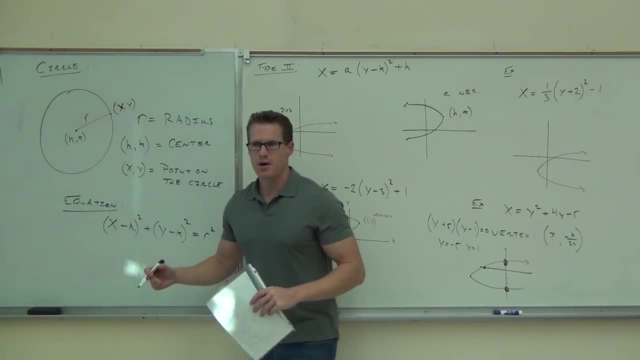 Now, this is going to be kind of cool. Do you remember how y means up and down and x means left and right? That's where our coordinates are. Notice how we're in parentheses here, we're in parentheses here. What if this minus h, minus h in our type 1 parabola ignored this type? 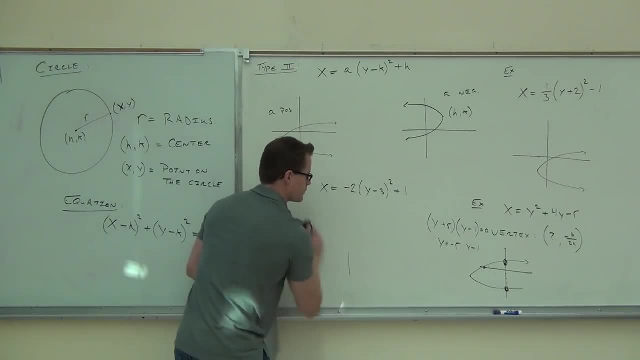 We're done with dealing with y as our independent variable. 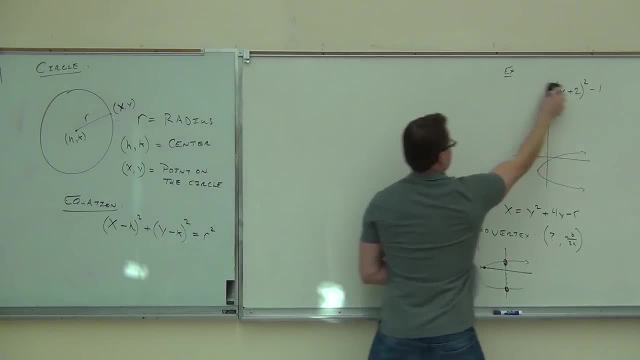 We now have two independent variables, x and y. So ignore this for a second. 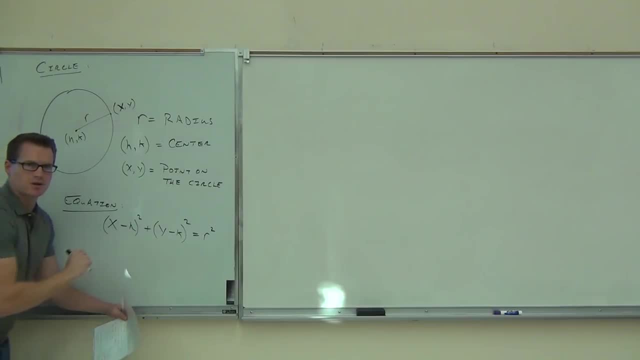 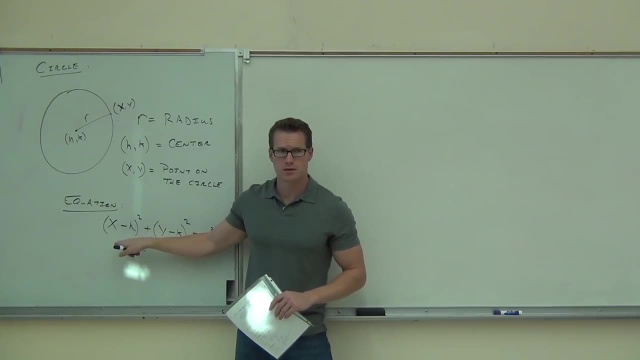 My question is, what did this minus h typically mean? This was left or right. Minus meant? No. Minus meant right. This k meant up or down, right? Minus means up here. Notice how it's in parentheses? Notice how it's in parentheses there? 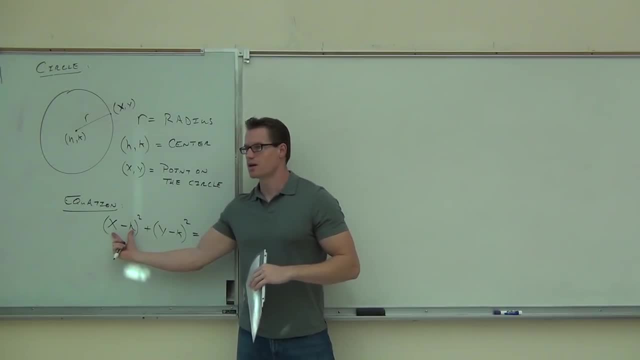 So it's like the opposite idea that we had. So this right here means our left and right still. This means our up and down still. In fact, our vertex, you can see it. Our vertex is, our center is found by h comma k. 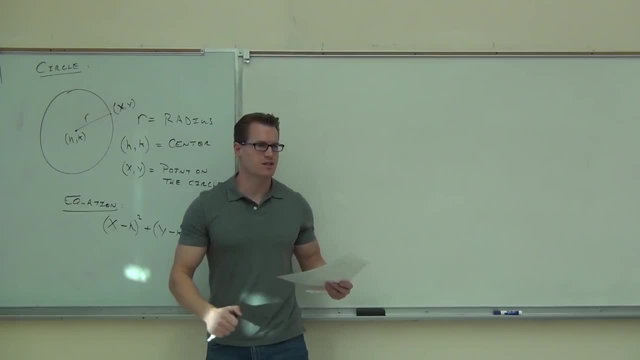 Our points are given by x and y. We're going to talk about some specifics next time. I'll show you exactly how to deal with that stuff. All right. 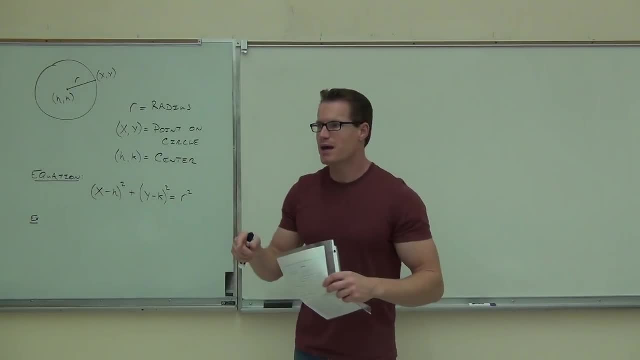 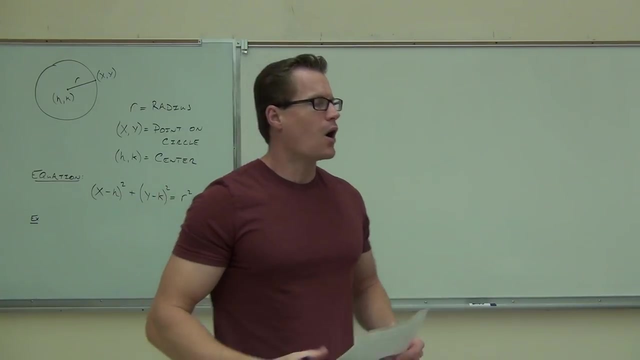 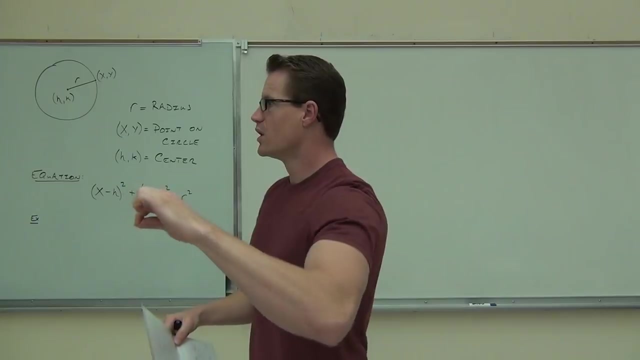 So we're talking about circles. We know these circles are these round shapes, and basically you make one up by sticking them up. By sticking something in the sand and getting a piece of string and drawing a set of fixed points around that stick, or basically we just draw a set of points around some fixed center is what we call it. Our center is always given by h comma k. It's going to be somewhere on your graph. R is the distance from the center of your circle to the, actually outside of your circle there, the actual points. 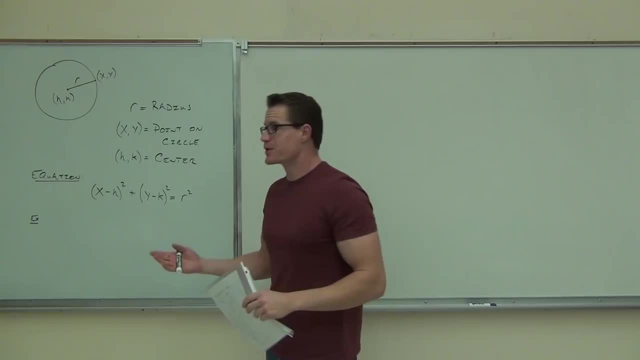 Every point is given by x comma y. So we have this shape that we're really familiar with. We just have never... We've never learned the equation and how to manipulate it. 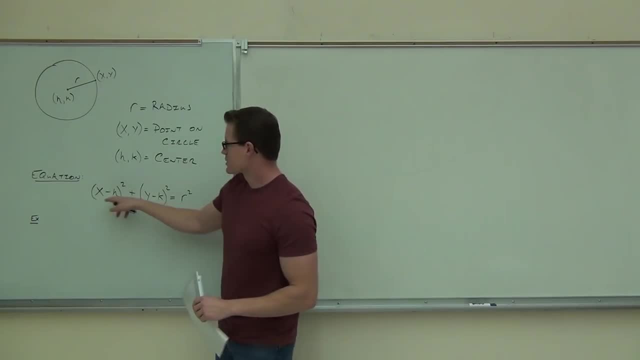 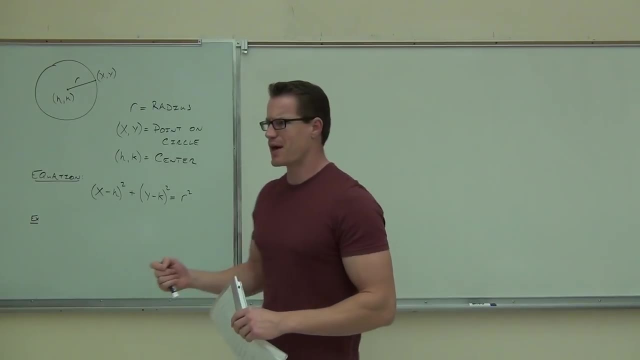 So we're going to look at that today. So our equation is right here. We have x minus h squared plus y minus k squared equals r squared. You can see a lot of squares on that, right? Even looks a little bit like the Pythagorean theorem because you have square plus square. It's not the Pythagorean theorem. It's a definition of a circle. 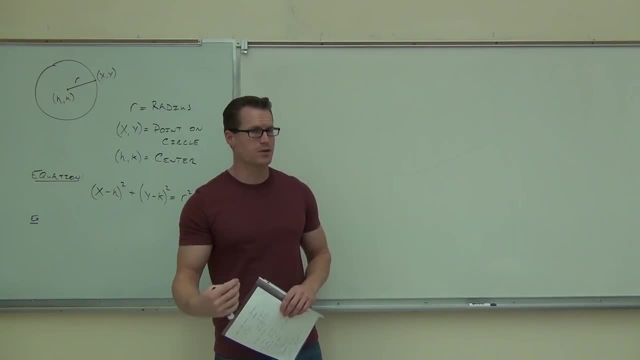 But I do want you to notice that a lot of things that we're familiar with in parabolas work here. For instance, with our parabolas, when we had this minus, if you ignore that for a second, that looks a whole lot like a parabola. It's not a parabola. 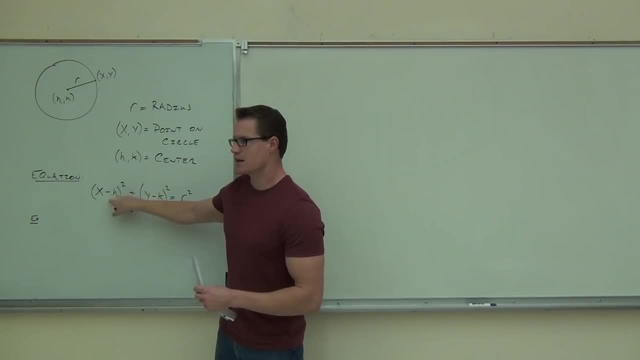 And that right there would say that this is a left or right shift. You follow me? That h was a left or right shift. 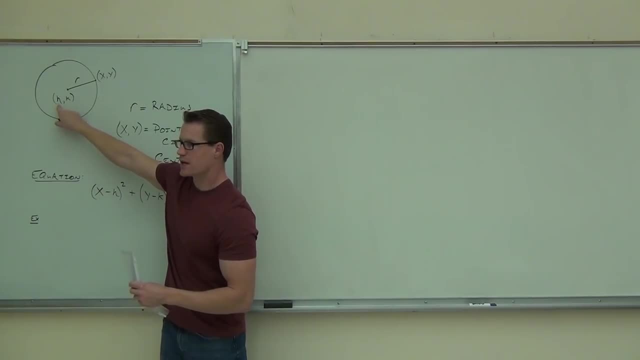 That's actually how we get our x coordinate. Notice how h and h, h goes with x, doesn't it? 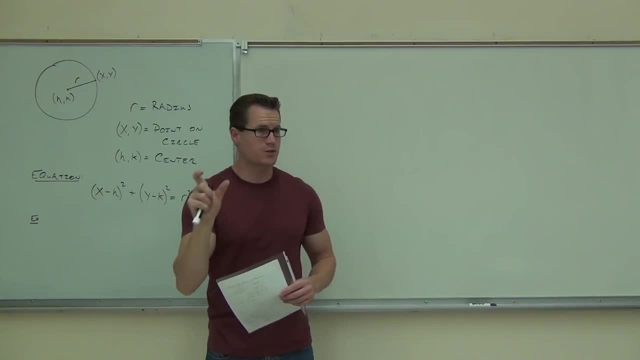 That is how we get our x coordinate. We're either a left or right shift. 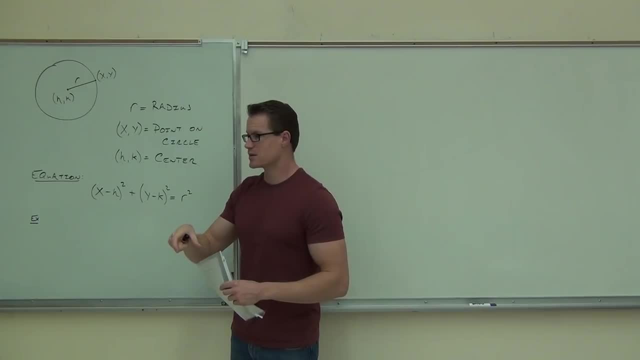 Minus means right, just like it did before. Plus means left, just like it did before. 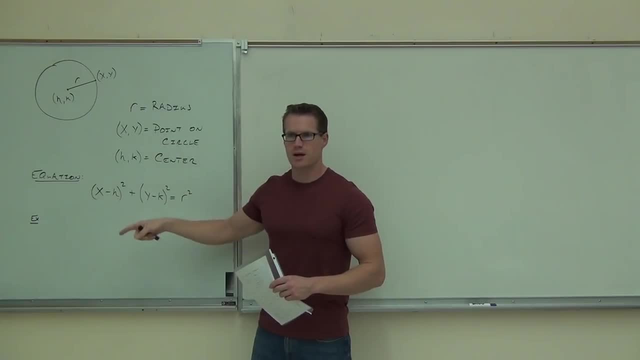 You with me on that? Now the y, y tells us our height, right? So that y minus k. 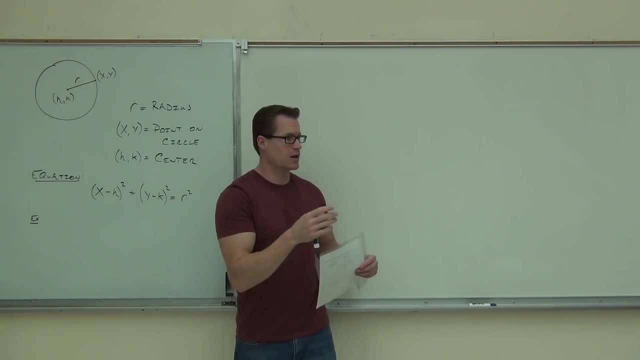 That k was also a shift up or down. Now, however, unlike parabolas where that plus k was up and the minus k was down, it's in parentheses now. And we know that really any time we have something in parentheses, it's kind of backwards of what we want to say it is. So whereas a minus would mean right and a plus would mean left, a minus means up 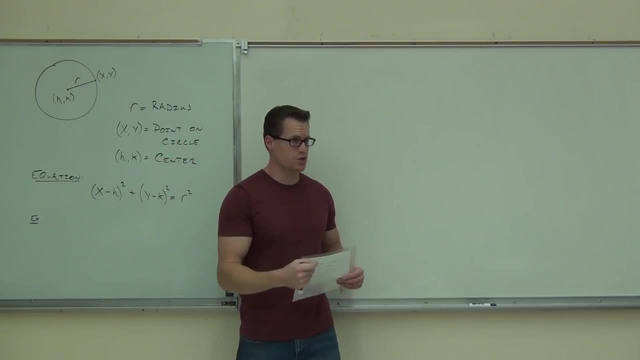 and a plus means down as far as the shifting goes for the center of our circle. Are you okay with that? So that's how it's going to work. 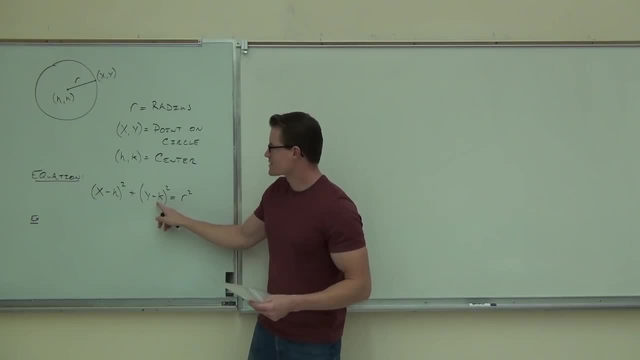 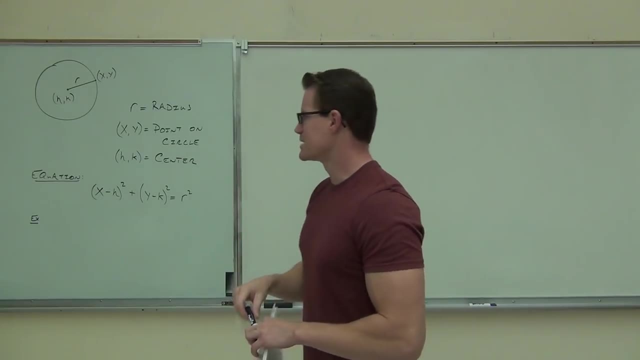 Very similar to the shifting of a parabola. And you'll notice that that's also how we find our center here, too. That minus k, that's given us part of the center of our circle, the y coordinate. Let's look at an example and see exactly how this works as far as finding the center of our circle goes. 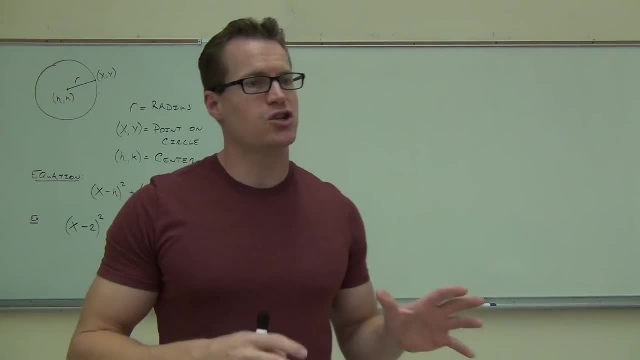 Firstly, I need you to be very good at identifying that this thing is actually a circle. How do you tell when something's a circle? Well, here it is. 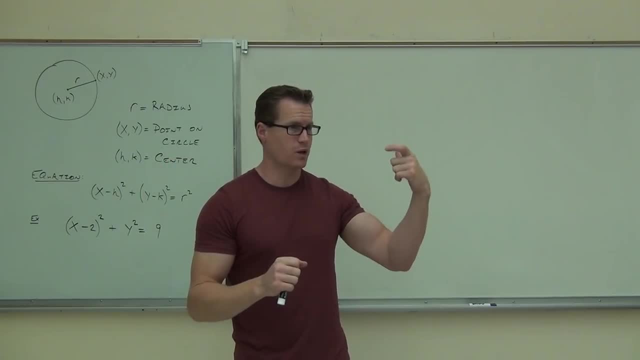 You need something squared plus something squared equals a number. So is it a circle? Do I have something squared? Yes. Do I have the plus? Now, I'm going to really emphasize the plus here because our next shapes have a minus there and they're going to be different, all right? So there's a plus, there's a square, there's a square equals a number. That's definitely a circle. Are you okay with the idea that this is a circle? Really, we're looking for a square, a square with a plus in the middle of it. 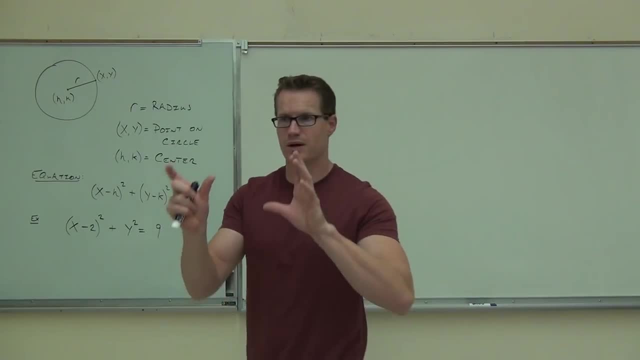 That's the whole definition of a circle. X squared and a y squared and we have some plus. 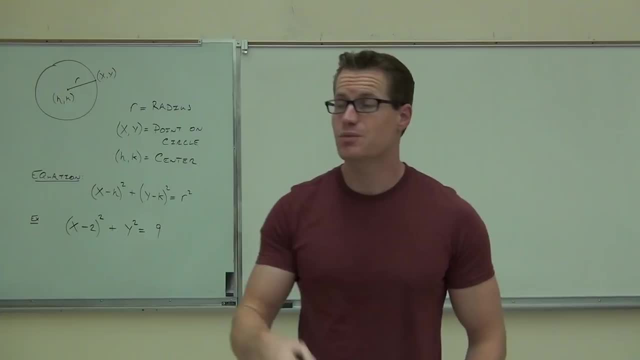 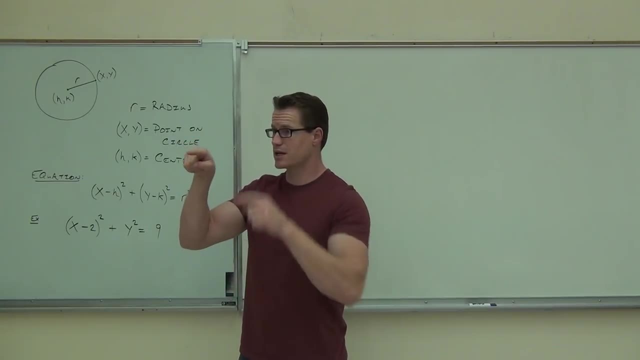 Now, we also have to identify a couple things about it. We've got to identify the radius. We've got to identify the center. But have you noticed that with circles, all you really need is two pieces of information? You need where that circle's centered and you need how far apart to put your points. That's really it. 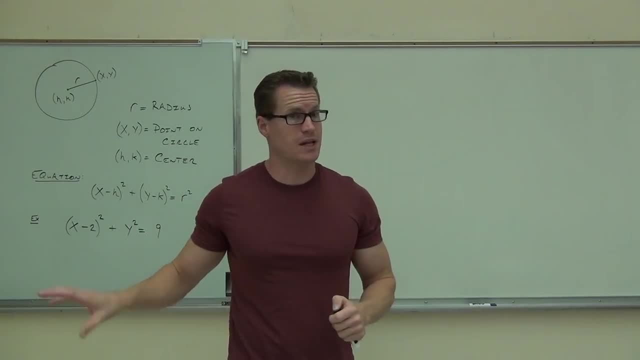 So if we can identify those two things, we should actually be able to graph this and that's what we're going to do here. So let's go ahead and try to identify the center. We're going to try to identify that. 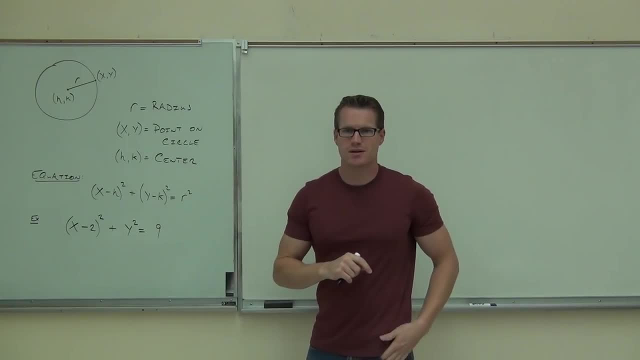 Can you tell me by looking up here, how much is the radius? A lot of people are going to say nine, but I want you to look at that. This is the radius squared. So could you write this as something squared? Yeah, you could. 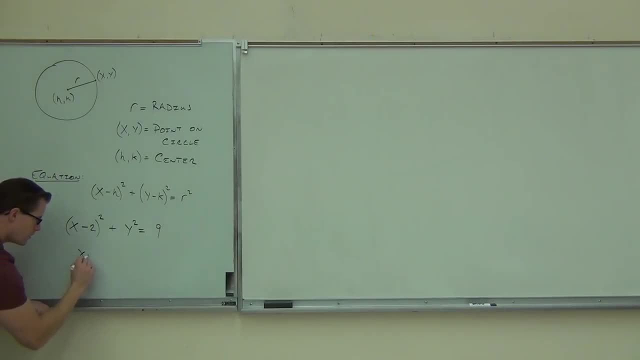 You could actually write it as, same thing on the left-hand side, but yeah, we could write that as three squared. 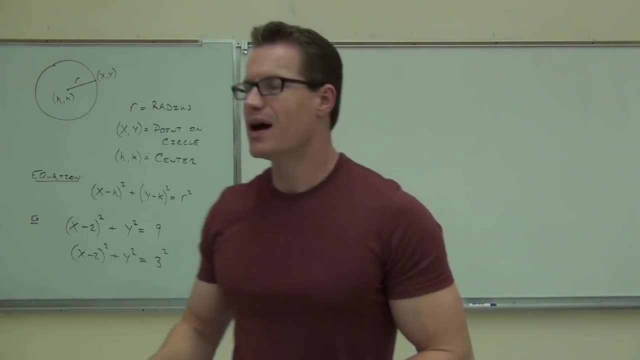 That means the radius isn't nine, is it? The radius isn't just that number right there. I'll tell you what. It's a number. I'll tell you what, on a multiple-choice test, of course, what am I going to have is one of the options for an answer. Nine. 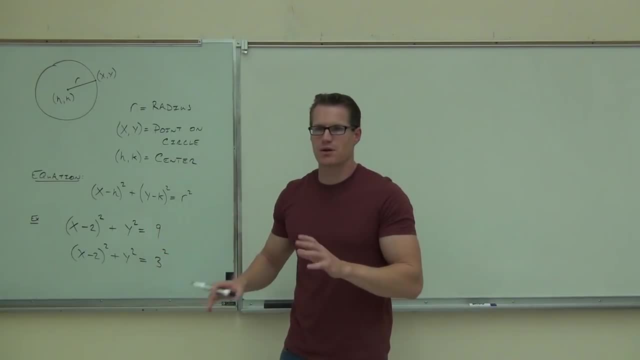 I'm going to have an option for the radius of nine, of course. I mean, because a lot of people, if they don't understand this, they're going to go, oh, yeah, the radius is nine. Yay, I win. 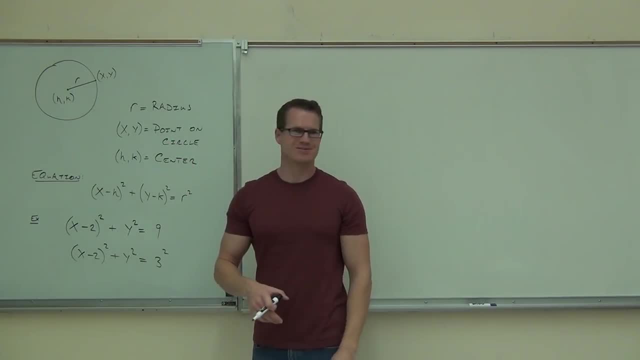 And you're going to see the problem on your test and be like, yes, ten points. Nope, zero points. 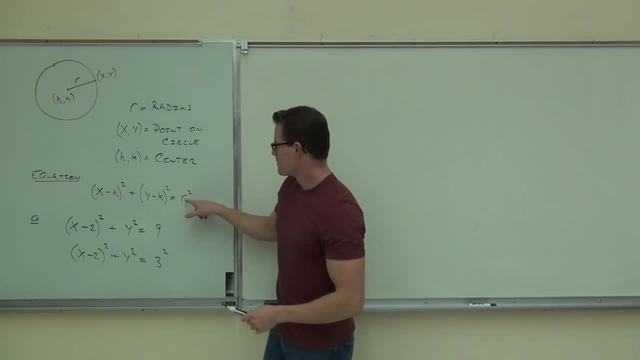 Because you need to understand what this formula says. This formula says that this number right here is the square of the radius. So whatever you have here, how are you going to find the actual radius? Square. Square. Not square, this is already squared. No, no, no. 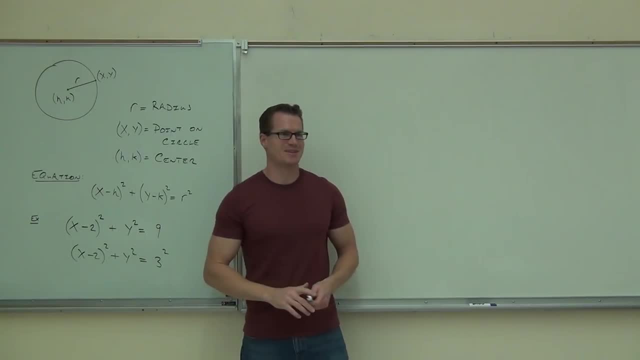 You're going to unsquare it. What's unsquare it mean? You're going to square root it. You're going to find the square root of it. So what's the square root of nine? That's your radius. 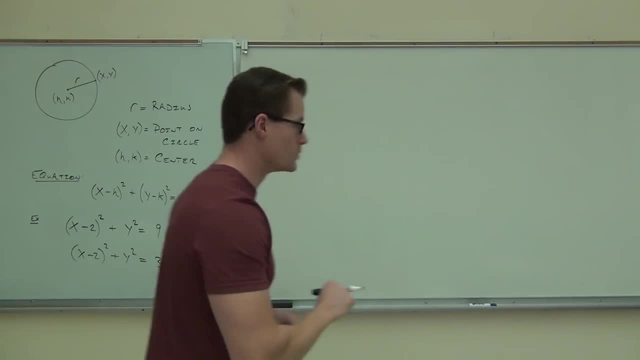 So let's identify a couple things here. This is the only two things we've got to do. Identify the center. Identify the radius. 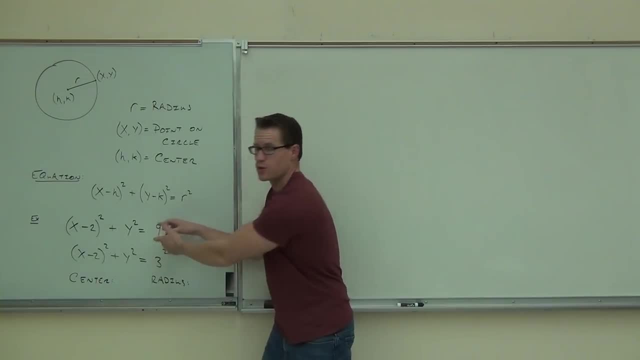 Again, our radius is the square root of whatever number you want to have. Why? Because we can write it as this number to the second power for our radius squared. 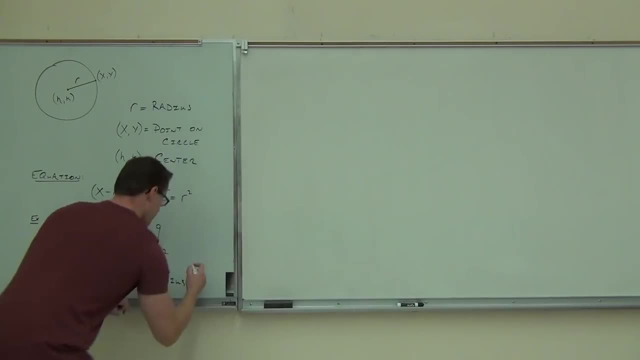 So right now our radius is three. That's kind of an important thing to know, right? 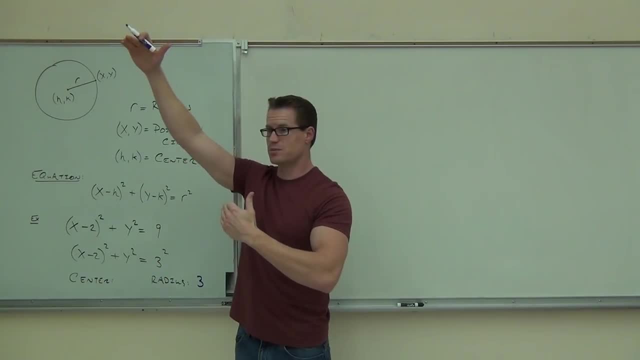 If you had nine, your radius is going to be three times as long as what it should be. It's going to be a big circle rather than a normal size circle that we should have here. Way too big of a circle. 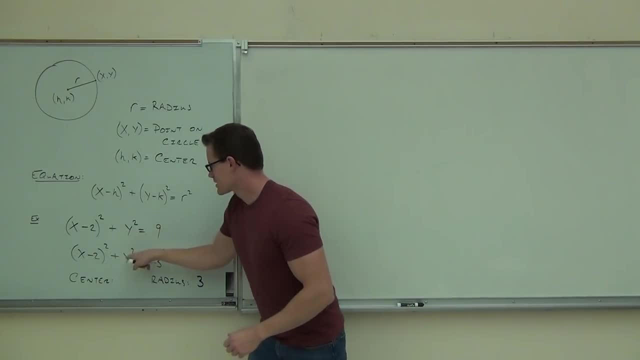 Now the center is also really important. We've got to be able to translate this into finding the center. 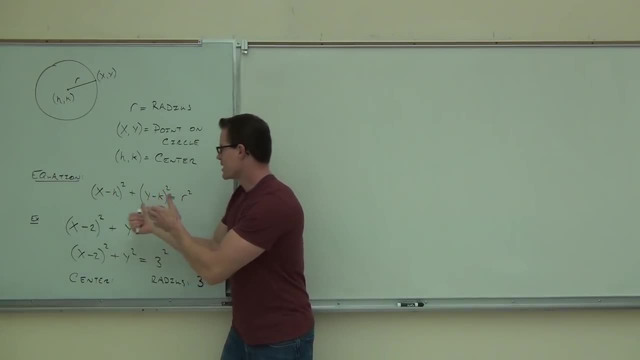 If our center is x minus h and then y minus, if it's given by the h and the k, let's look at that. What is our h here? Two. Two. And if you look at that, it says minus two, that would be, now this is going to be a little bit, hopefully not weird for you because it works just like a parabola did earlier. 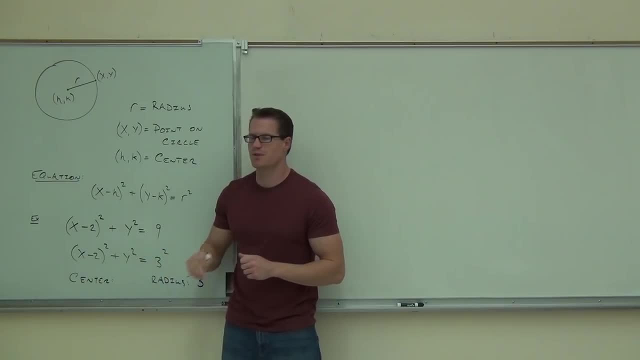 Is our center negative two comma something or two comma something? Think about it before you answer. 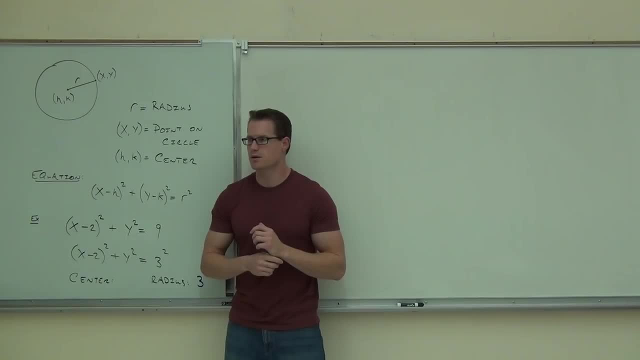 Two. Negative two or two? What do you think? Two. Negative two or two? Two. 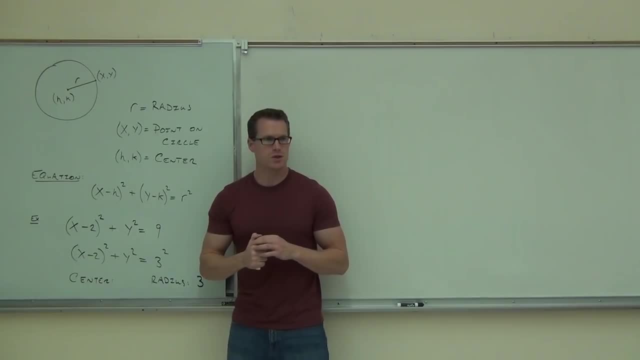 It says minus two there, I know, but I want you to think about this before you answer this. Would this be a shift to the right or left? To the right. 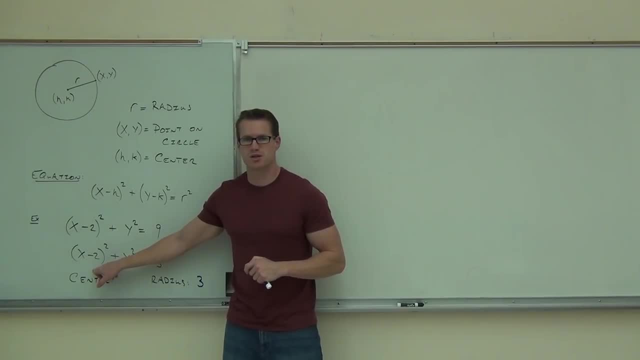 That would definitely be to the right. That minus two would be a shift to the right. Eyes up here with me, okay? This would be a shift to the right. Are you with me on that? So is that going to be negative two or two? Two. 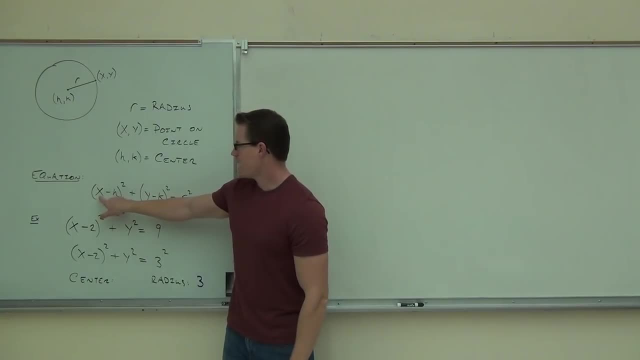 And I want you to look at the formula. The formula says x minus h. Yet our center's at h. Are you with me on that? 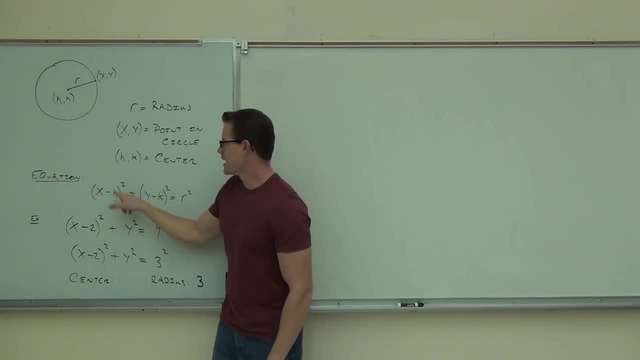 So if it says minus h, well, if you want to think about it as taking the opposite just like we've been doing the whole time, that's what you're doing here. 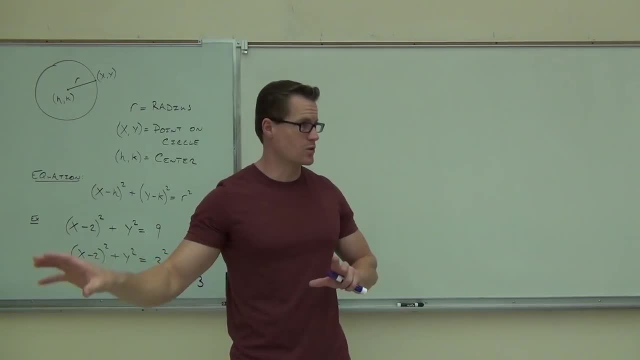 This is a shift to the right two units. That means that if it says minus two, you're getting two. If it said plus two, what would you have? Negative two. 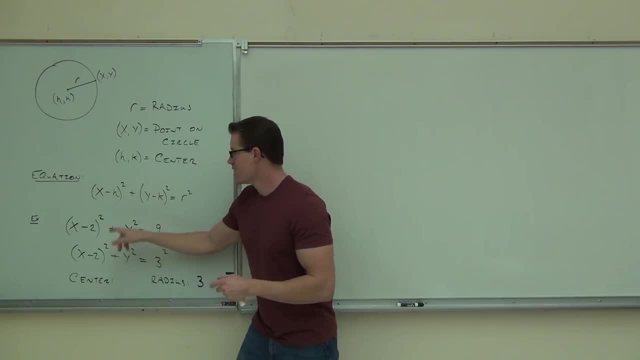 Negative two. Yeah, just like a parabola. So our center is at two comma, well, now wait a second. Hang on a second. This says just y squared. Does that add up? Negative two. Negative two. Yeah, just like a parabola. 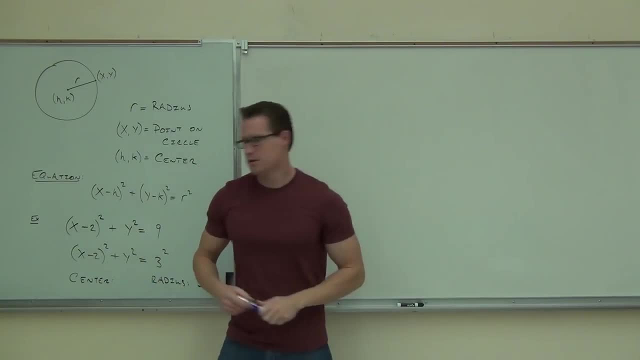 So our center is at two comma, well, now wait a second. Hang on a second. This says just y squared. Does that add up? 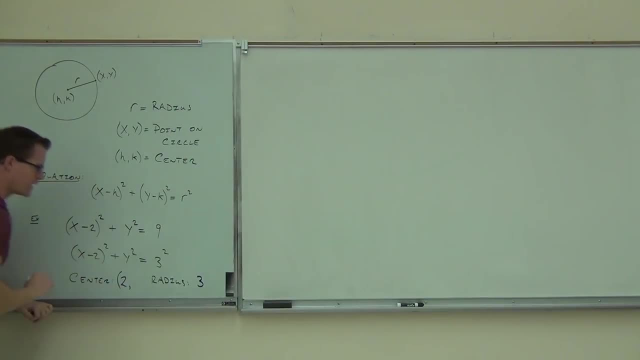 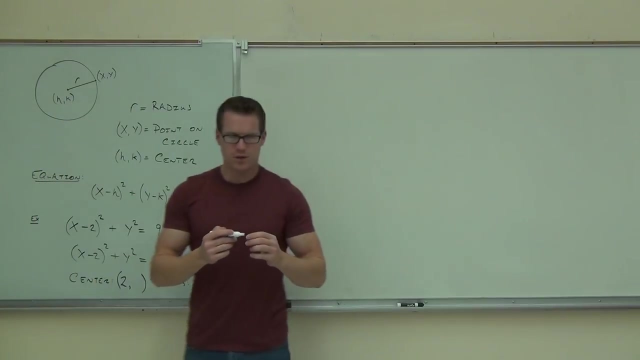 Does that have a coordinate there? It's got to have a y, right? It's got to be a point. So what would I put there? What's being subtracted from the y? Is anything being subtracted from the y? Negative two. 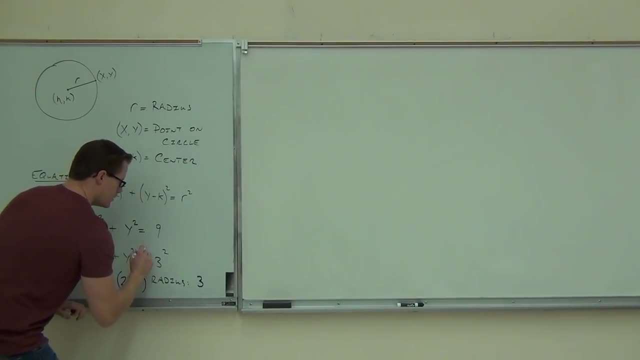 Negative two. So from here, notice that I could do minus h, negative two. 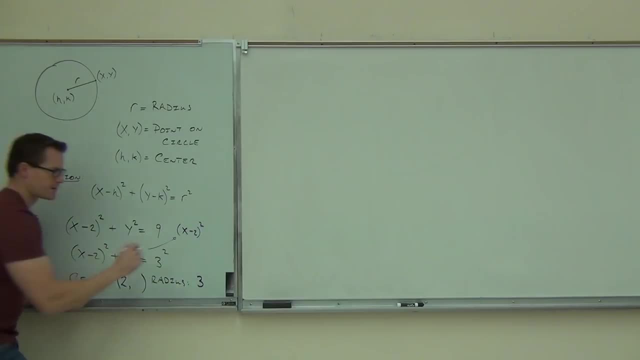 X minus 2 squared, that's that, plus, how would I represent Y squared? I could do Y minus 0 squared. Is this the same thing as that? Yeah. Yeah. So what is our, what's our coordinate for our Y? 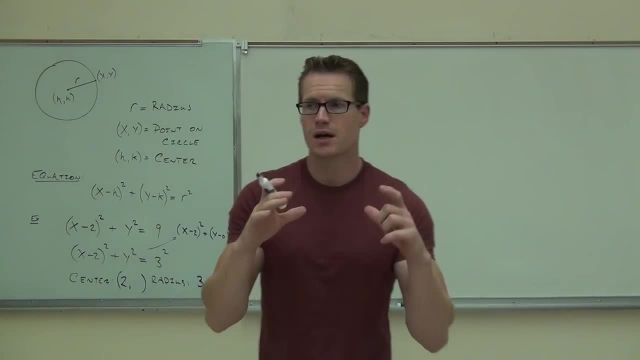 So long story made short, if you don't have anything in parentheses, your center, part of your coordinates is 0. 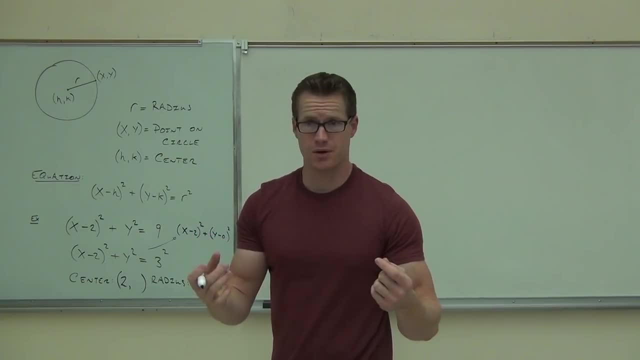 So if I have Y squared, that means the Y coordinate is 0. Rich, how do you feel okay with this so far? Right, so this would be 2 comma 0. 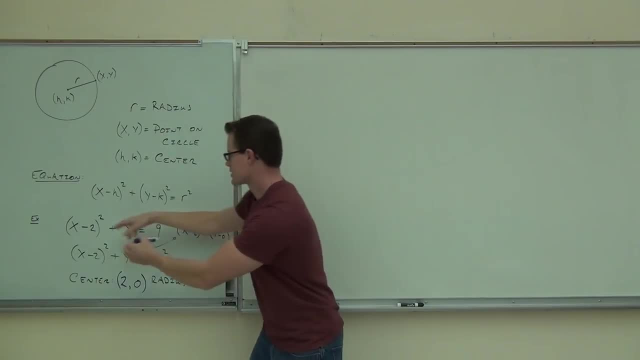 So radiuses are R. Our points are X comma Y. That's why we still have an X and a Y in any problem that we're going to have with circles, you have to have an X and a Y. That's how we plot points. 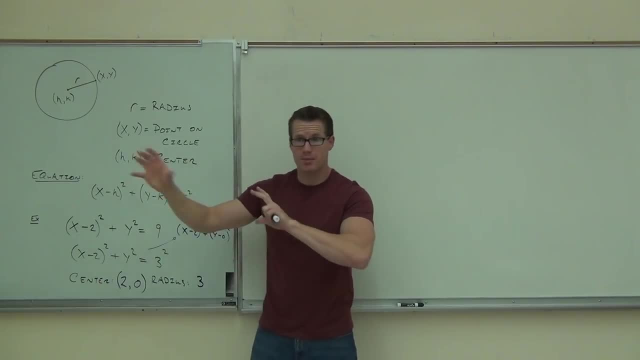 Our center is given by HK, and we know that it's kind of backwards like parabolas are in finding our coordinates. 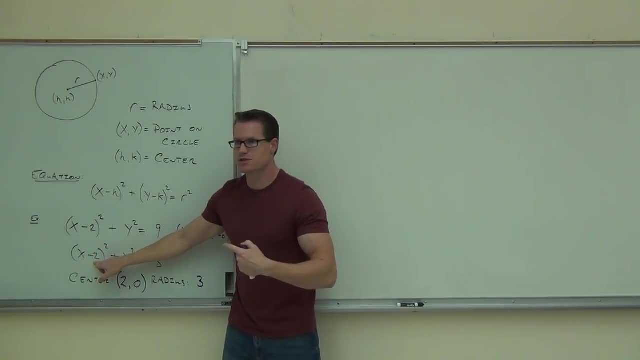 So if we have X minus 2, our center is not at negative 2, it's at 2. Of course. Of course, I'm going to have a center at 2, 0 on your test, right? 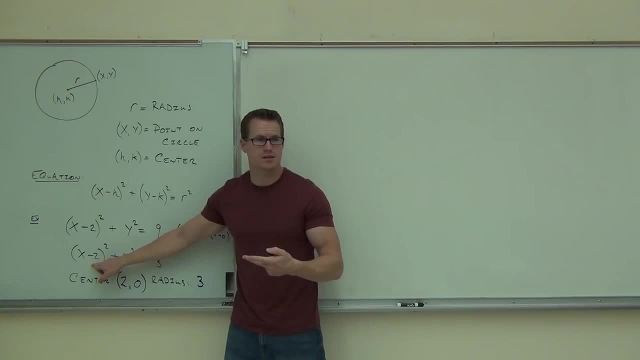 And I'm going to have a center at negative 2, 0 on your test. 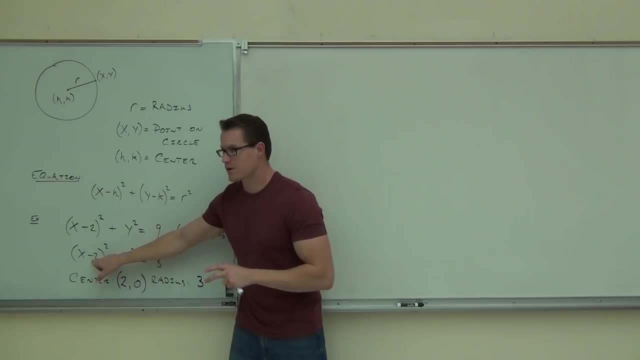 So that way I understand whether you know that this, whether or not you know that this is a positive 2 right there because of the shift to the right of two spots. 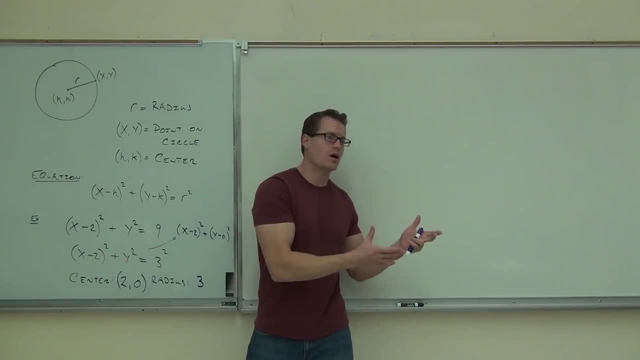 If we don't have a number being added or subtracted, that's like adding or subtracting 0. That means that we're going to have a coordinate of 0 if we don't have any number associated with one of those X or Y coordinates. 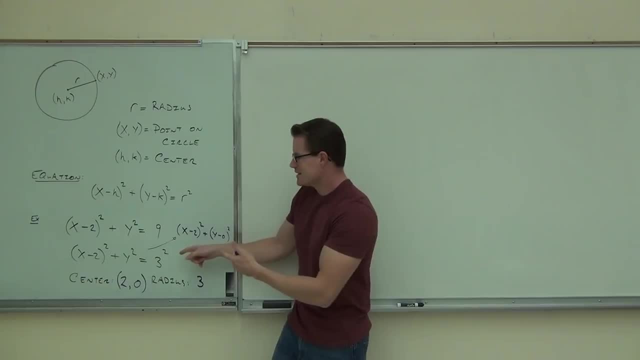 So we have here 2 comma 0 for our center, and our radius is 3. Not 9 because we're taking a square root of that number, because we know that the number off to the right is actually R squared. You still okay so far? Now let's graph it and see how to do that. 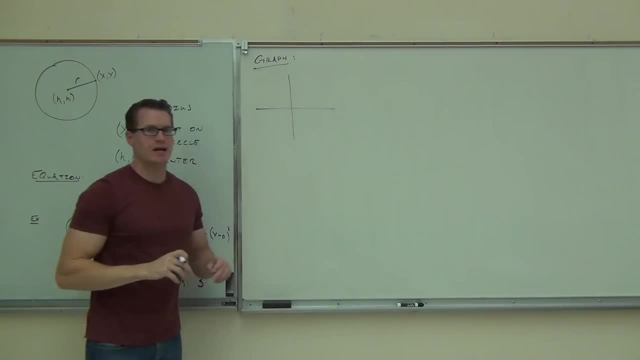 Now fortunately for us, there's only two things we've got to know about graphing circles. We've got to know the center. We've got to know how far apart to put our points from the center. So our center, we're just going to put that point somewhere. 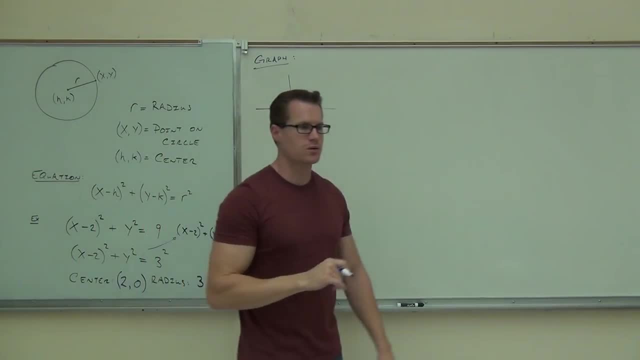 So our center is at 2, 0. Go ahead on your graph right now, plot 2, 0. 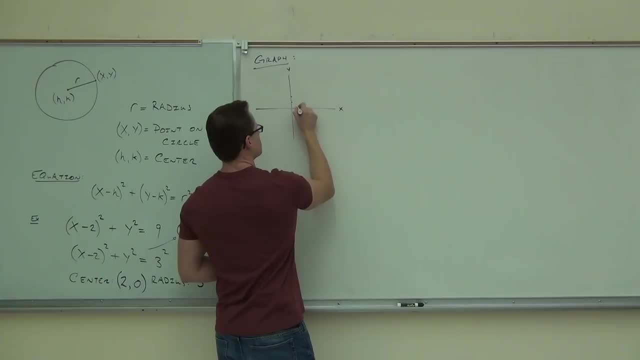 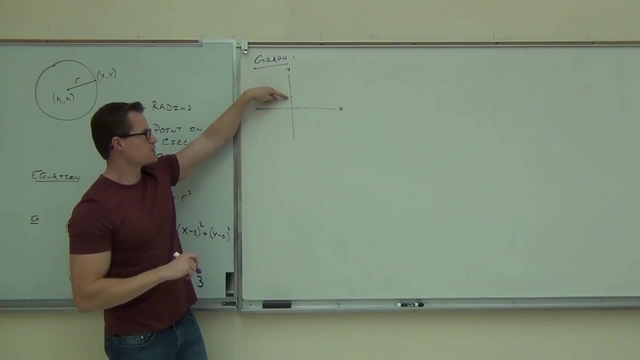 Where is 2, 0? Is 2, 0 up here? No. 2, 0 right here? Yeah, that's 2, 0. So we're going to put a integer right there. 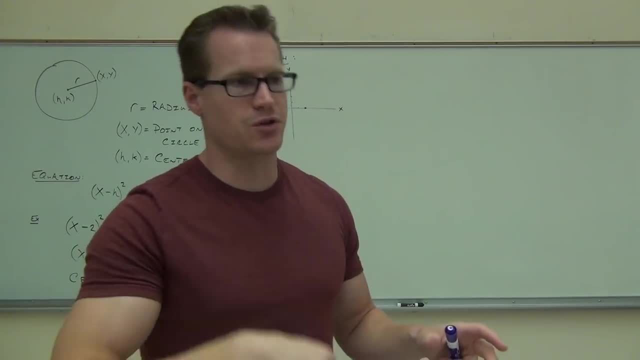 After you find your center, you're going to use your radius to make your circle. How much was our radius? 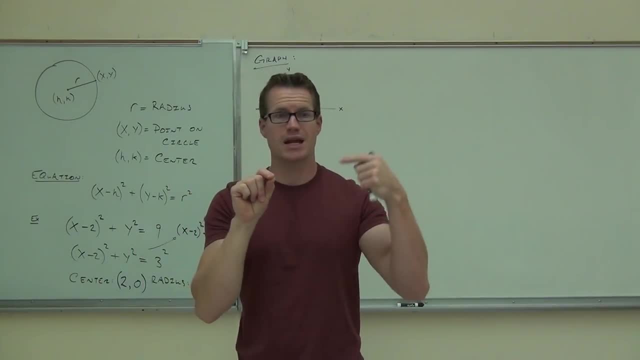 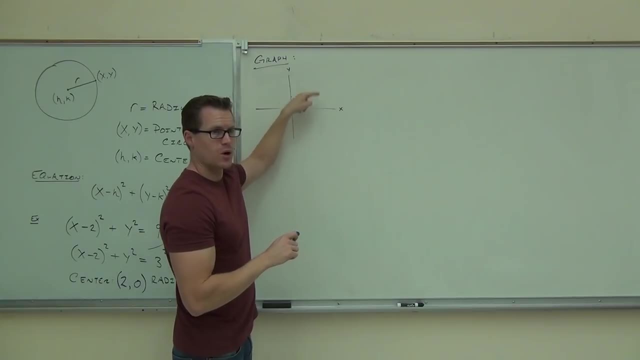 Radius means that from your center, you go out three units in every single direction. True? Now it's really hard. It's really hard to go in this direction three spots. However, can you go up three? Right three? Left three? Go three directions, three units in every single direction right now and put a little dot. So I'm going to go from here up three spots. 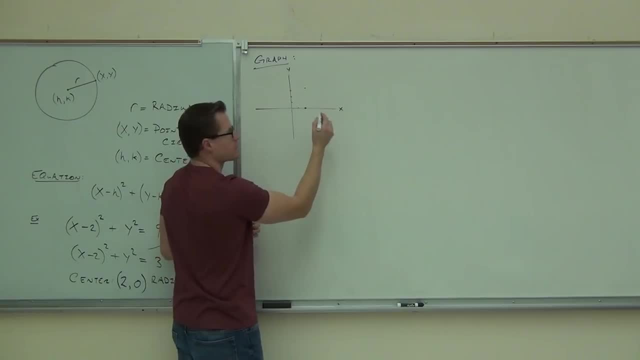 One, two, three. I'll put a little dot right there. I'm going to go to the right three spots. I'm going to go down three spots. And I'm going to go left three spots. Try that again. Try to make a circle. 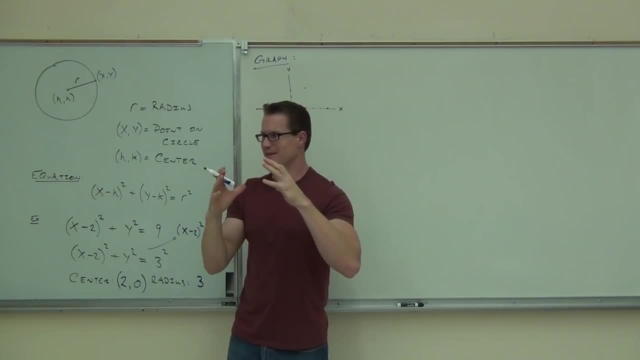 Try not to make a weird diamond-looking shape thing, okay? These are circles here. 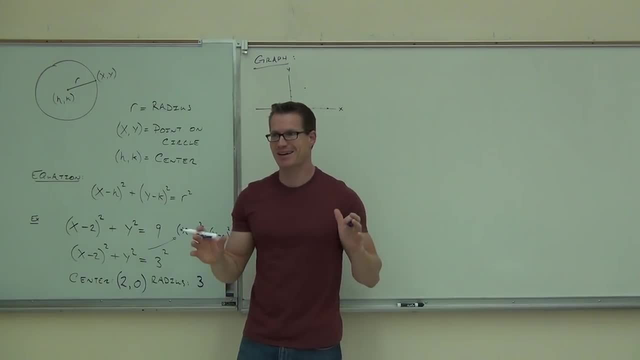 I'm horrible, horrible at drawing circles. I really suck at it. But hopefully you're better than me. 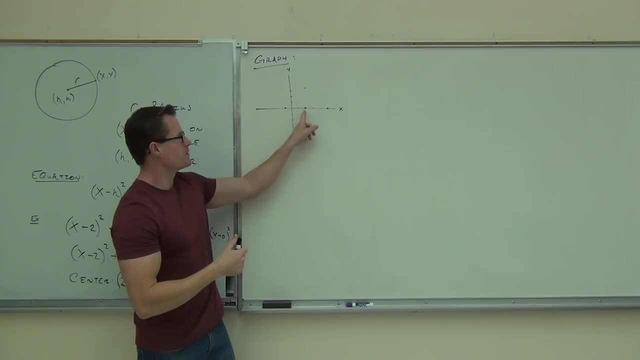 After we make those four points, notice that these are all three units away from that center. That's going to make a circle for us. 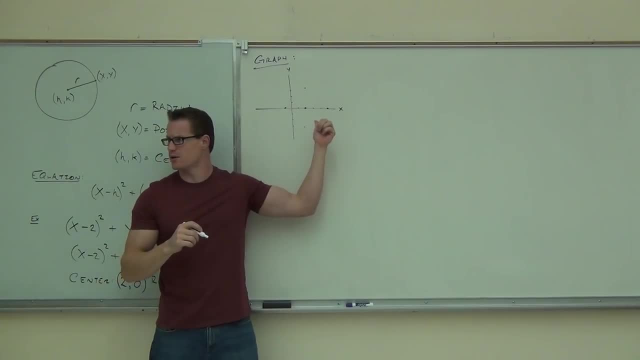 So if I connect those three points, first say, are you going to give a head nod if you're okay at getting those three points? 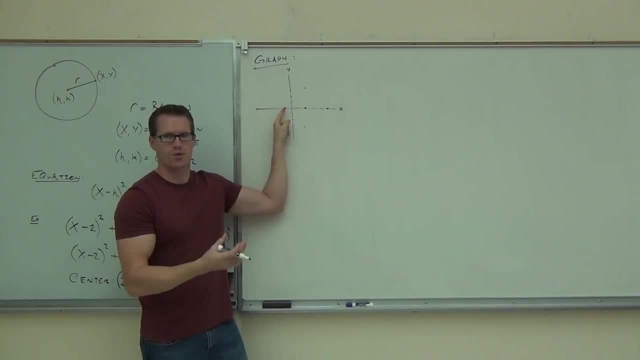 Yes? So from our center, not from the origin, right? Because our center is not at the origin. 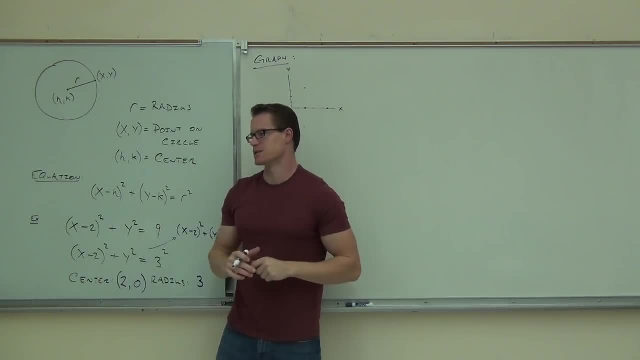 So I don't go from the origin every time. I go from where my center is every time. So if my center's here, I go up three, right three, down three, left three, from that spot. 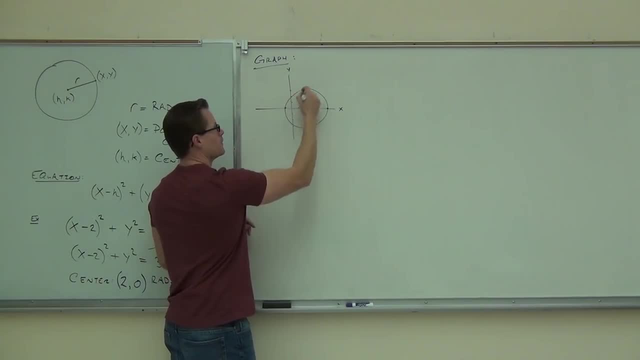 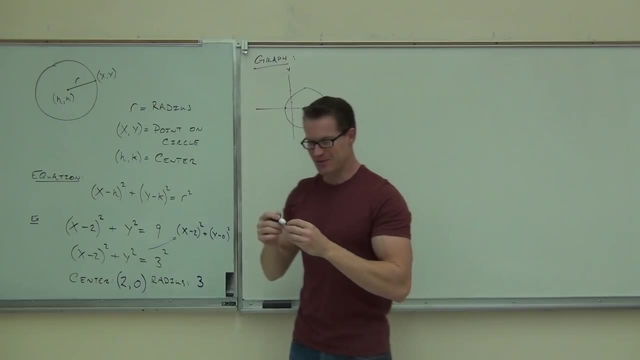 And then, oh, that's one of the better ones I've drawn. That's pretty good for me. I'm happy with even that. It's still better than the other one. Usually they look like weird footballs. You ever watch Family Guy? Yeah. 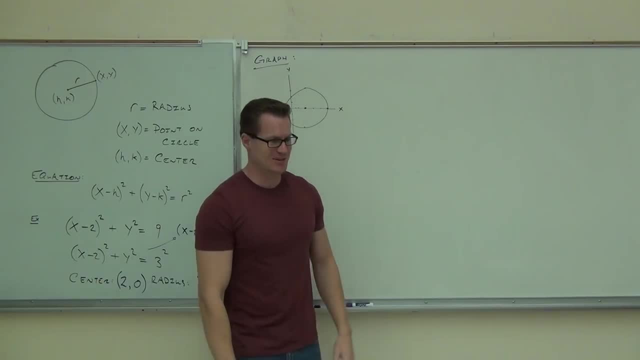 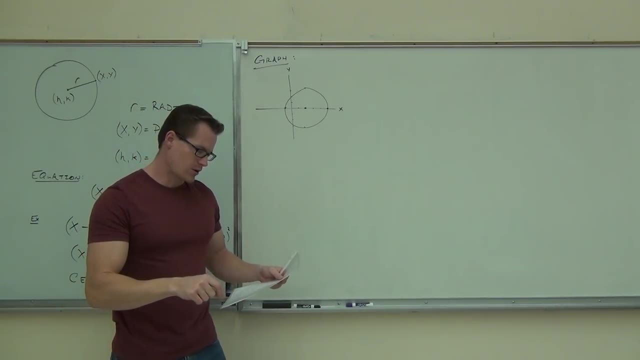 I draw a lot of stewy heads on my . It looks ridiculous, but. Why don't you? Okay, now, I would like you to, well, actually, let's try a couple more on your, together, and then I'll give you a couple more on your own. 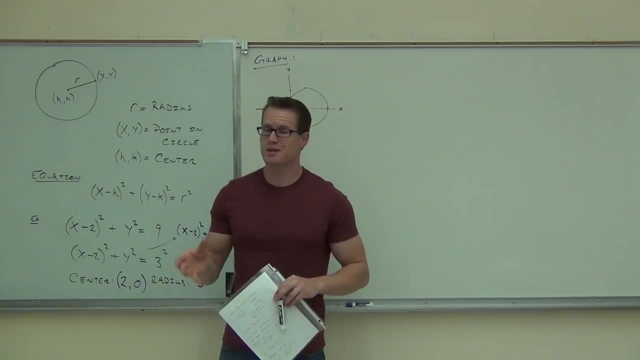 Just to make sure we really get this idea, I want you to be really good at drawing circles, because the next shape that we're going to talk about, ellipses, are really similar to our circles. Okay, there's two things we need to know. How about circles? First, the center next to the radius. 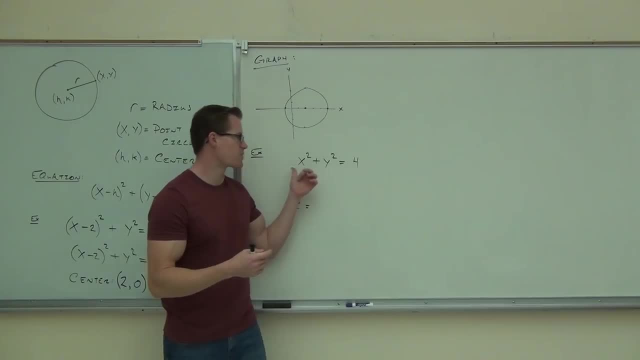 Before that, though, we've got to identify that they are, in fact, circles. So, let's look at this problem on the board here. 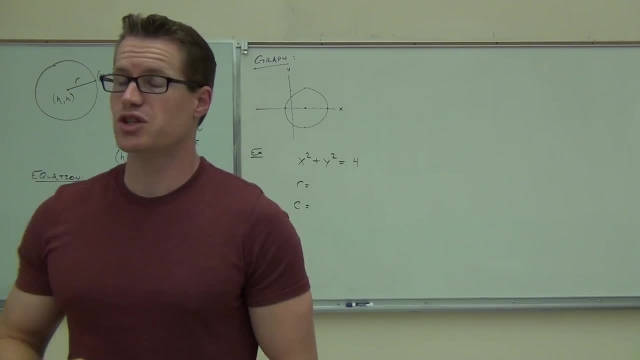 X squared plus Y squared equals four. Can you tell me whether or not that is a circle, just by looking at the formula? Yes. 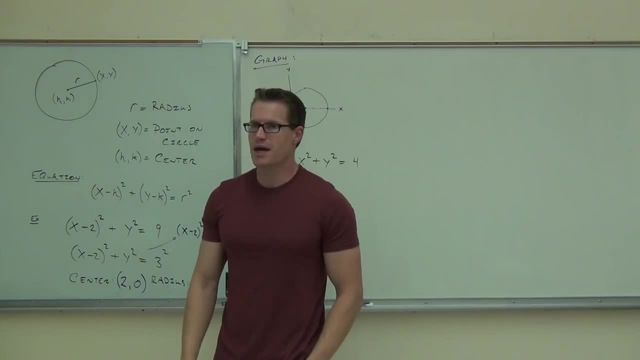 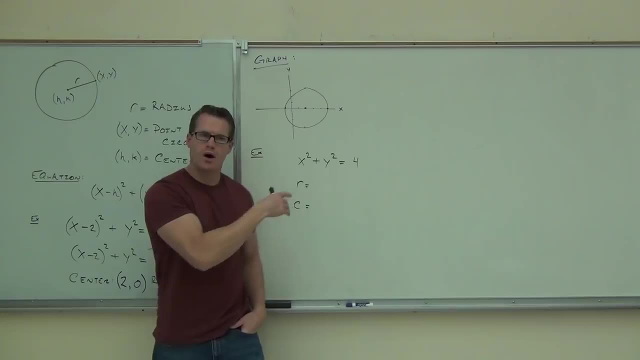 Okay, so if I gave you four choices and said, what is this? Is this a circle, an ellipse, a hyperbola, or a parabola? Well, you know automatically, you don't even know what those shapes are, right, since it's a parabola, but you know automatically that that thing is a circle. 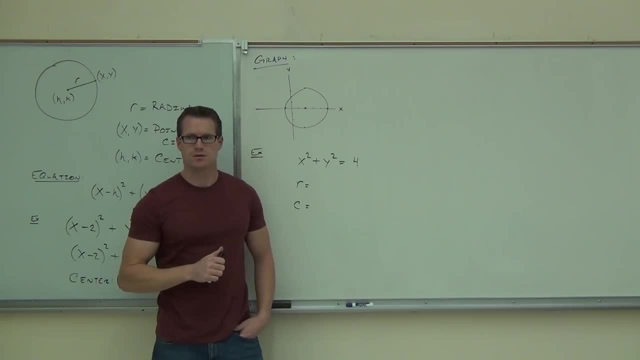 Tell me why that thing is a circle. That's how they explain it to me. 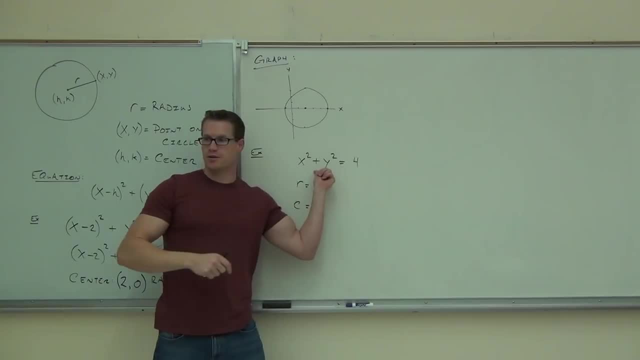 These are both squared, yes, and there's a plus in the middle of it. That right there, and there's the same number in front. We'll talk about that in a second, but we have squared, squared, and there's a plus. That means that we're going to have a circle here. You okay with that so far? 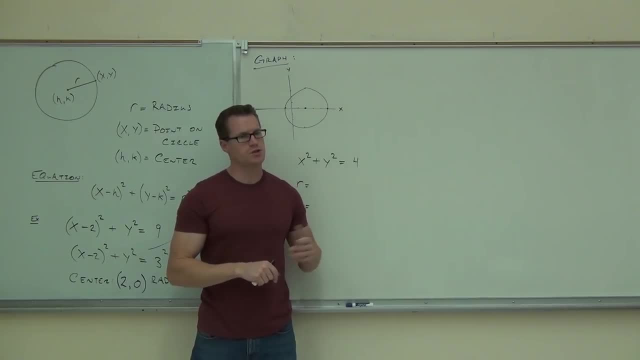 Now, it's up to you to find the radius and the center for your circles. So, first thing you've got to do, look at the radius. How much is the radius here? Two. Why? 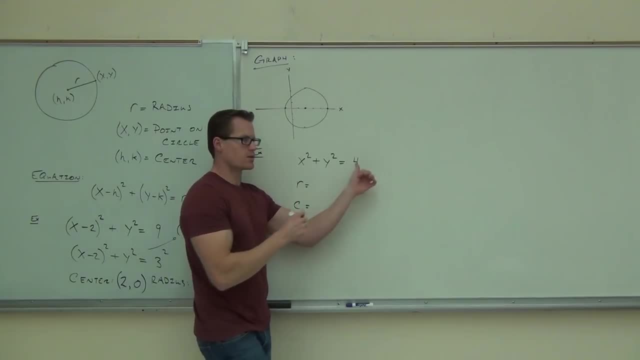 Because it's going to be . Okay. So, we know right here. 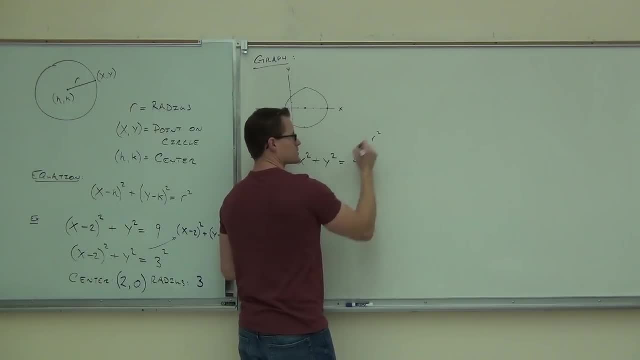 This number is actually the radius squared, or in our case, this is two squared. That means our radius is two. 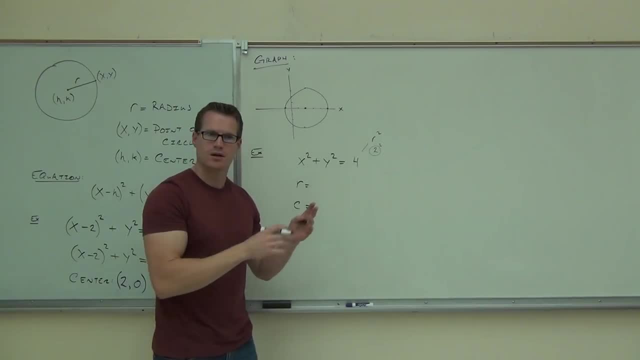 If you take the square root of whatever number I give you, you're going to get the radius. So, our radius is two. Not 16, not four, two. Hey, what about my center? Can you find my center here? 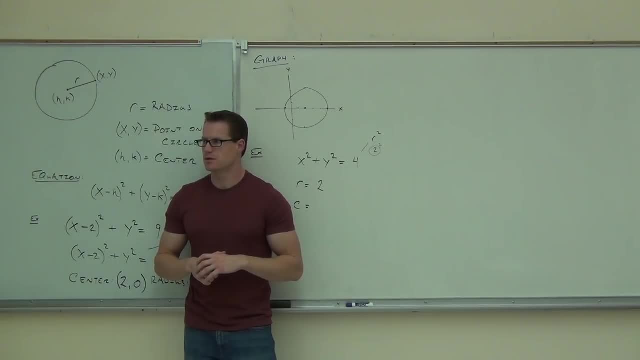 Zero, zero. Why zero, zero? Because it's x minus zero over square root of y minus zero. 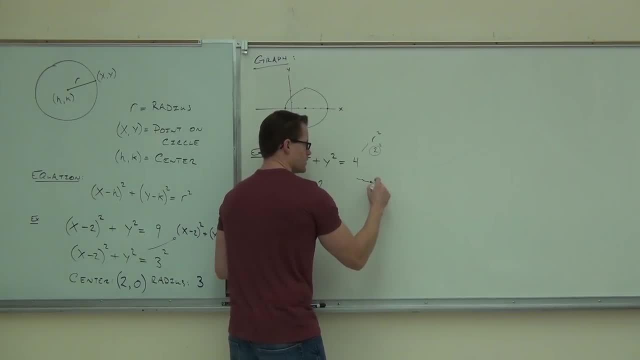 I could write this as x minus zero squared, sure. 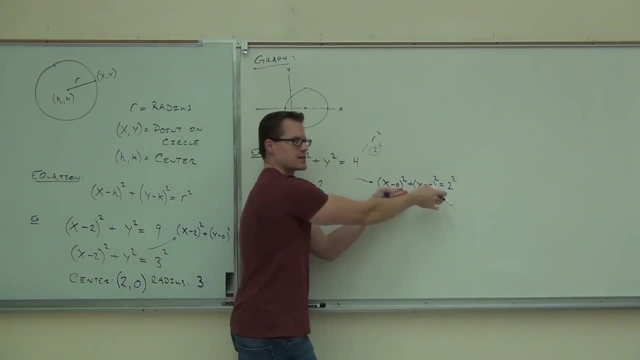 And y minus zero squared equals two squared. That's a different way I could write that exact same equation. 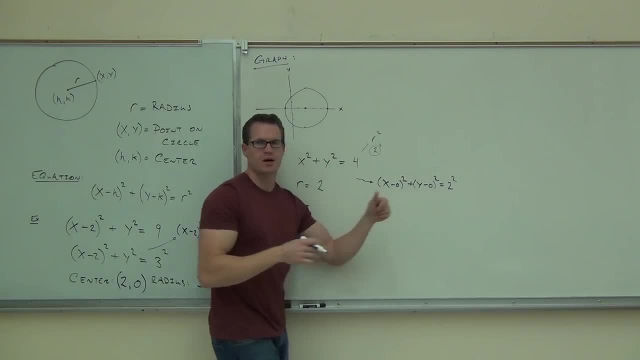 That's still four. This is still x squared. This is still y squared. I'm just subtracting zero from it. That means that my center is at zero, zero. Would you raise your hand if you feel okay with this example? 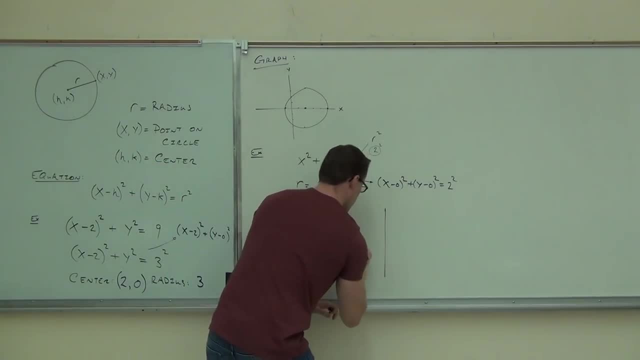 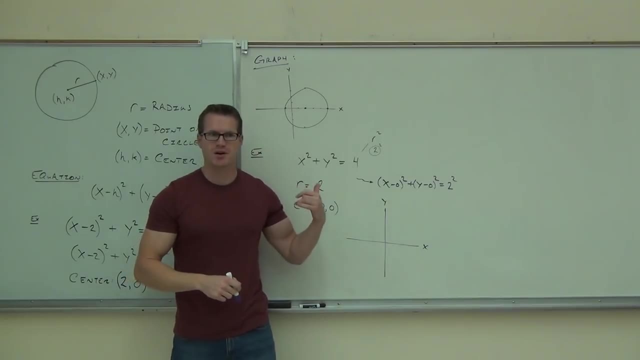 Well, now, let's try to graph it. I actually gave you the hard one before the easier one. It's weird, though. 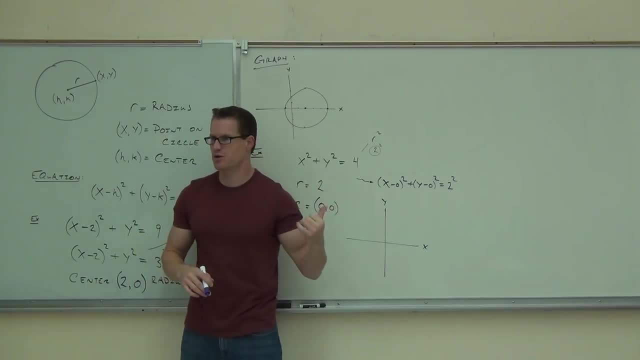 If I give you this one first, a lot of people are very confused on where the center is zero, zero is. But if I give you this one, they're like, oh, yeah, that makes sense. So, it's kind of strange how that works. 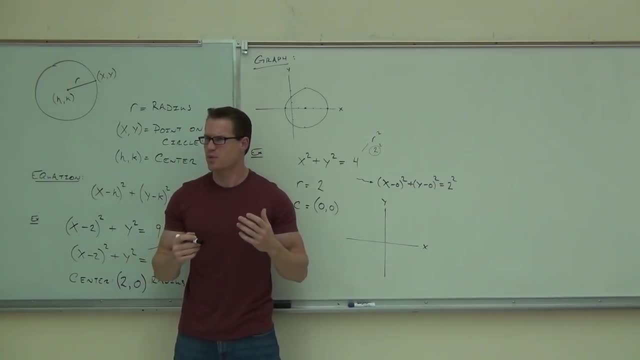 But if the center is zero, zero, then our center is at, what's that point called in the middle? Origin. Yeah, we're right at the origin. 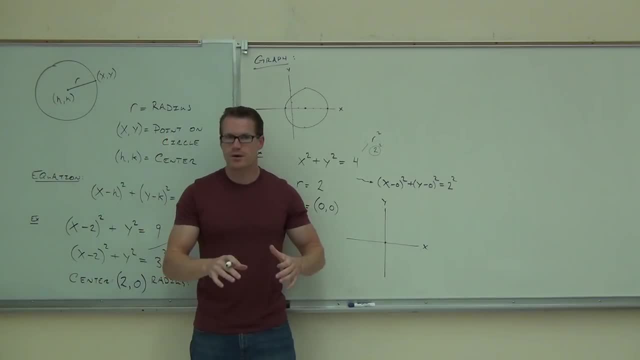 The center is at zero, zero. And the radius is, again, it's not four. It's not 16. How much is it? Two. 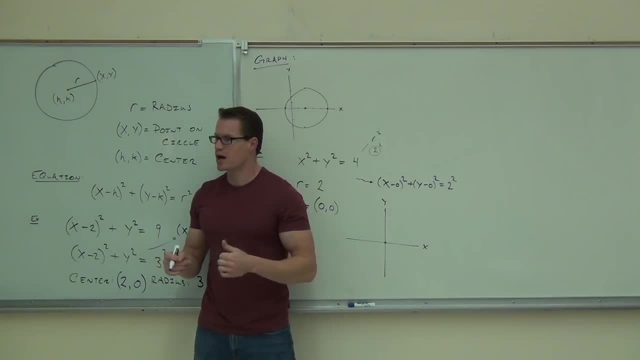 So, from the origin, I'm going to go two in every direction. Now, I'm from the origin at this one, not this one, because my center happens to be at the origin. So, I'm going to go up two, right two, down two, and left two. I'll make my circle around those points. I can't see his lines. I can't see his lines. 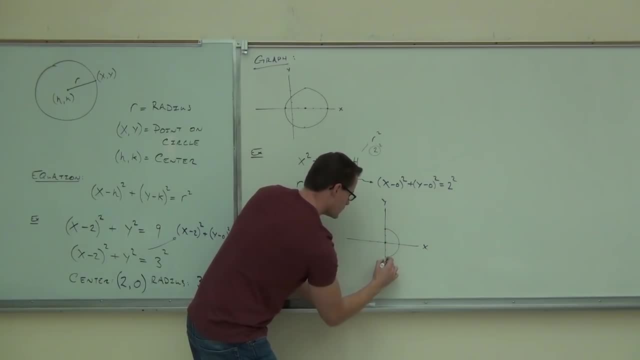 Oh, he didn't make one of the dots. I can't see his lines. 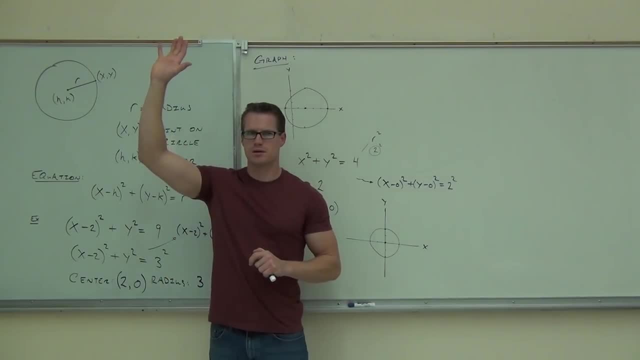 Okay, show of hands so far, how many people feel okay with what we're talking about up here? All right, let's do one more together. I'll give you one on your own, and then we'll talk about ellipses after that. 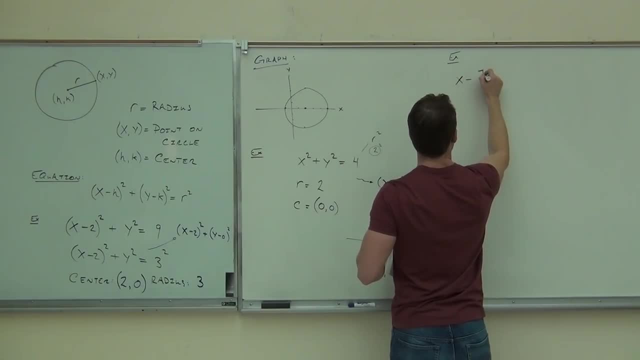 Don't make any fractions. There's nothing left. Yeah, just keep it simple. Oh, my God. How about that one? No, I'm just kidding. I'm just kidding. I'm about to have a heart attack. Fractions? 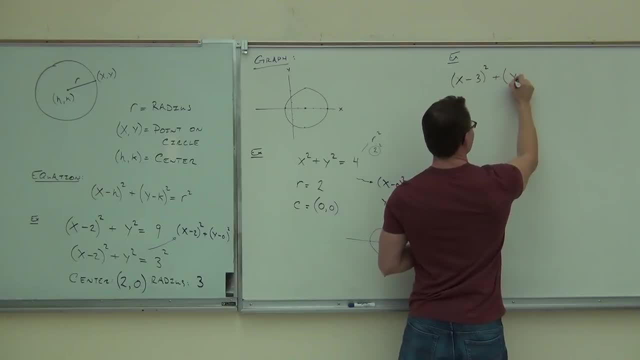 Like we haven't been dealing with them for this entire semester. They're ugly. They're ugly. 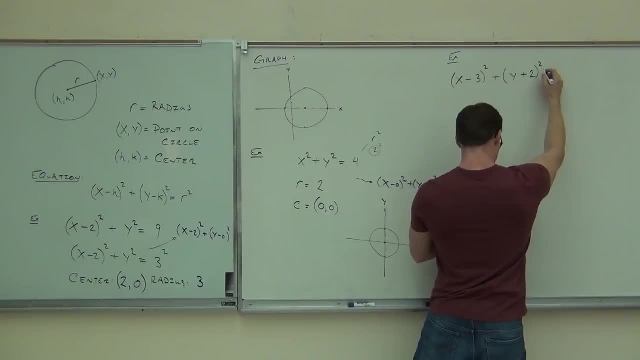 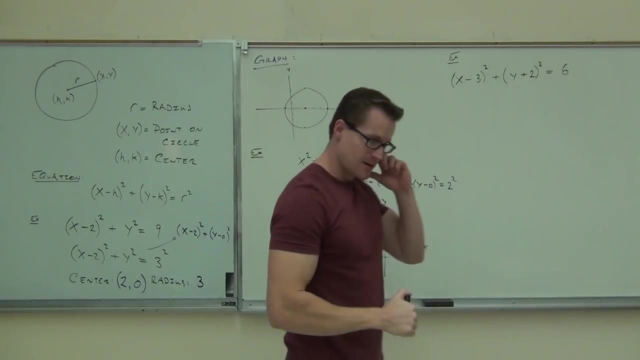 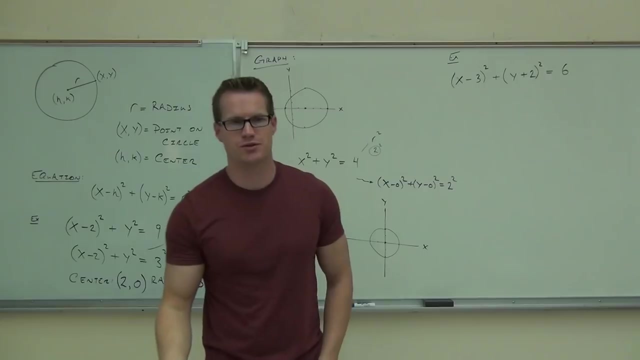 Okay, again, it's up to us to find the center and the, that's only two things you need to know about a circle. 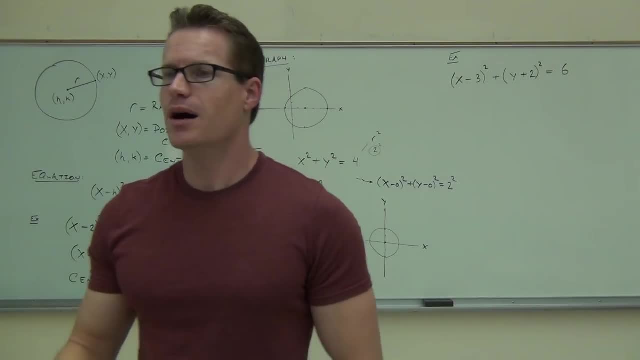 That's it, besides the fact that it is, in fact, well, a circle. So let's identify, first, it is a circle. 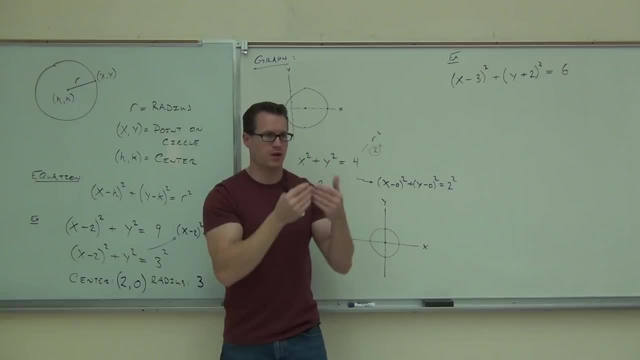 Do you have an x squared, a y squared, and a plus between them? Yes. Yes, all right. Great. So we have that down. 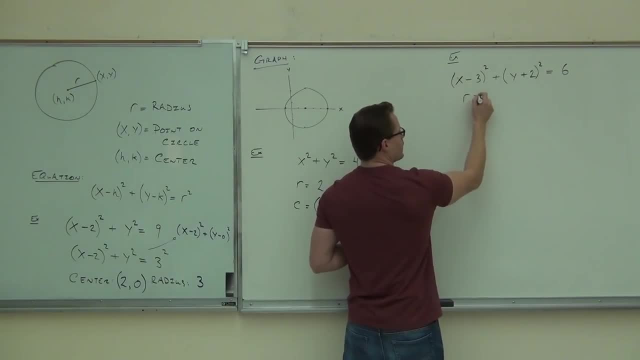 Next thing, well, let's look at our radius. But before that, on this particular one, I will look at our center first. 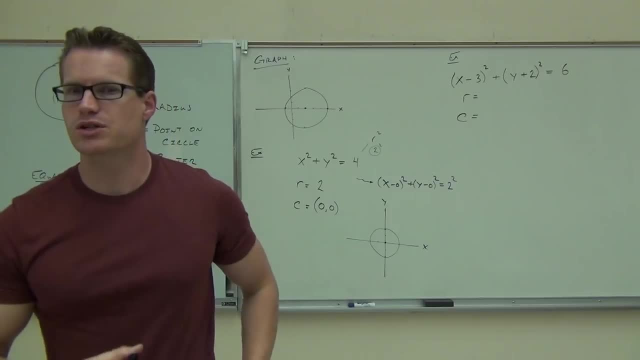 Our center at this point should be pretty easy to find. So let's go ahead and do that. I want you to write down what you think the center is right now. Think about what we've talked about so far and write down the center. Don't say it out loud. I don't want anyone to do this. This is up to you. 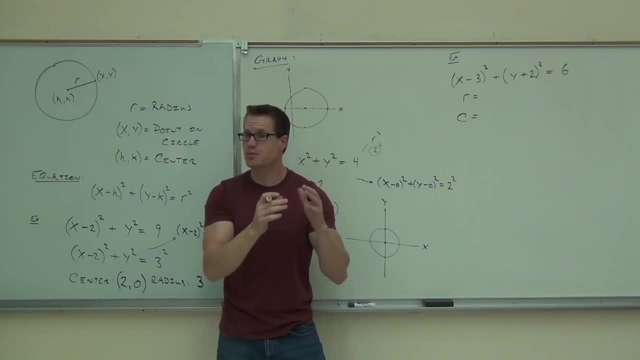 The center is always going to be a point, right, because we've got to put a point on our graph. It's not just going to be one number. 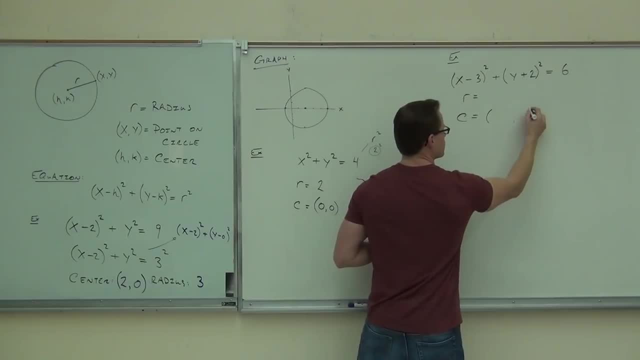 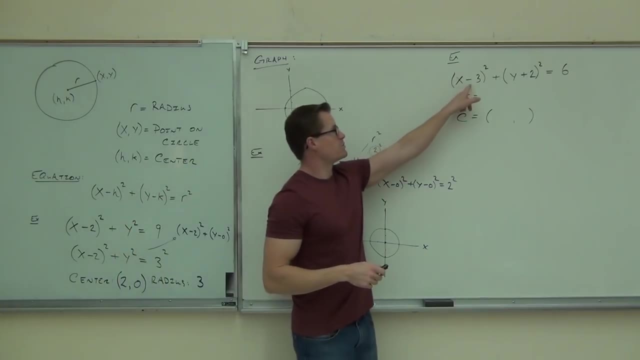 It's based on the x and the y coordinate. So our center should be something comma something. If you think about it, this right here, this minus 3, that minus 3, since it's associated 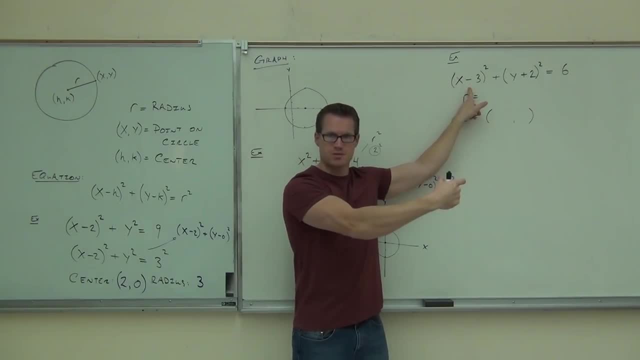 with our x coordinate, means a shift to the right three spots. Does that make sense? 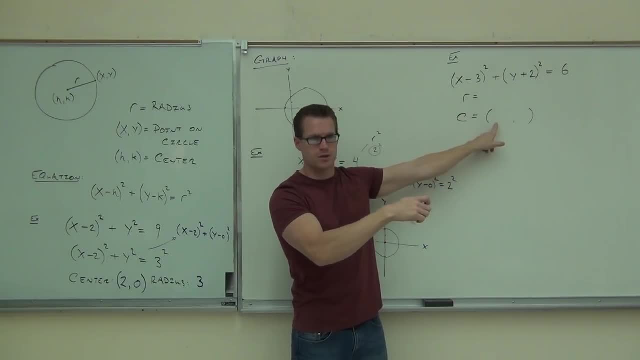 That means that we're going to have plus 3 or minus 3 here? Positive 3. Positive 3. Yeah, absolutely. 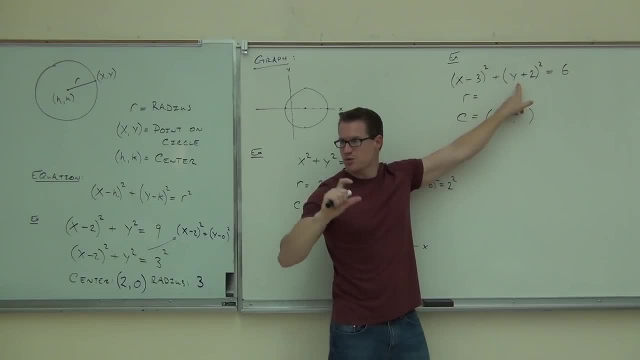 Now this y, that y, since it's associated with y, it's going to be either up or down. Plus means down. Minus 3. Positive 3. Positive 3. Minus means up. 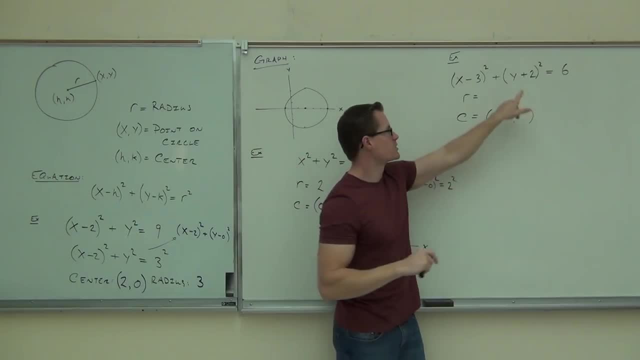 It's in those parentheses, so it's back to what we want to think it is in our heads. So is this going to be a minus 2 or a plus 2? Minus 2. 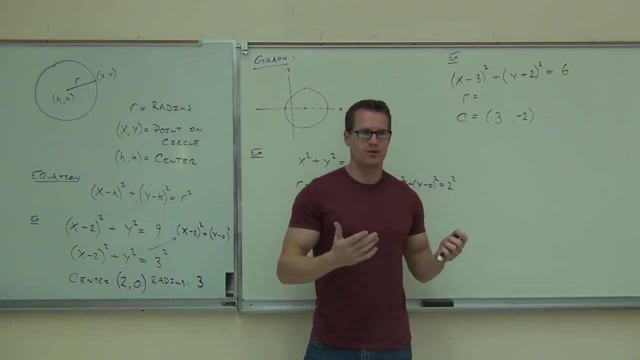 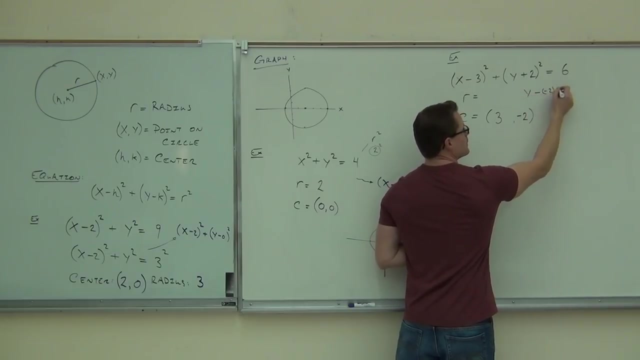 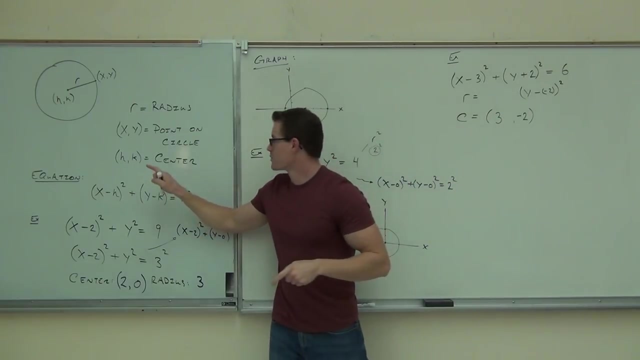 By the way, for some of you mathy guys who want to, or mathy gals who want to think, well, wait a second. This is minus, well, why is this plus, why does that plus mean down? If you write this as the formula, you could write it y minus negative 2 squared. Isn't y minus negative 2 the same thing as y plus 2? Now it fits in our formula right there. Y minus k. Y minus k is negative 2. That's how we're getting our center there. Do you guys see it in the formula as well? All right. 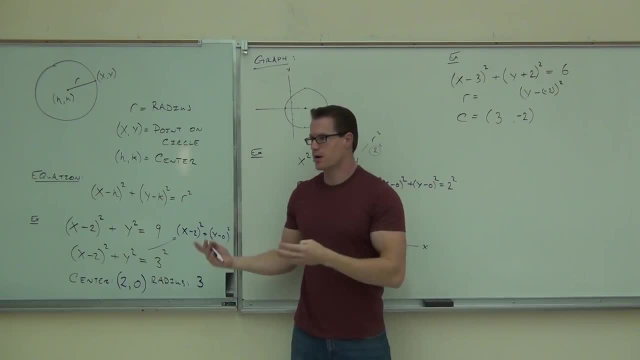 So it now makes sense shifting-wise. It now makes sense formula-wise. You have two ways of looking at it, whatever way you guys prefer. In either case, I need to be able to get the center of 3, negative 2. How many people were able to find that? 3, negative 2. Okay, good. Whoa. Whoa. Now, radius is, of course, 6, right? Radius is 2? 3? What's the radius? How do you find the radius? Oh, no. 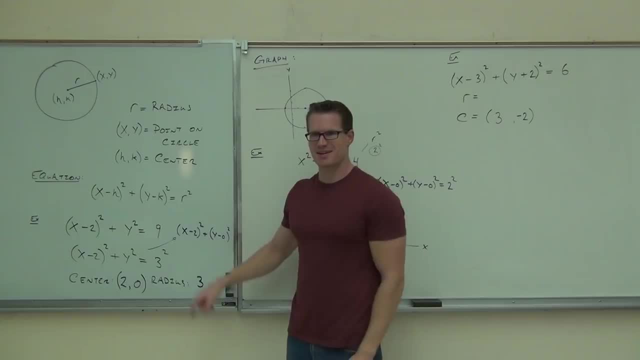 The radius here was the square root of 9, right? Which you were all like, yeah, 3, got that. The radius here was, well, 2, because you're like, 4 squared of 4, that's 2. That's easy. Well, how do you do 6? 36? Is it 36? No. No, because then this would be radius of 81. That doesn't make sense. 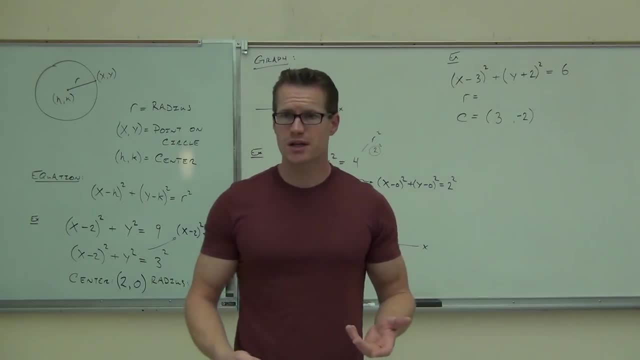 We're actually taking square roots of things, right? Well, can you take the square root of 6? Yeah. 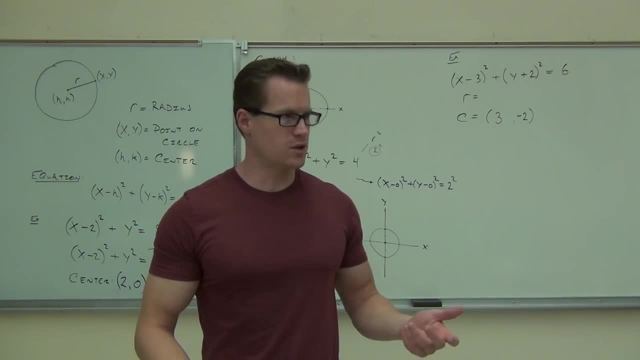 Of course you can. Is it a whole number? No. Well, no. But you can still do it, right? No. 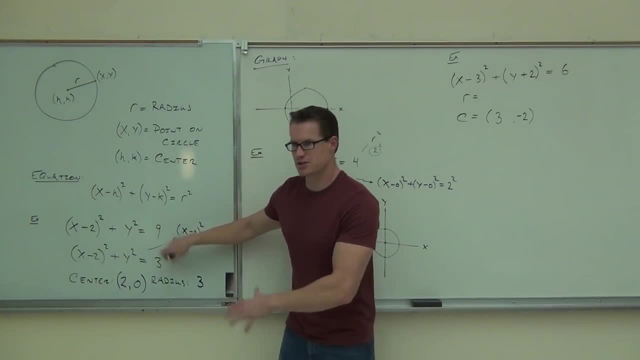 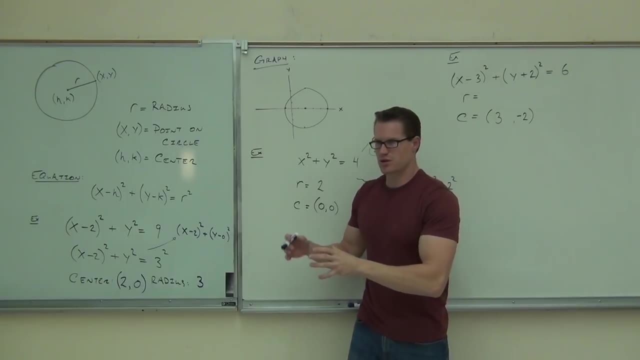 So, if our number here, our constant is 9, our radius is 3. If our constant is 4, our radius is 2. If our constant is 6, it's not a pattern, it's a rule. 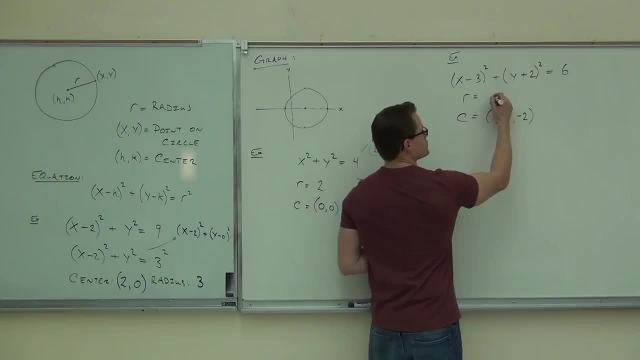 We're taking a square root, we're taking a square root. So, our radius here is the square root of 6. It's a root of 6. It's a square root of 6. Why? It's not 6 squared, right? It's not 36. Why? Well, look at it. Look at the board here real quick. 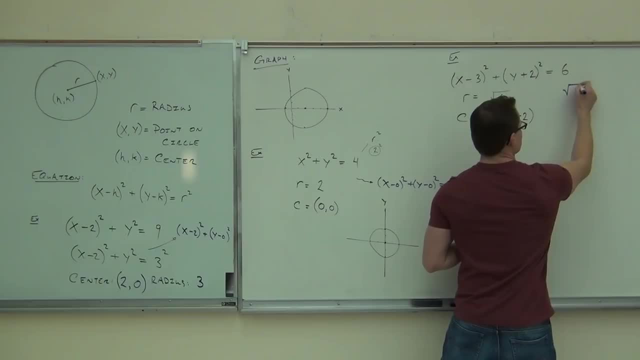 Couldn't you write this as square root of 6 squared? Is that still 6? 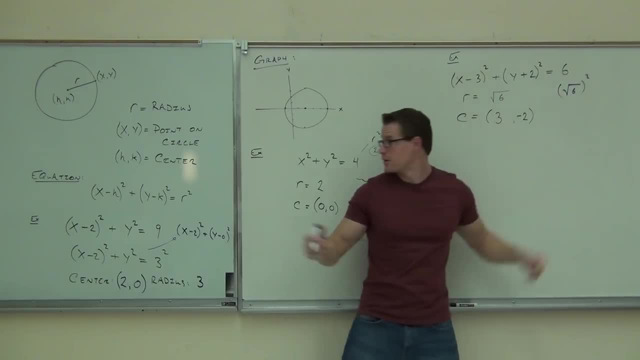 Well, now this fits in our formula. This is the radius squared, just like that. That's the radius squared. So, our radius is actually the square root of 6. 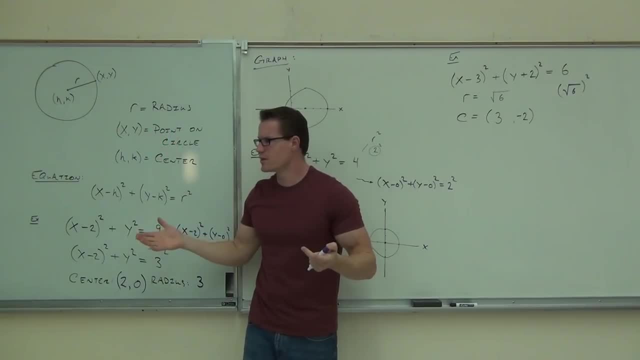 Would you raise your hand if you feel okay with that one? That's a little weird, right? We don't get a whole number. Could you still graph the square root of 6? Take your calculator out, find out about how much the square root of 6 is. 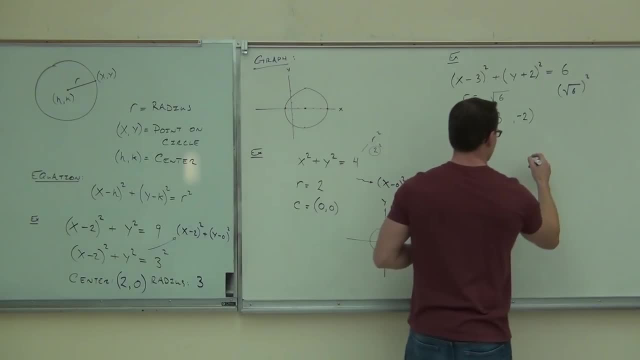 2.449, so about, like, 2 1⁄2, around there. You said 2.498, right? Exactly. 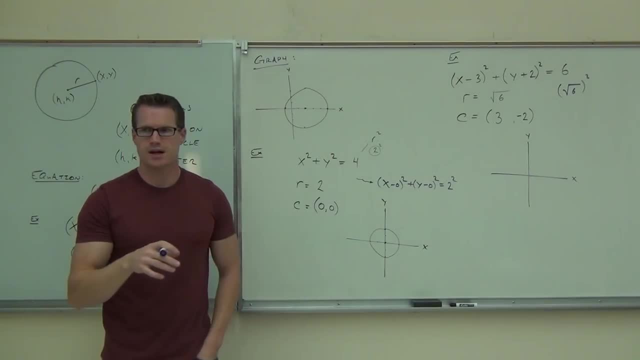 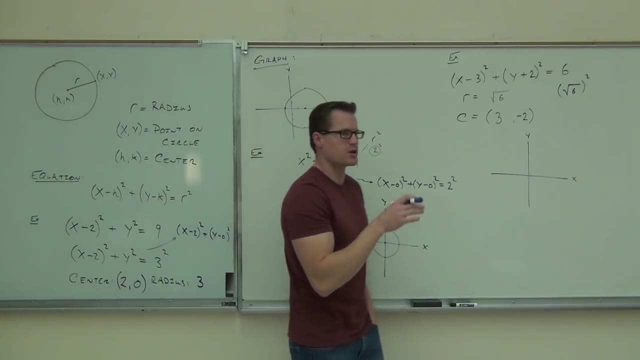 Okay. So, if our radius is the square root of 6, we find out about 2.4, just under 2, 2 1⁄2. So, we'll go ahead. We'll plot this. You make your center first, and then approximate your radius. 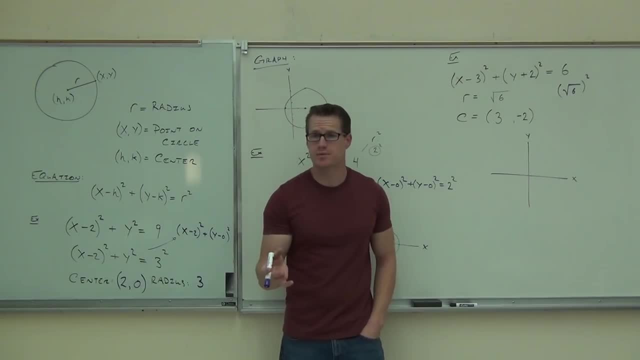 Now, you're not going to be exact, because you can't be exact with the square root of 6, but you can approximate it. 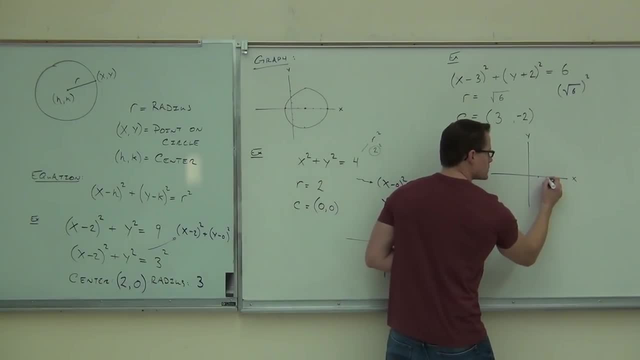 So, if we're center 3, negative 2, 3, negative 2 is 1, 2, 3, down 2. Hey, just like our shifting would work. Look at that. Isn't this kind of neat? I hope it's neat for you. 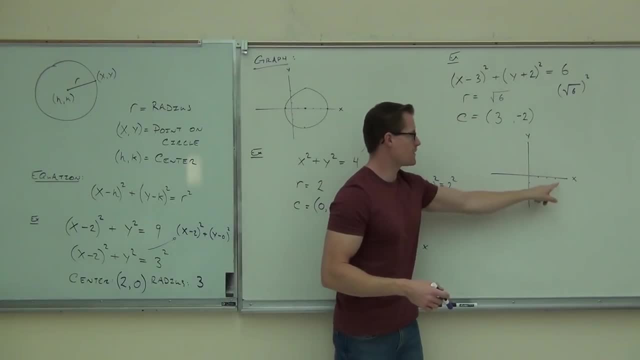 You can shift this to the right 3 and down 2, and that's exactly where your center is going to be, exactly what we thought it was going to be. Are you with me on that? 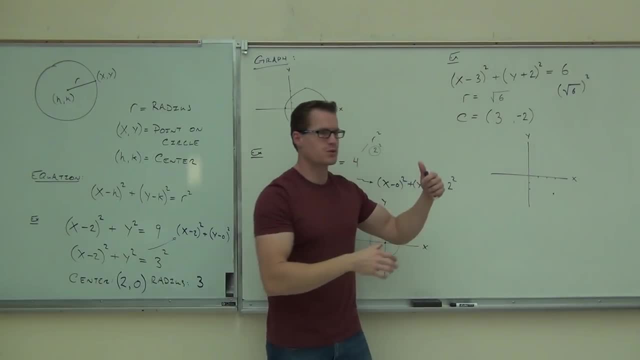 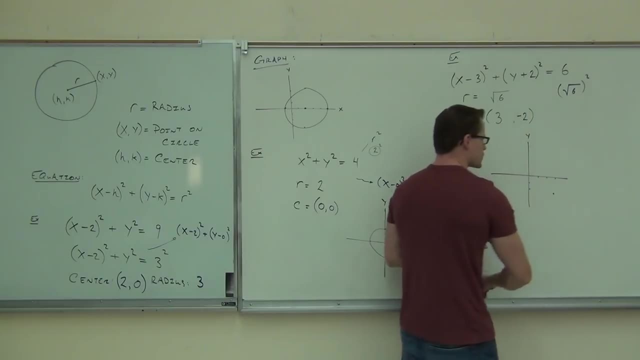 From there, we've got to go up 2 1⁄2, about 2 1⁄2, down 2 1⁄2, left 2 1⁄2, and right 2 1⁄2, or 2.4. So, a quick question. Are we going up, down, left, and right from our origin? 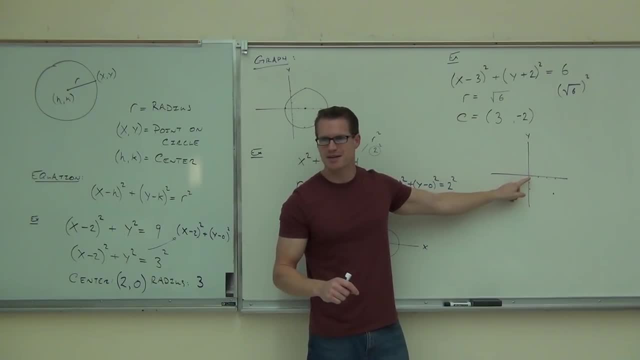 No. No, because then every circle would be centered at the origin. That's not the way it is. Our center can move around. 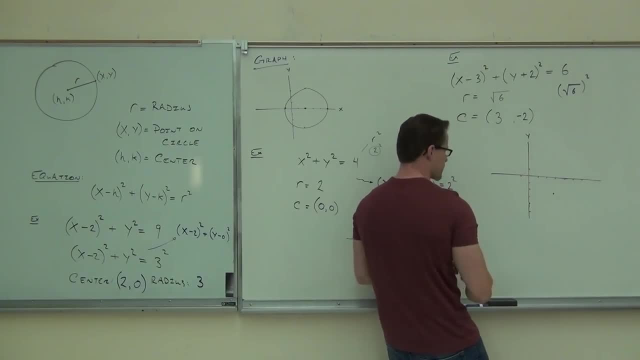 Okay, so I'm going to go up 2 1⁄2, 1, 2, and a half, just about 2 1⁄2. 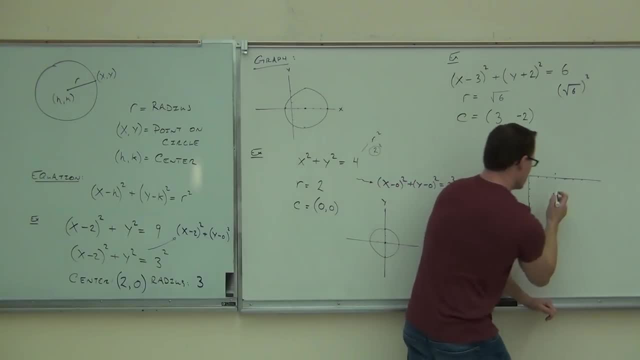 I mean, it's 2.4, but on a graph, you're not going to be able to tell the difference, really, unless you do a really precise graph. 1, 2, and a half. I'm doing pretty good. I'm on it today. 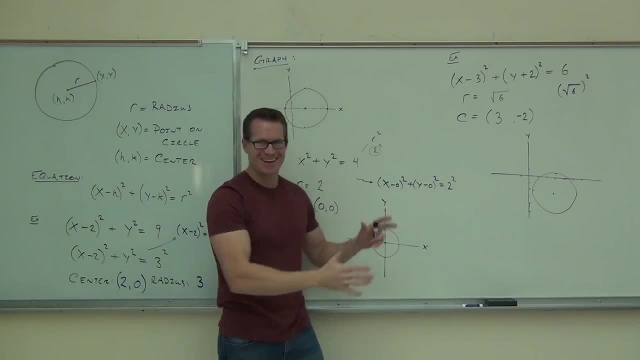 Take a picture. Oh, I have a picture of this. These are the best circles I've ever done. I'm really, feel good about that one. 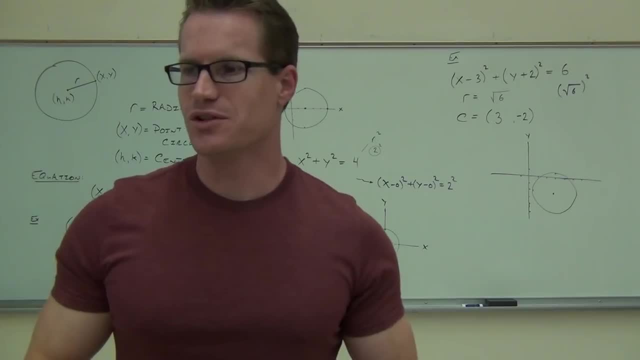 Do you feel okay on how to draw your circle, well, not draw circles, because I know some of your circles suck out there, but do you feel okay with finding your center and your radius? 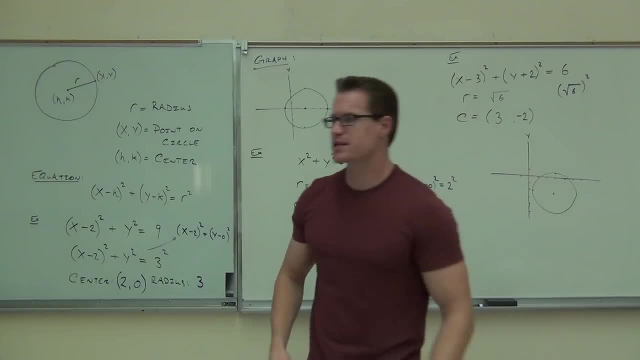 That's the big thing, is finding the center and the radius. Let me go ahead and give you one example to do on your own. And we'll move on to a shape called, ellipse. Ellipse. Ellipse. 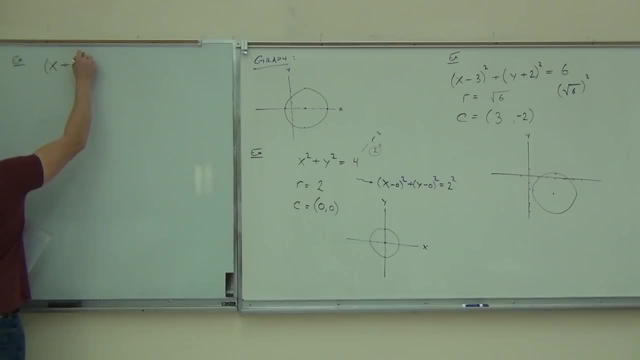 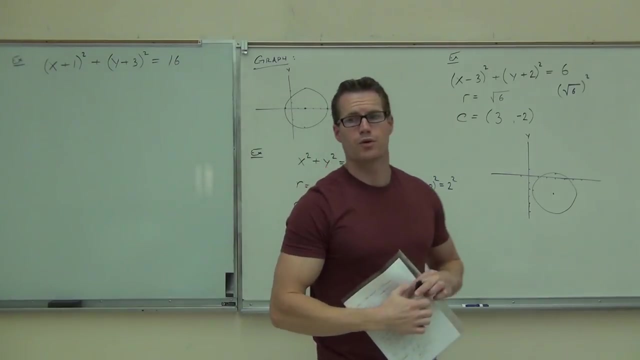 It's like a football. Okay, go forward. Do this on your own. I want you to find the center and the radius. It doesn't matter the order in which you do that, but when you draw your circle, you've got to do the center first. So. . . 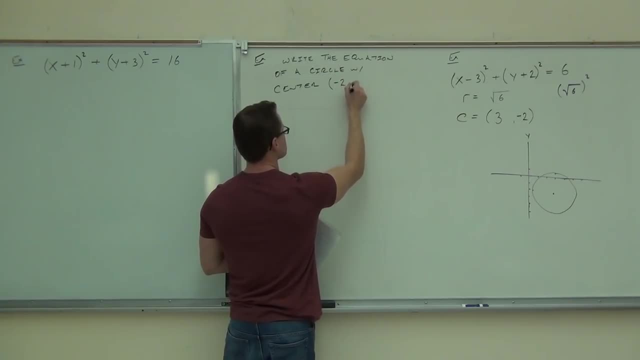 . . . . . . . . . Thank you. 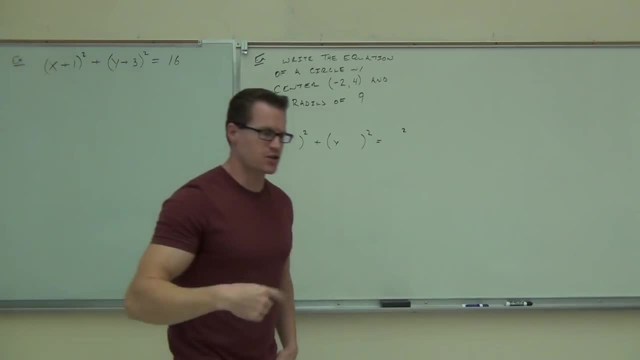 Once you get the hang of these circles, they can go pretty quickly. We're able to find the center and the radius here. 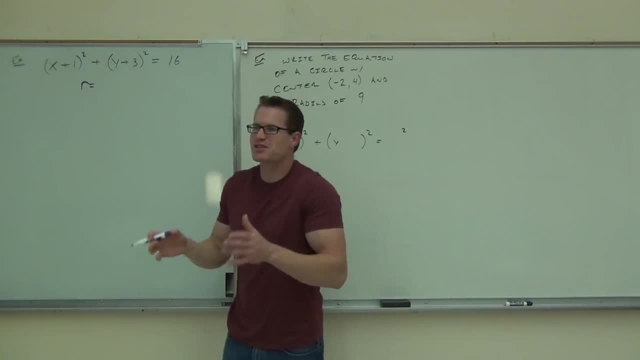 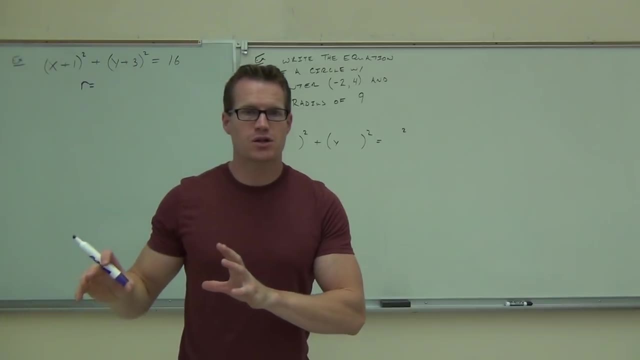 Is the radius nice in this one? Radius isn't like the last one where we had the square root of 6. Here we're taking the square root of whatever constant number is off to the right-hand side. So in this case it's 16. So for 16, are we going to get 16 radius of 4 or radius of 16 squared? Which one? 4. 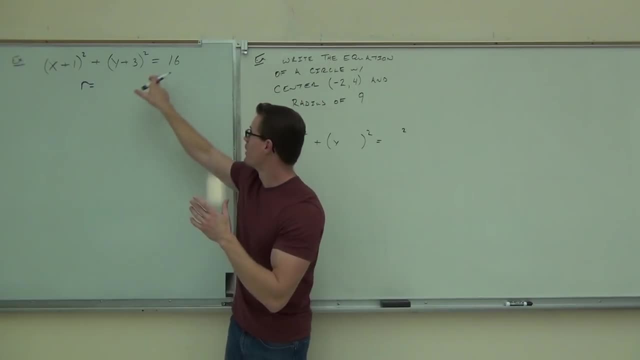 4, because whatever that number is, we're taking the square root because we know that this number is actually the radius after it's been squared. You follow me? How many will we be able to get 4? 4? 4. 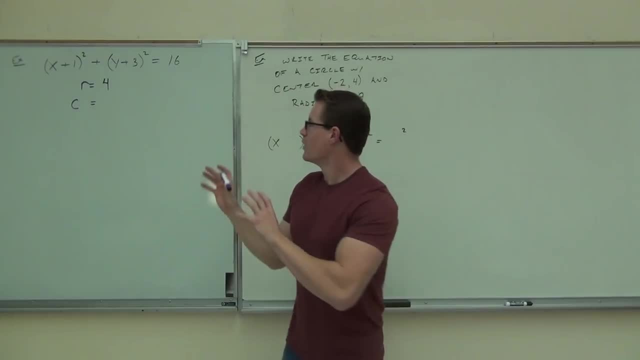 Now the center, the center you've got to be rock-solid in the center. So you've got to know where the x-coordinate is coming from, associated with the x, where the y-coordinate is coming from, and get the correct directions out of this. 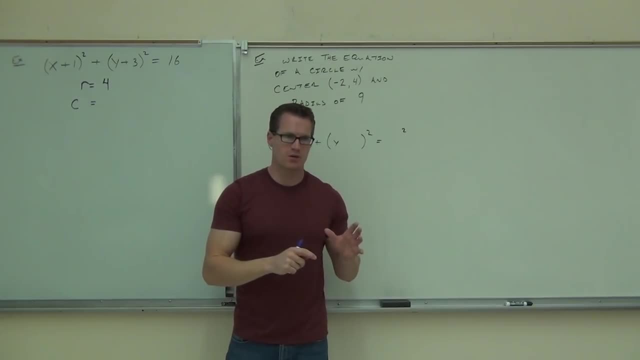 Now we know from our parabola days, from all the work we did shifting graphs around, that whenever we have a number inside a parenthesis, typically it's opposite of what we want to think it is. It's a shift in a different direction. So in our case right here, that plus 1 is associated with x. That means we're going to be going to the left 1. This plus 3 is associated with the y. That means we're going to be going down 3 spots. So on your center, you should have negative 1, negative 3. Do you have that? 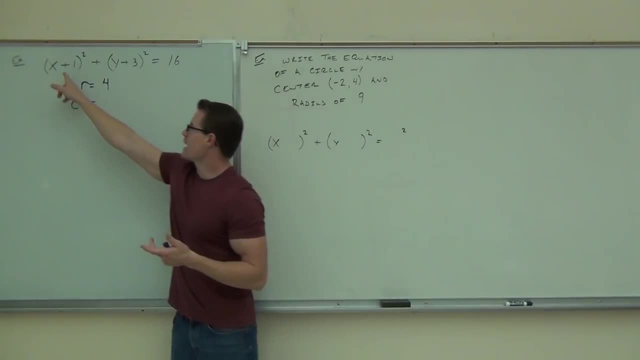 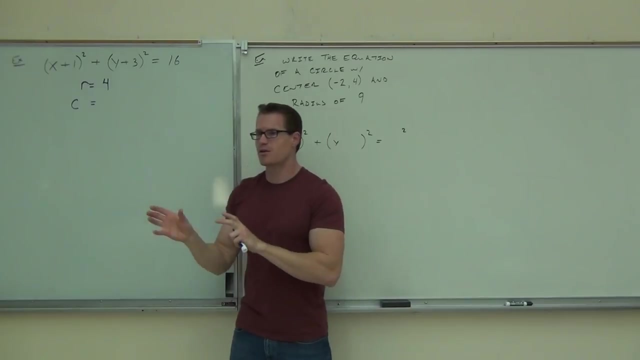 According to the formula, you can look at it that way also. This could be x. Minus negative 1, y minus negative 3. Minus and negative, that's where they're getting that plus. So again, by the formula, you should be getting here a center of negative 1, negative 3. 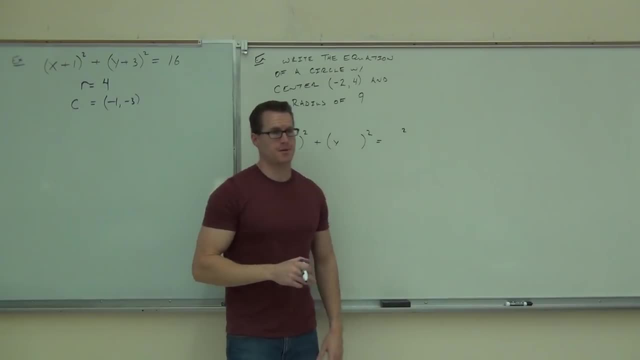 Not sure if you got both those things right. Okay, with that, you should be able to graph it. 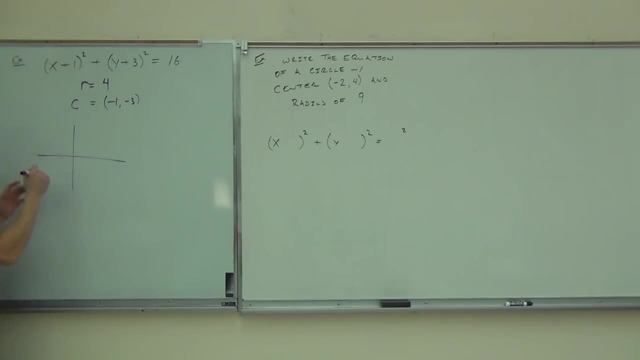 So after we find our center, we're going to put that on the graph. 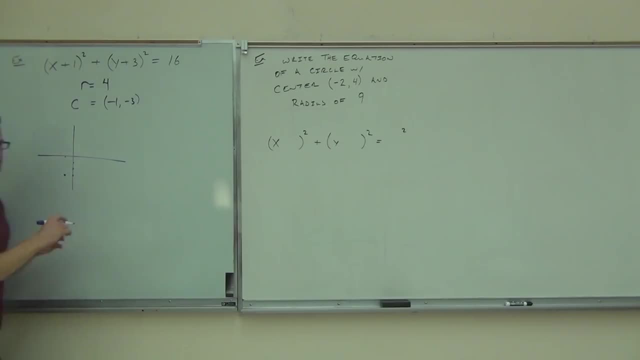 Negative 1, negative 3 is just a point right there. That says your set of points is going to be circled or centered around that specific spot. From there, we're going to go forward in every direction we can. Now, on graphs, that means up forward, down forward, left forward, and right forward. 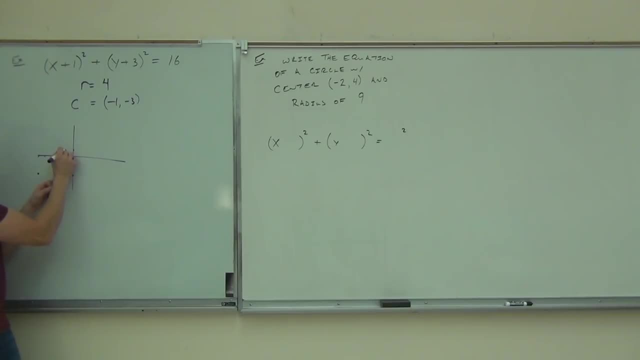 So that's here. That's up forward, down forward, and right forward. Okay. 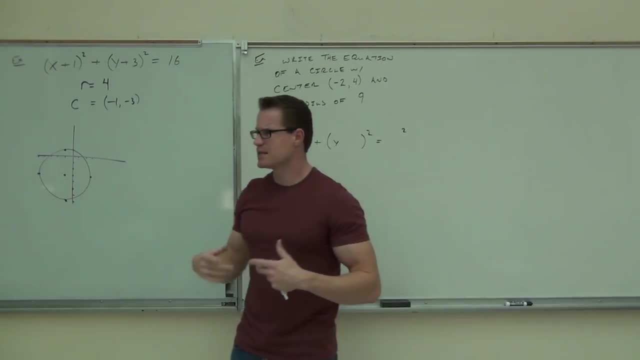 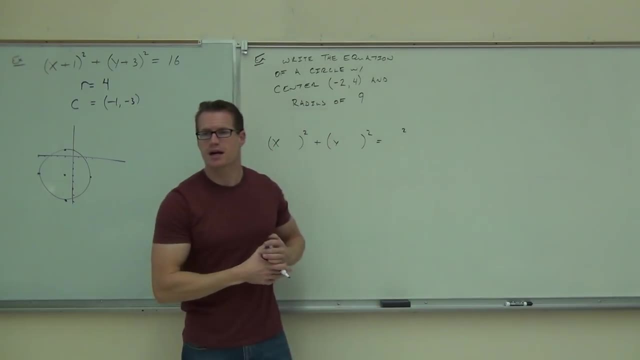 Which way should we have to get a circle about like that? Do you feel okay with the idea of these circles? One last thing we can do, can you go backwards? For instance, if I don't give you the equation, I say find the equation if I give you the center and I give you the radius. Can you do that? Yes. 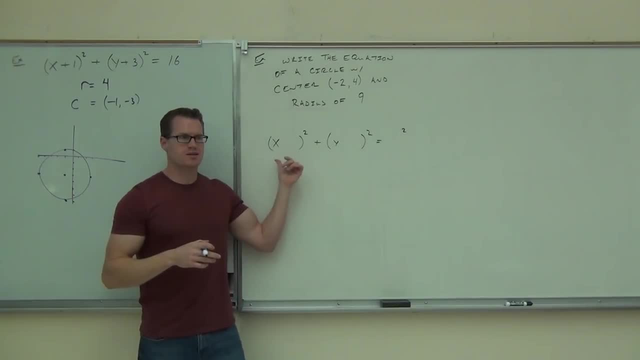 Notice how the equation for a circle is always this thing. It's always x squared, y squared, and then a radius squared. You just have to fit these numbers in appropriately. 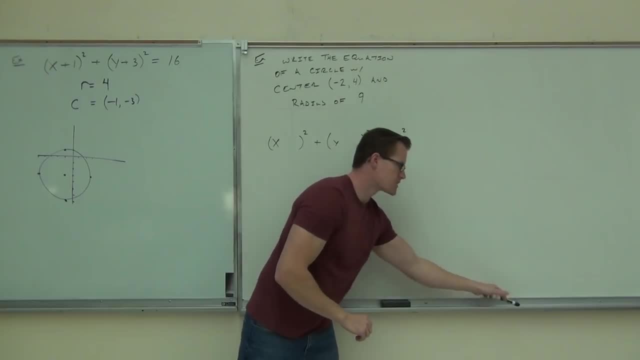 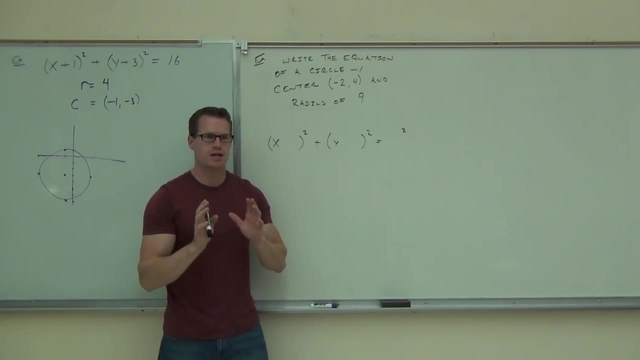 So can you tell me if I'm centered at negative 2, 4, negative 2, 4, you're either going to plug in 2 or negative 2. Where's the 2 or negative 2 going to go? With the y or with the x? The x. Yeah, x's go with x's. Y's go with y's. 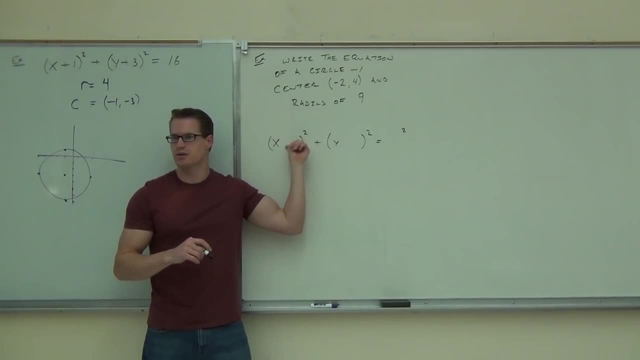 The question is are you going to have a plus 2 or a minus 2 here? Plus 2. Plus 2. Why plus 2? 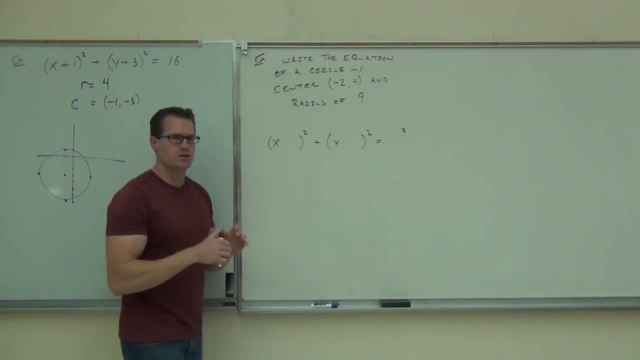 Yeah. Hey, you know what? This is going to be kind of equally awesome. If you were to plug this into the formula, the way it is, notice how we're supposed to have x minus h squared 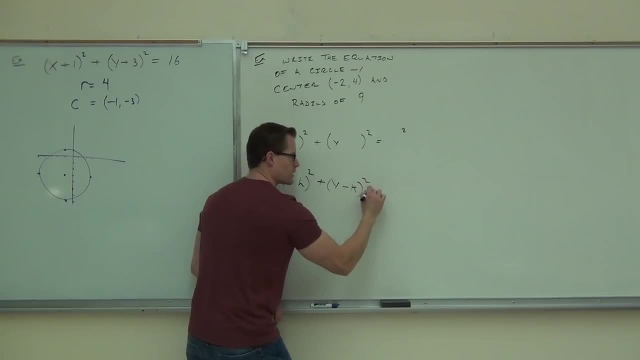 plus y minus k squared equals r squared. 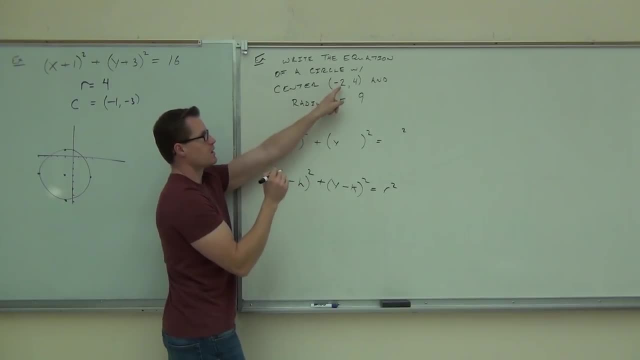 If you plug in minus h, that's your h. What's it do when you have a minus and negative? It changes to that plus. That's where we're getting that from. 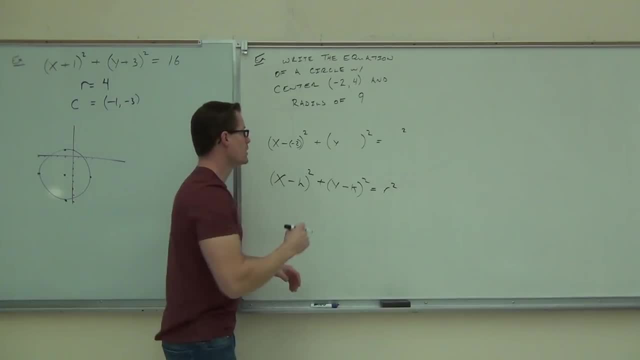 That's why we were able to understand this center from the formula. So yeah, we're going to get x plus 2 there. 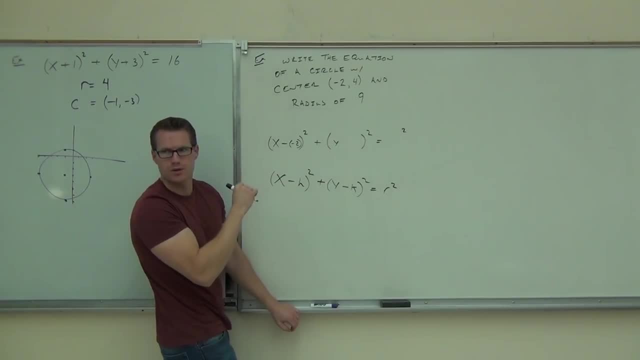 What are we going to get over here? y plus 2 or y minus 4? What do you think? Again, you plug in minus, y minus k, k in that case is 4. 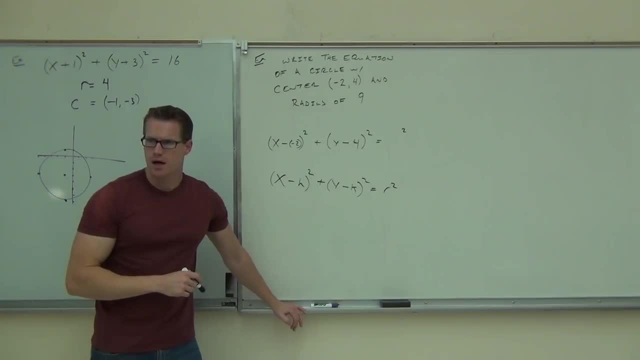 What about our radius? Nine. Nine. So is it just, is it just, are we going to leave it just 9 down there? Are we going to put 3? What are we going to get out of our? 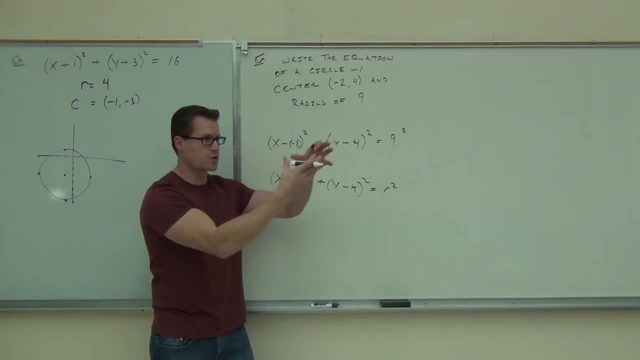 81. 81. You're going to square that radius. Just like you would take a square root of that constant to get your radius, you're going to square the radius to get that constant. So in my case, r. 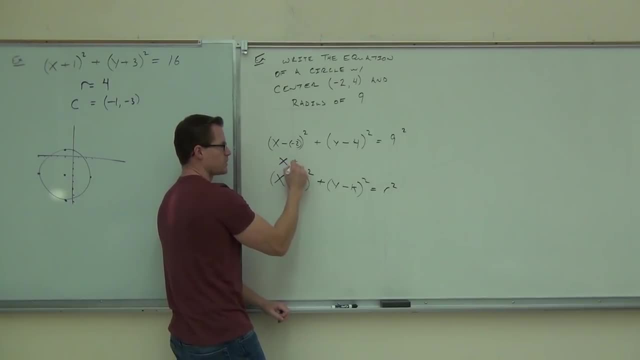 The formula for our circle is x plus 2, y minus 4, both being squared, equals 81. 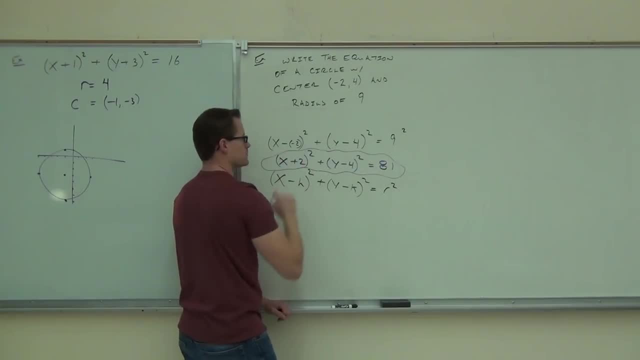 How many of you feel okay with that so far? Would you like to try one of your own? Sure. Okay, same question. I'm going to give you just your center and your radius. And just make sure that you're in the right place. 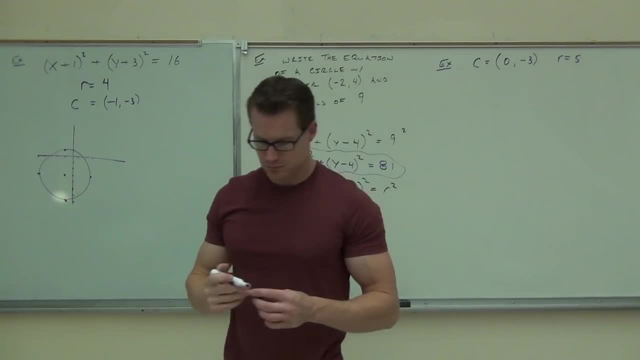 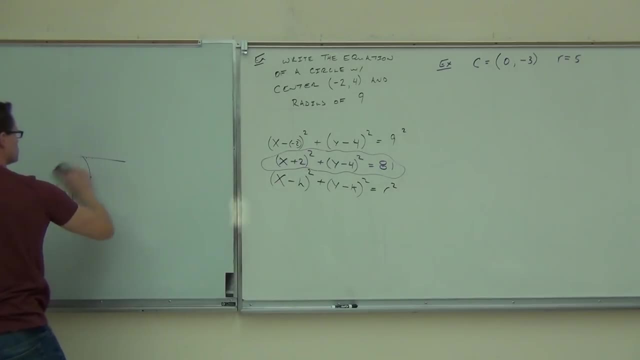 So just make sense? And just make the acept IQ as, Yeah. 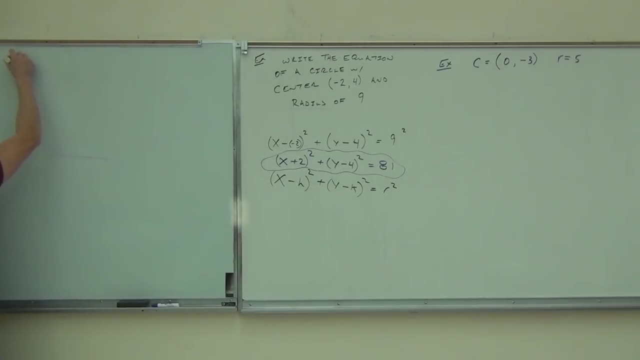 All right? So if you can explain that before we get to question 우리는? We can. Thanks. I'll see you soon. Bye bye. So stay tuned until next week. Okay. 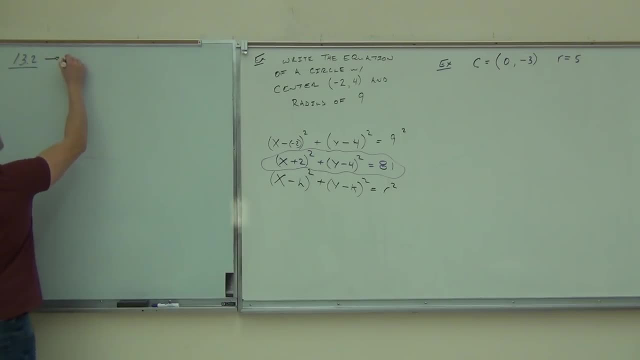 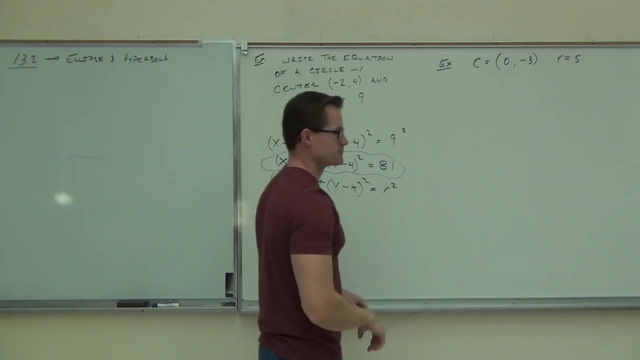 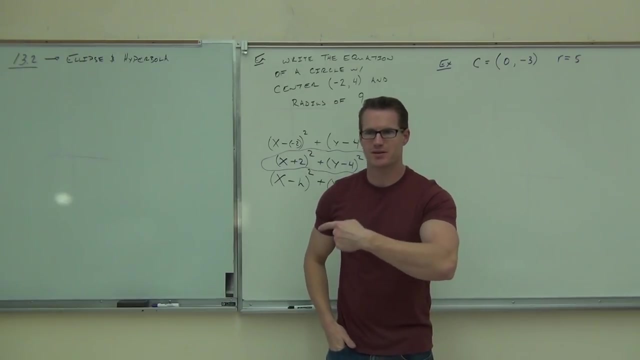 It's even quicker than the actual graphing part, right? You just plug these into the formula, basically. 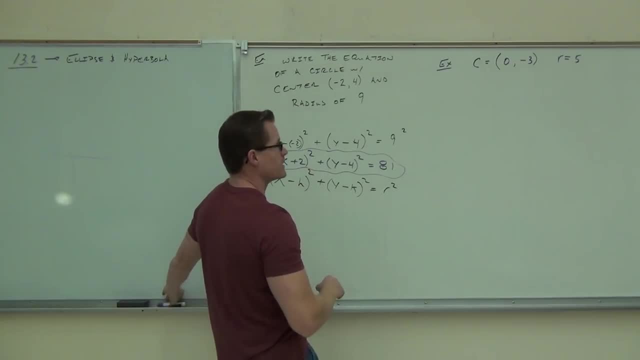 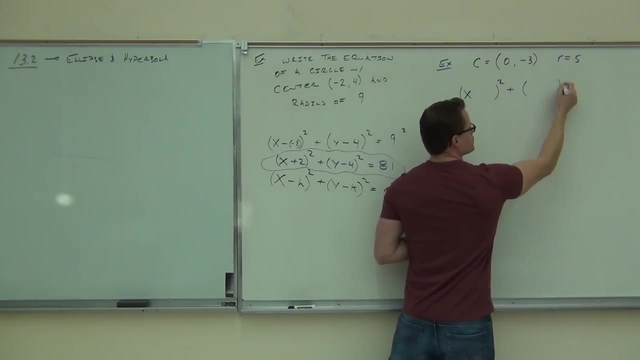 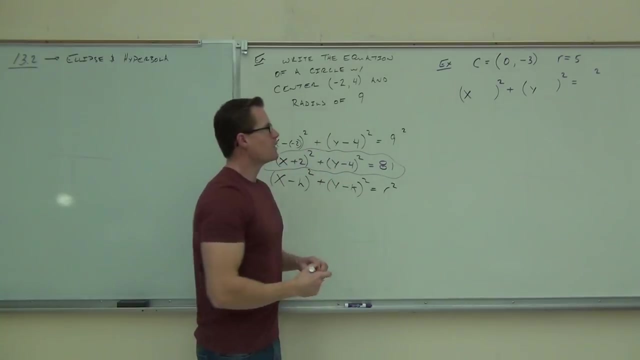 So if I'm asking you for the equation of a circle, and I've got my center and my radius, my equation is going to be x minus something or x plus something squared and y plus or minus something squared equals r squared, whatever that happens to be. 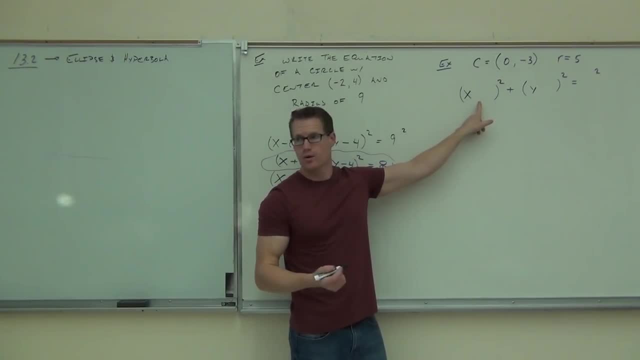 What am I going to be adding or subtracting to my x here? Zero. Oh, okay. So it really doesn't matter what you put because you're adding or subtracting zero. 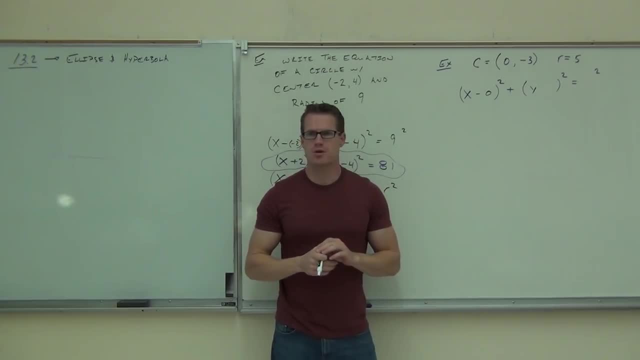 Just make sure you have a zero up there. How about with the y? Am I going to be adding three or subtracting three? Adding three. 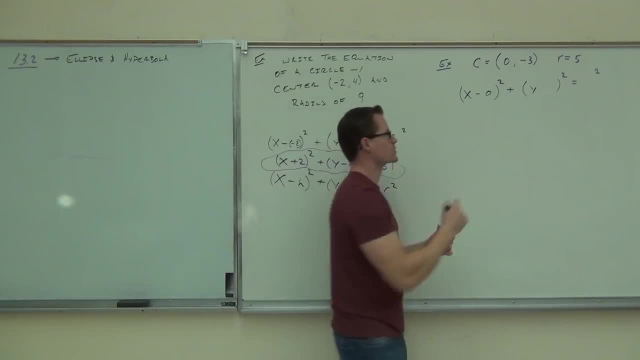 Adding three because you're subtracting a negative. That's how the formula works. 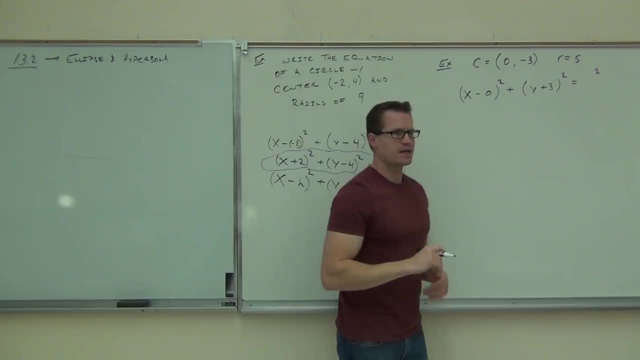 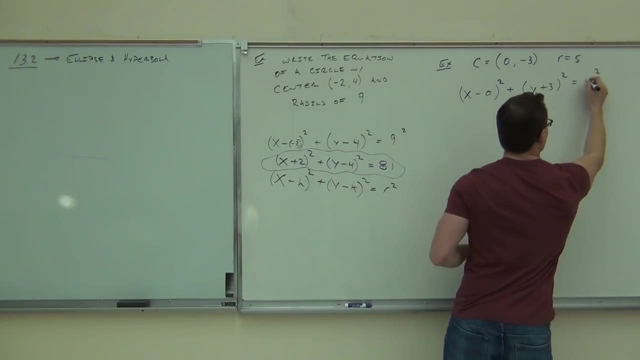 So we would be adding three and the radius that we're going to have, what is that? So am I going to end with five or end with 25 or something different? 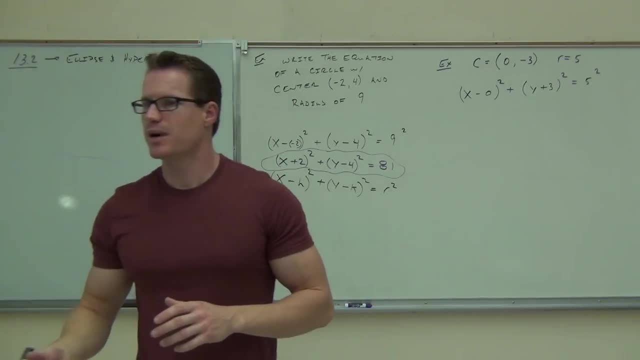 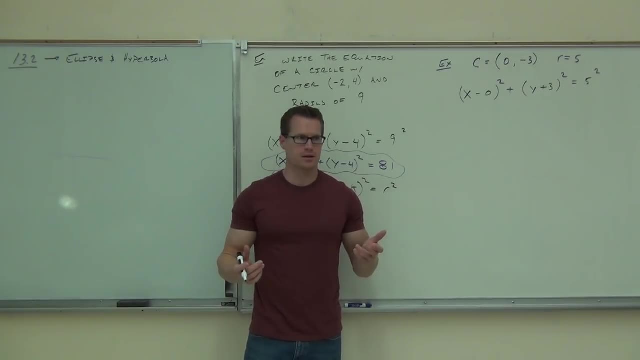 So plug that into the formula first and then simplify what you can. X minus zero, how much is x minus zero? X minus zero is x and then we square it. So this whole thing, don't leave it as x minus zero. 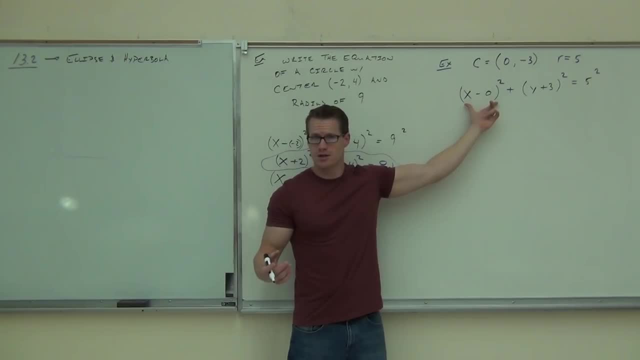 Write it a little bit more better, write it simpler than that. 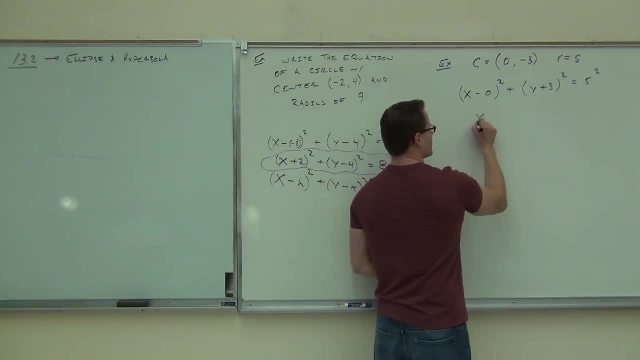 So x minus zero, that's x. If we square it, we're going to get x squared. You okay that that is actually x squared? 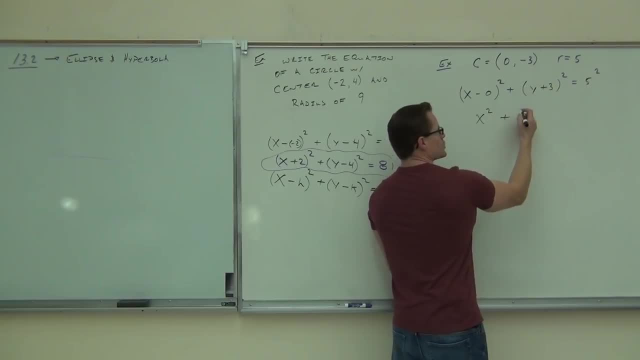 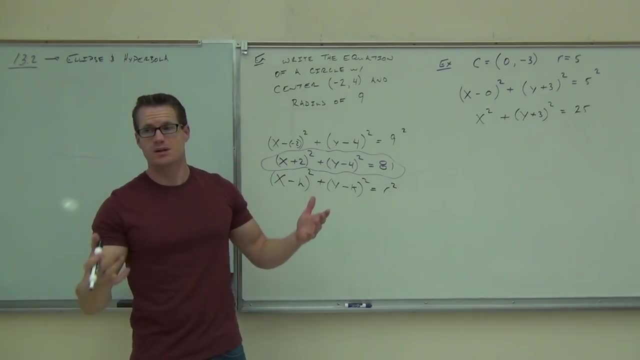